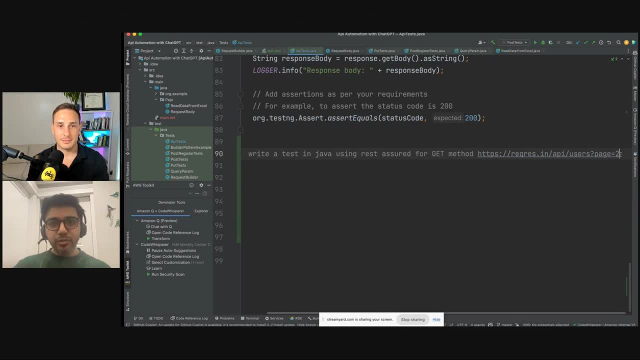 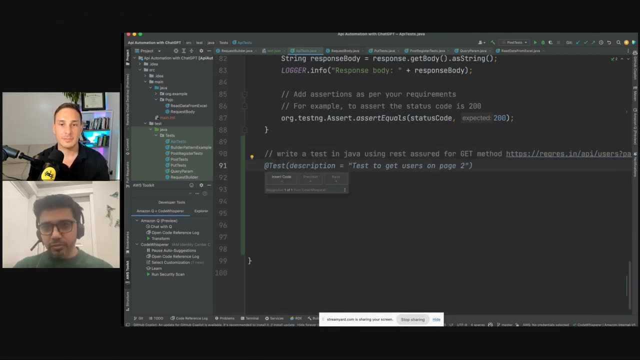 let's give it a try- that how we can write a automation script using rest assured and Java for get method And for demo purposes. I'm using this endpoint. Okay, this is an open source endpoint. you folks can also use it. There is no harm in it. So this is the prompt. I have given the try to test in Java using rest assured. 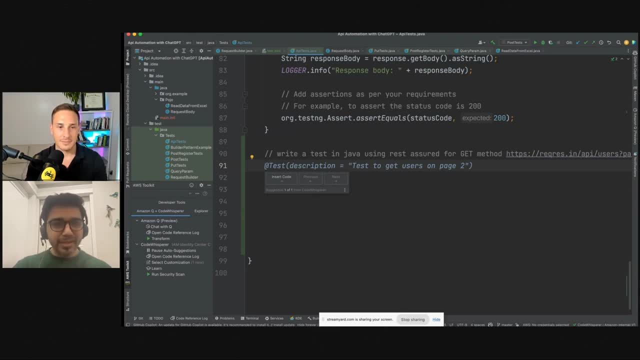 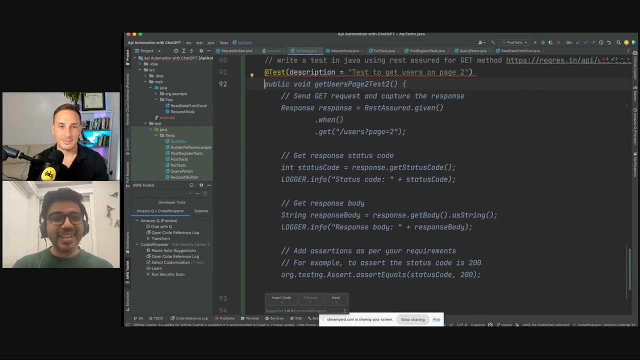 for get method right. So, if you have noticed, it has already prompted me at the right test description. So see, AI is pretty smart, right? It is using description, which we folks miss a lot. Okay, so I haven't pressed enter again. And after you press enter, see, So I guess it doesn't take. 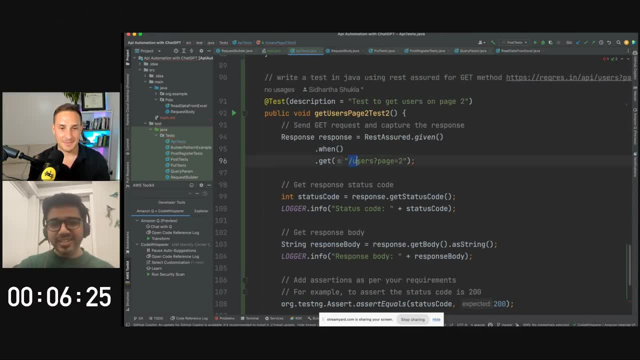 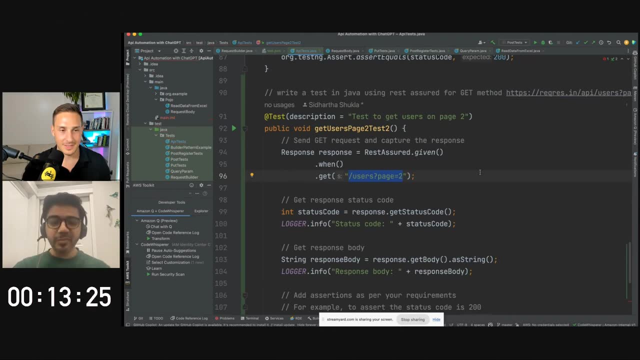 even 60 seconds. it has completed writing the code in just two or three seconds. Let me run the test to see if it works. Couple of changes we need to do for sure Right. For example, here it has used slash users to 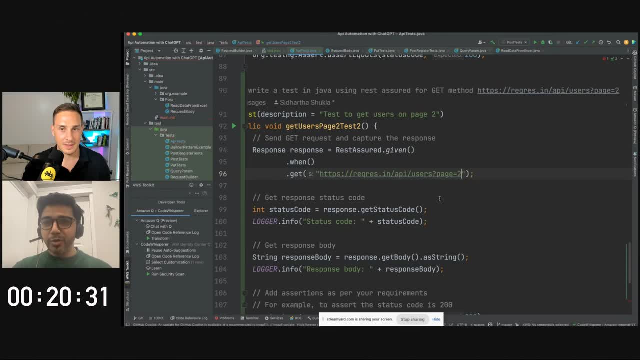 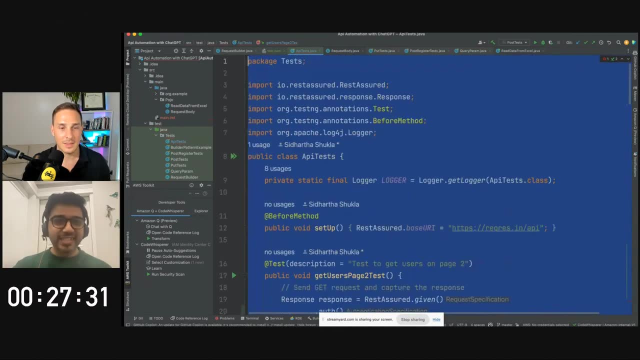 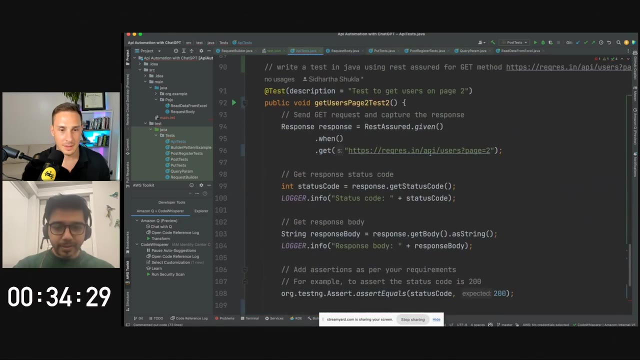 write, but it may not work with that. What I'm going to do? I'm going to change this one Right. That's why they told right over: dependence on AI is not good. So those small changes definitely we need to do correct And I will prefer to comment all the previous code: See the before method. it has. 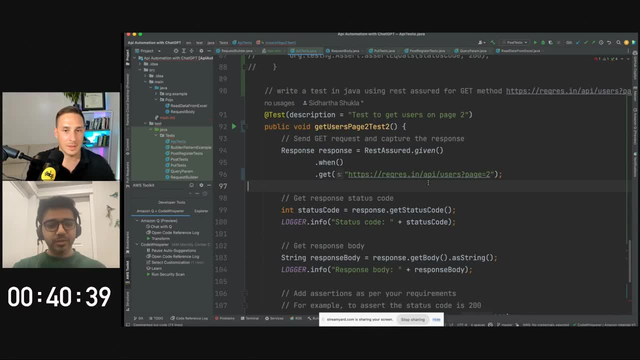 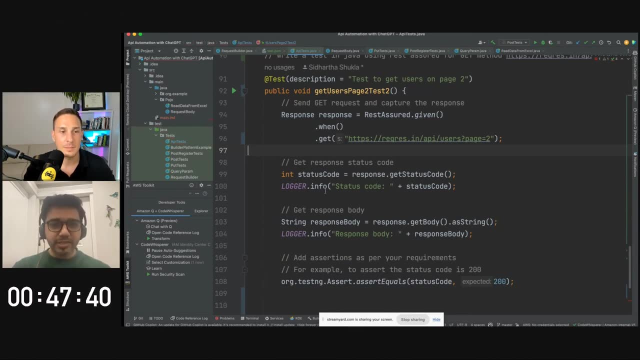 already used base URL. That's why actually it was not Using over the previous code there. i guess that's the reason it was not kind of adding this entire url, but i am adding the entire url for ease. so now we have used response right. we are doing just validating the status. 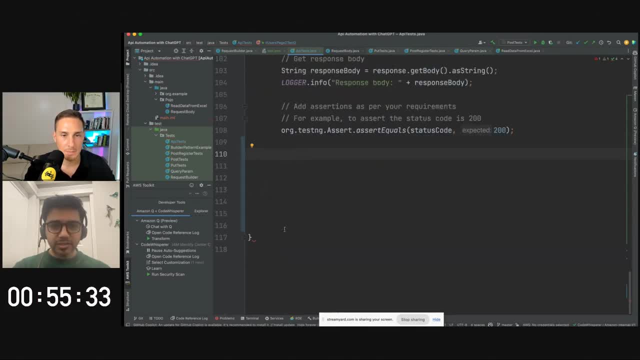 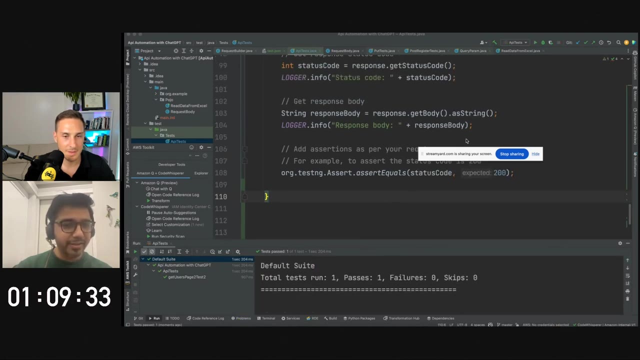 code assertion i am not using, but last it has used one assertion, so let's see if it works or not. okay, folks, let me check. there is one error. i guess maybe it has forgot to close. yeah, so now we can give it a try. run api test. crossed your finger, we are dependent on ai, right? oh, awesome, it worked. 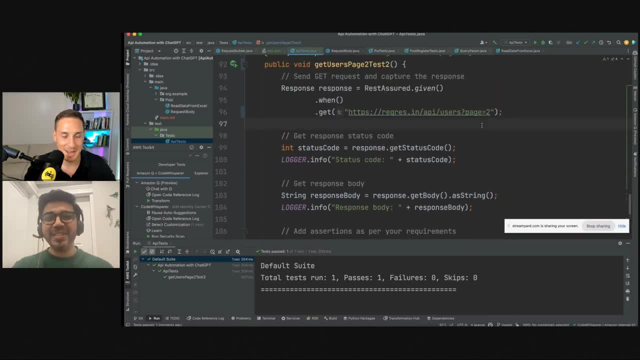 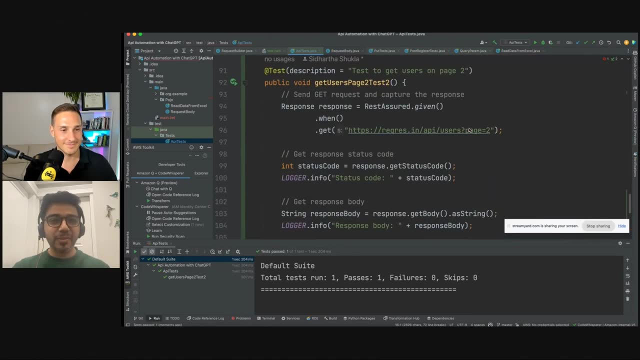 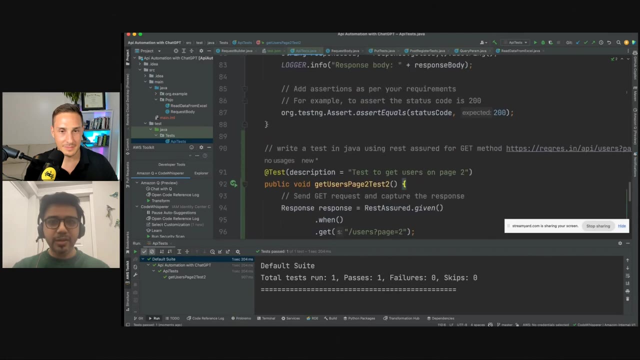 see, yeah, it's not that bad, right, amazing. so we have created it in less than two seconds and the best part is work. i try to rectify it, but let's see whatever code it has created, right? so i'm just editing everything. okay, i just want to be over dependent on ai right now. i'm just using. 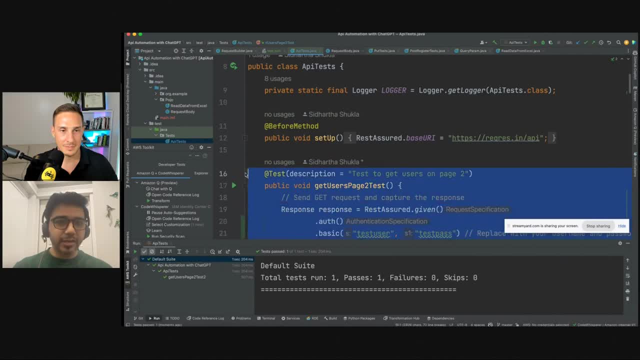 slash users, page two, right, let's see if it is working or not. quickly, i'm just editing everything. okay, i'm just using slash users, page two, right, let's see if it is working or not. i'm just commenting again the existing code. why i'm commenting? because i don't 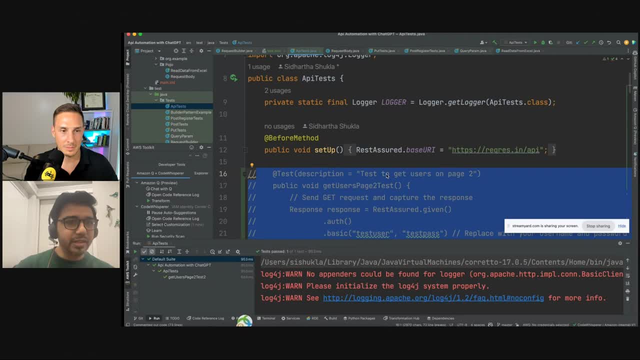 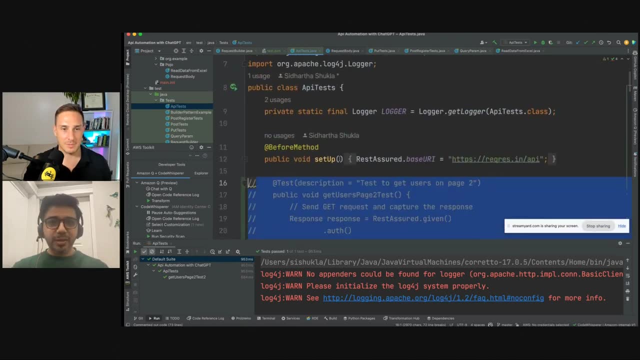 want to execute the entire class, right, okay, cool, let's see if it is working or not with the exact code the ai has generated. awesome, it is working, so i don't have to change this one. why? because in the before method i have already set it up, the base url- and it is so smart that it has already. 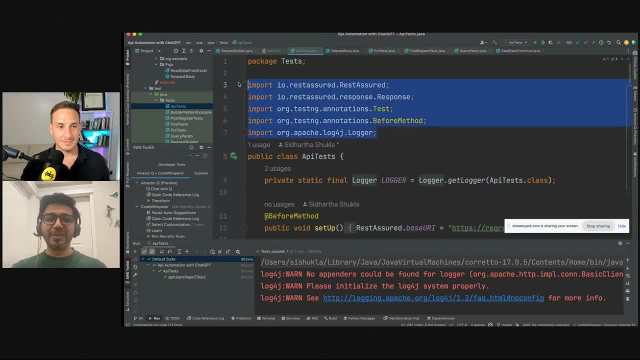 learned from it. right that i have set it up the base url. that's why it was not using the entire url, but one tips over here. folks, if i remove this one and i ask to write, then it will not able to write, because this code generation tool learns from your imports. 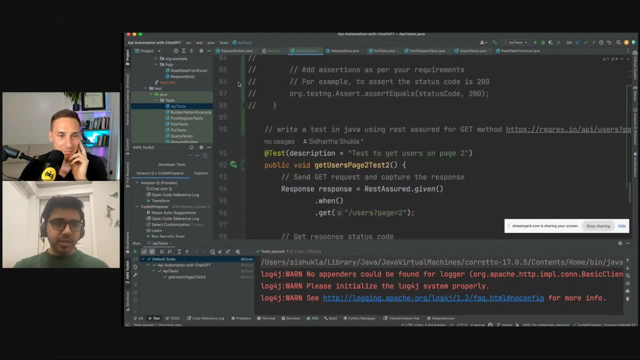 so if you don't do proper imports, it will not able to write. for example, if i will create a new class and just give the command that write api test using, rest assured it may not give this perfect output. so this is just a tips, because if you try right away like this, it may not work and you feel 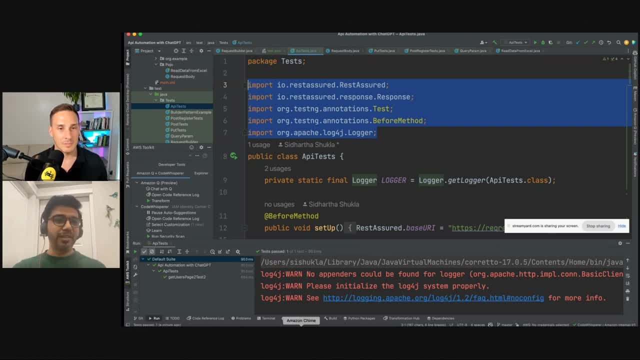 like your ai is not working properly, but, yes, you need to feed it properly with the inputs. make sense, right? yeah, that's a really great tip, sid. so pull in your imports. if you know the technology that you're going to use, you can pull in the imports and then from that the ai will be able to figure out which methods make more sense to use. 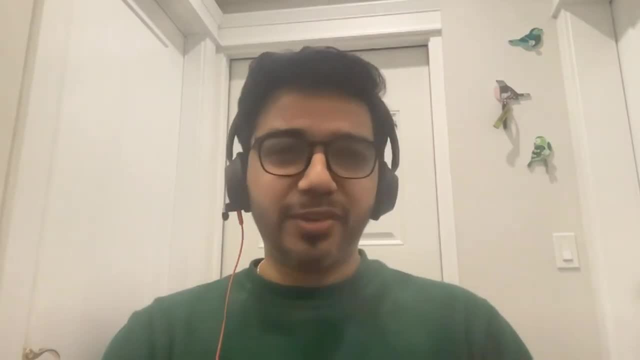 for the task that you assign it exactly. so if you don't write any import, it will not give you this kind of means how we have done. it will not work in this way. it will give you some random code which may not work. everyone just want to take a quick moment for some awesome news, so we have a bunch. 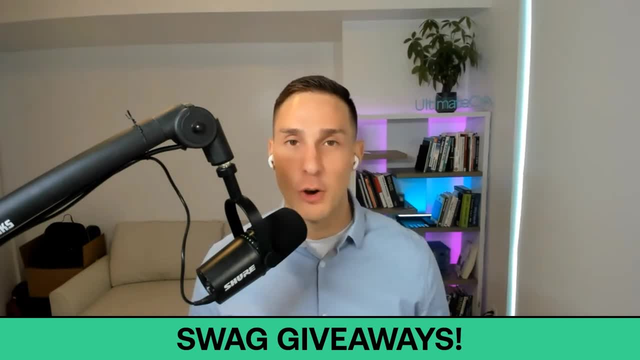 of legacy softlapse remaining and we're trying to give it out. so if you want some softlapse swag, what you have to do is subscribe to the youtube channel and comment down in this video below, and every single week i'm gonna pick my favorite comment out of the lineup and i'll contact you and i'll send you. 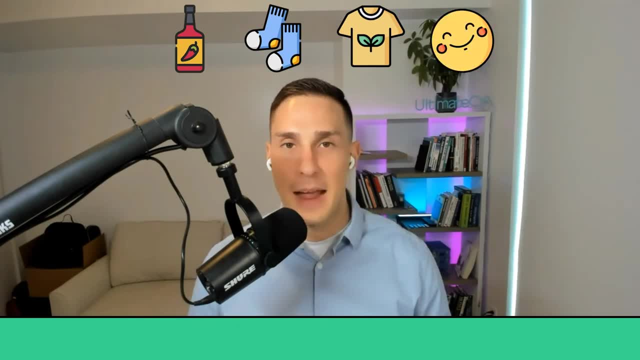 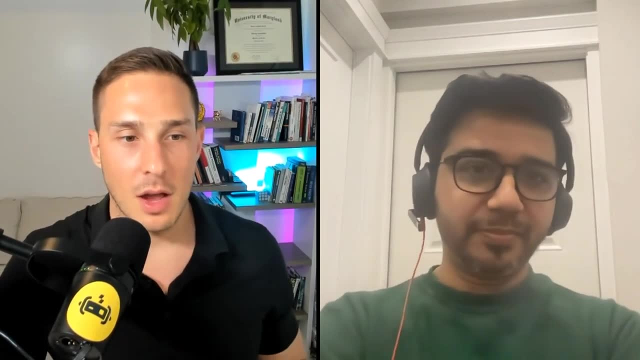 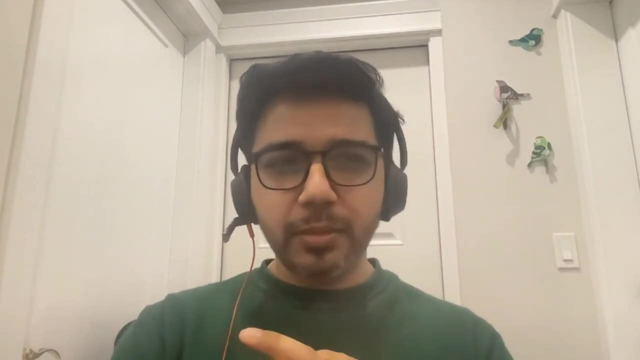 some awesome hot sauce: socks, t-shirts and maybe some more. all right back to the program. i got another rapid fire question for you in 60 seconds. what do you think is the biggest career mistake people make in tech? people always try to miss the bigger picture. what do we mean by bigger picture if they are doing testing? 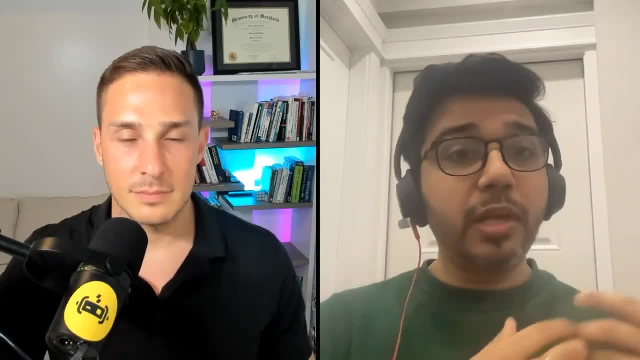 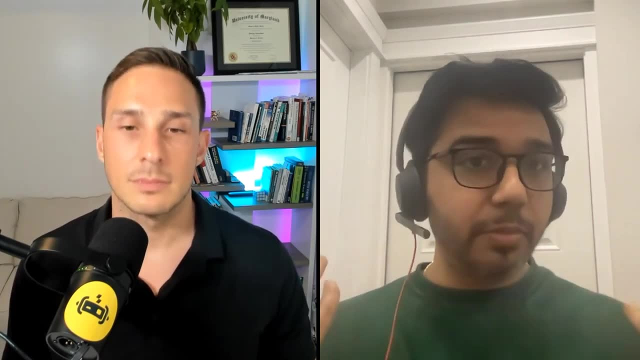 they don't focus on how we can contribute for the architecture things right. when we go for architecture calls i have seen many times that qa folks don't give any inputs right. but you need to have a bigger picture. you need to understand the architecture to give proper inputs. same goes for 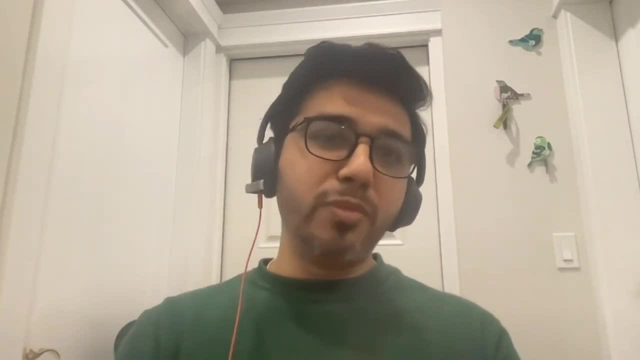 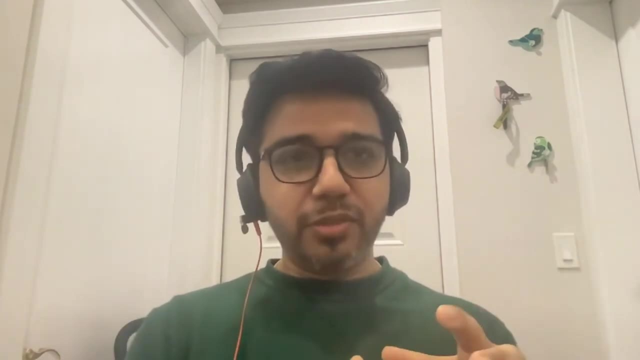 if you are a developer, if you don't look at what qa folks are doing, you may keep on missing those small null checks and many things like that again and again while writing code. so as a dev, you should focus, like what is happening in the qa and understand your entire architecture as a 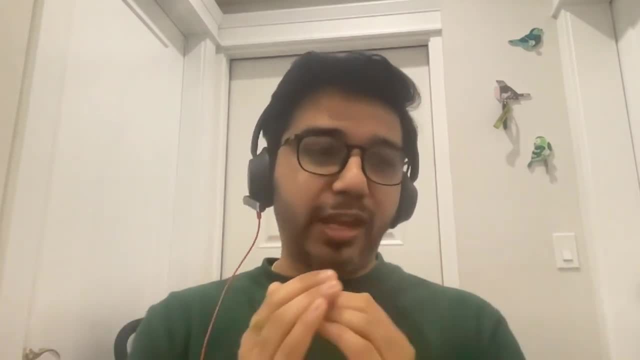 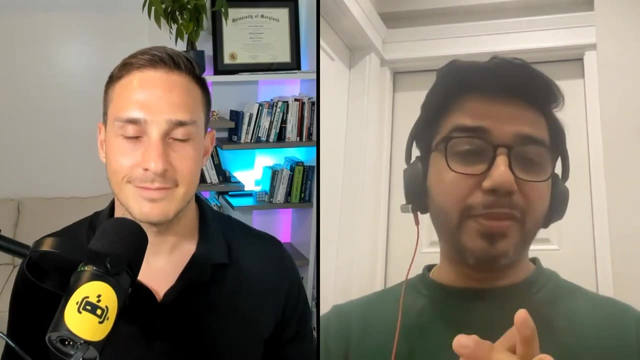 qa. also, you should focus on the entire architecture, not just- okay, i'm testing only a specific feature- that i should not understand the architecture. no, i feel it's very important and, as an sd, as that is kind of a breeze between sd and qa, right, so they have to understand in and out everything, right. 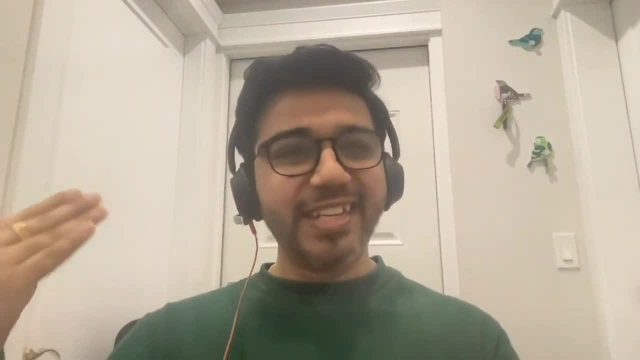 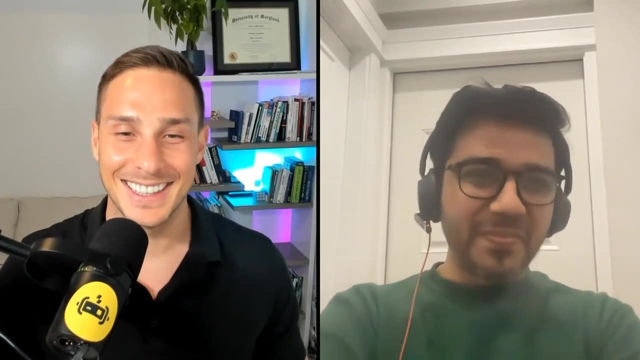 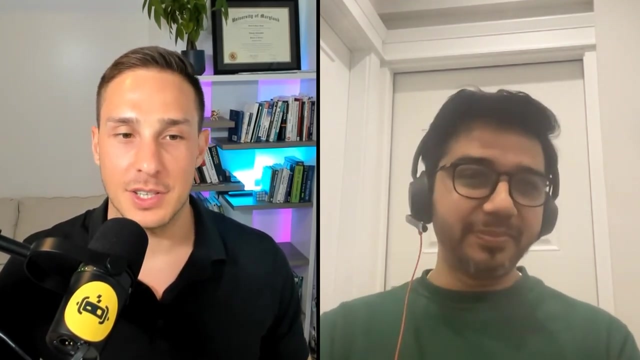 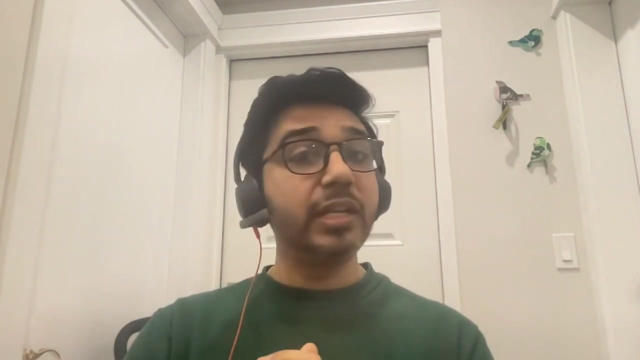 starting from unit test to regression, functional performance, everything. so i sometimes feel as jack of all, master of none. yeah, that's a great way to put it and sid. one last rapid fire question for you: what are your top skills for automation at the amazon? first important skill is how good you are in writing, code, your coding standards and 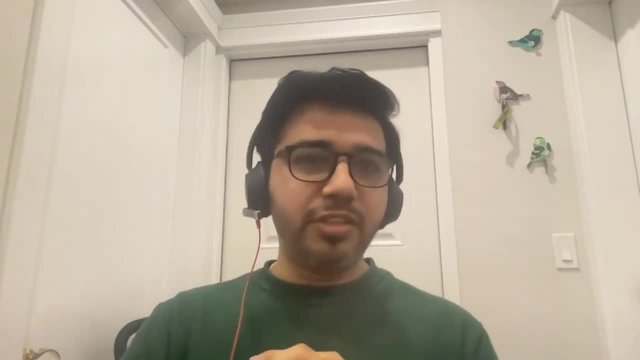 writing optimized code is very important because you know right, you cannot stick to one language. you cannot say: i am good in java, i will not work in javascript. no, it doesn't work like that, right, because if they need in javascript, you have to learn and do it right. so the one thing that i'm 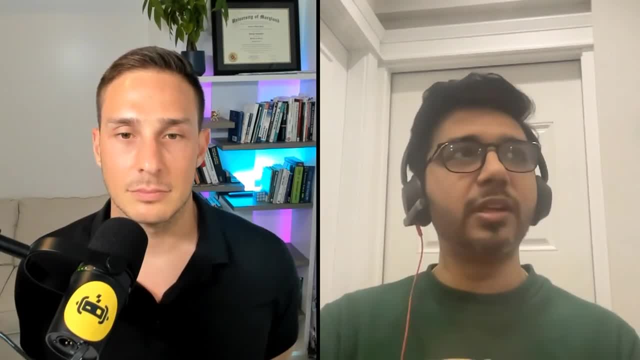 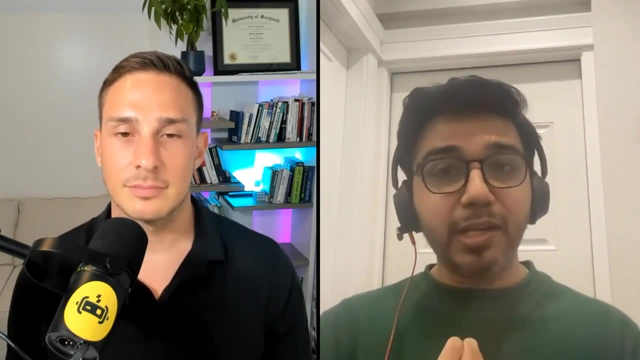 désintéred is going to remain. same is your coding standards and how you write optimized codes. and second thing, how well you understand what you are writing and it's not like juridical. it's how well you understand means. if you are writing a for loop, it's not like you are just. 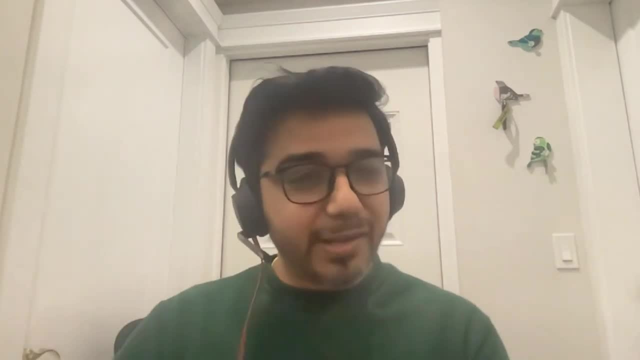 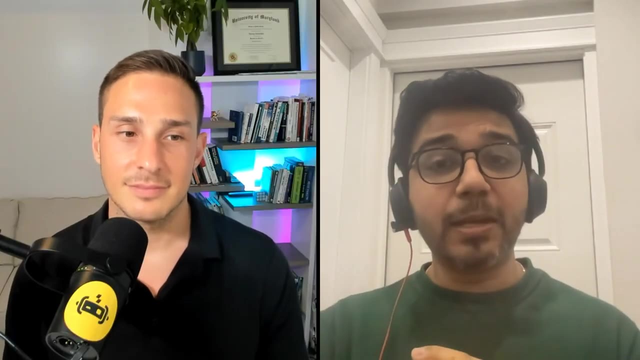 thinking: okay, i need to complete this logic. no, how well you can complete this logic? so you have to always ask yourself how well you can write the code. that is one thing, and the second thing which i feel is like you have to be very flexible. you cannot say like, okay, i will work in selenium as rest assured, no, it will not work. in lycawk, though, i thinkyson as the third one, which means contains зар, not, i am outside. you know it will not work and and that should be it. and then at the end it should be so much longer and far, yeah, and you should keep up theiveness. you want that as long as possible. so 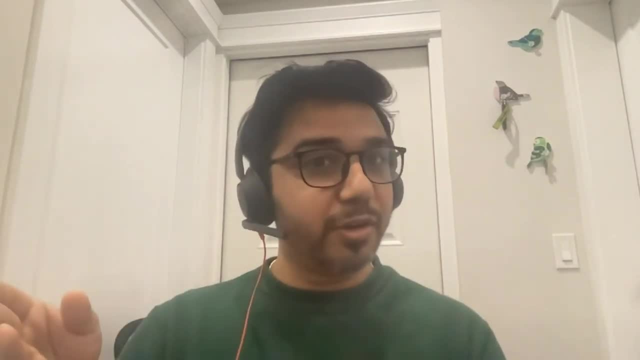 work in that way. You have to work best suited for your project. You will not work on where you excel. It doesn't mean, like you excel in Selenium, you keep on doing Selenium. No, if you excel in Selenium, keep it aside. start learning something new which will work better for your project. 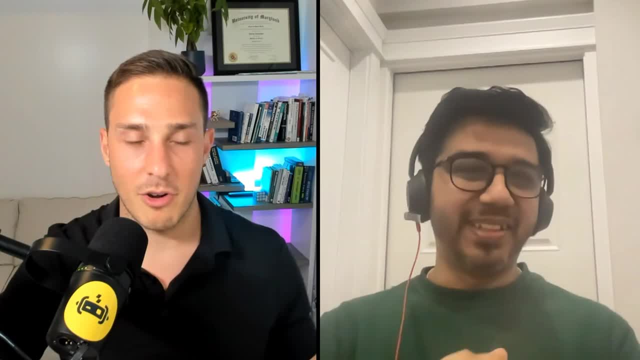 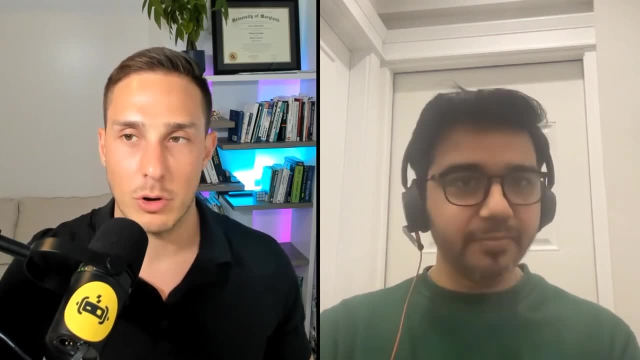 right. So your mindset should be project specific- more Great advice, Sid. So it sounds like thinking about your code and how to write it efficiently is a big and important component of being an asset at Amazon. 100%. You have to write very good code. You cannot write just random code. 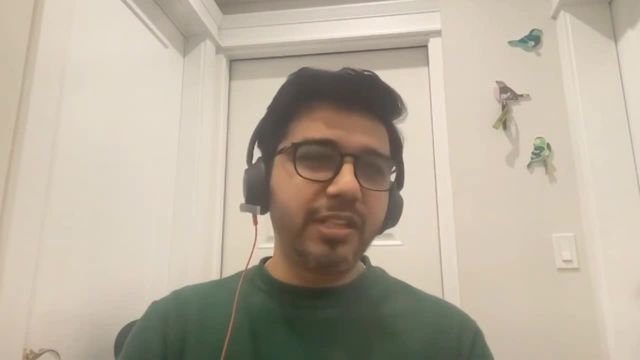 You cannot use just old techniques, right, You have to upgrade yourself and you cannot keep yourself inside. only. I will only write automation scripts. No, you have to contribute for unit test, right, You have to understand how JackoCo works, how code coverage works, how you can efficiently 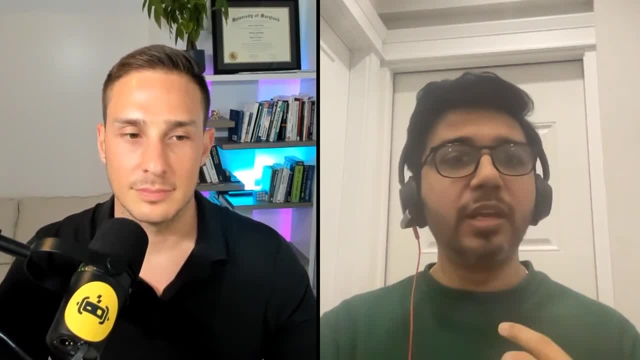 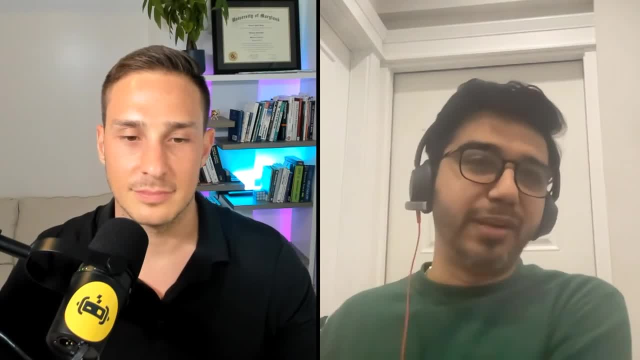 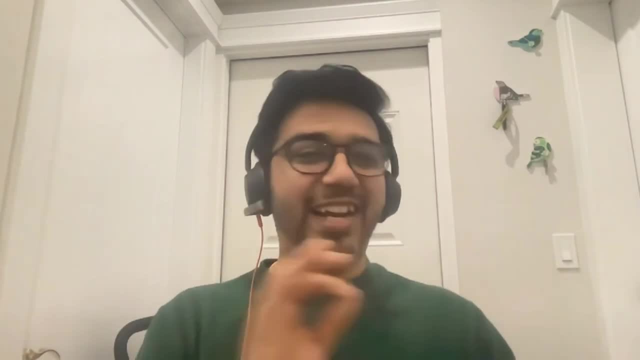 Automation. web automation means web automation, API automation and mobile. no, You have to take care of everything. Everything that starts with test means start, test, start. Everything that starts or ends with test, you need to pitch in, Irrespective of it, unit integration, anything. 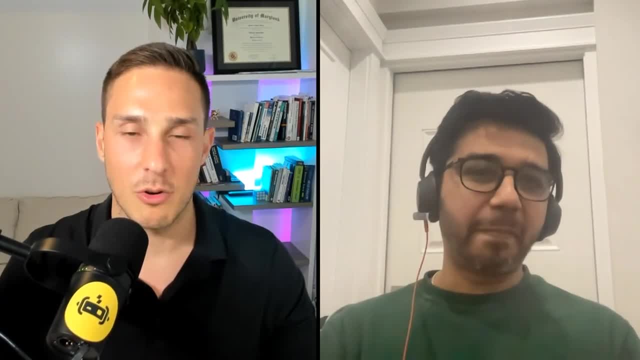 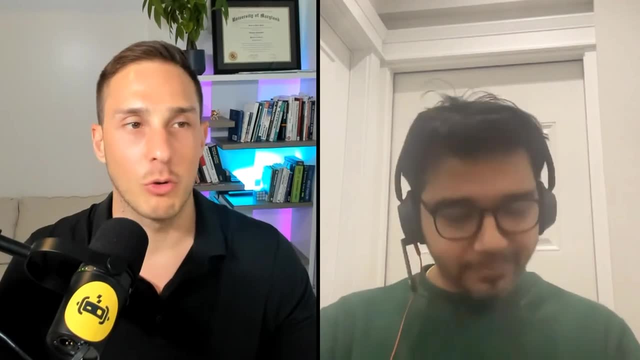 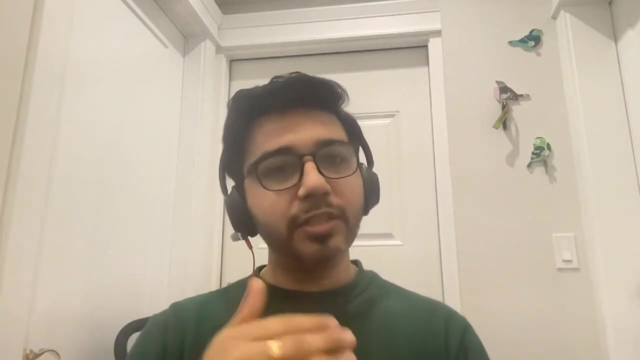 you have to pitch in. That actually brings me about to a great question: being an asset at Amazon, What is your typical day-to-day look like? How much time do you spend coding versus other activities? There are five. There are five important things we do. First, I have to build a distributed, highly scalable 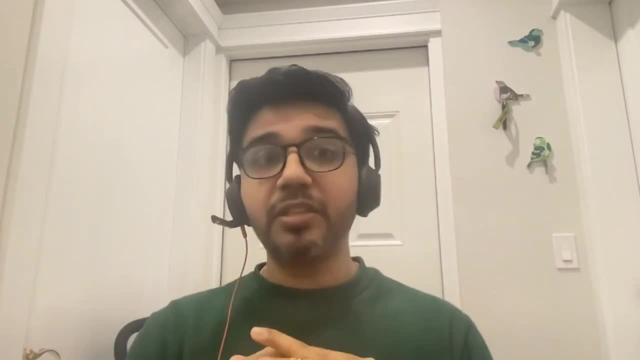 and fault-tolerant systems and services As an asset. I need to write systems and services. It's not like I'm going to only write automation. I need to design services. I need to mock service. I need to work on that. So I need to make sure I have written it properly. first task. Second task. 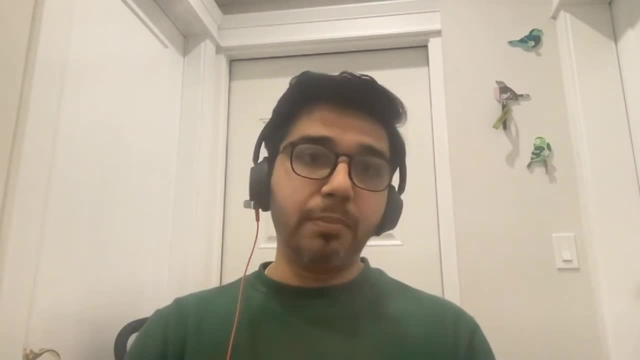 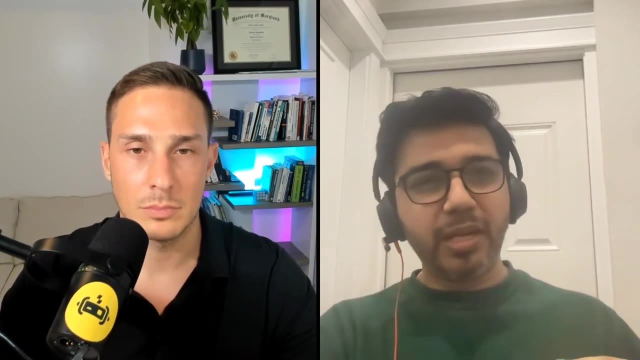 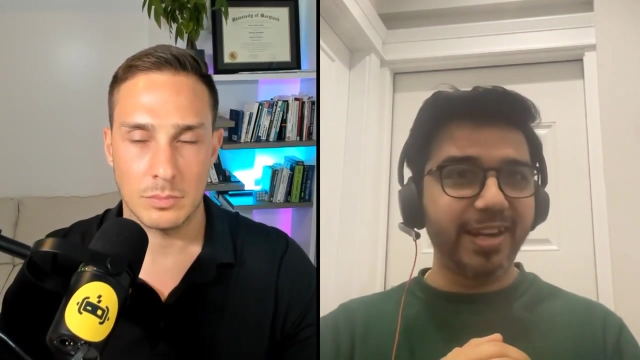 we need to be involved in designing tools, So maybe tools in terms of helping QAs- maybe they are spending a lot of time in fetching some information by going into UI, entering an order, creating an order- We may try to create a small tool internal so they will just put information and it will give them an order ID. 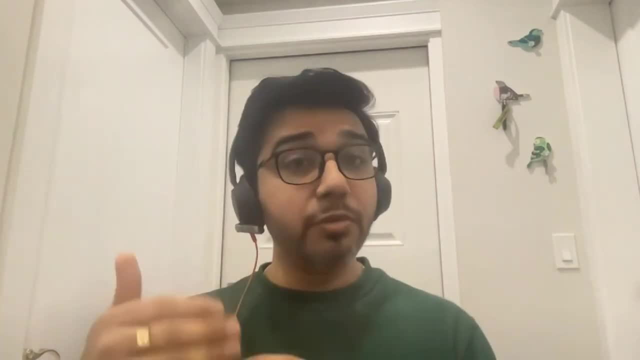 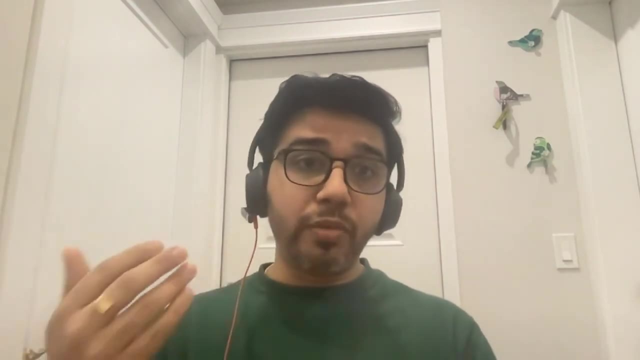 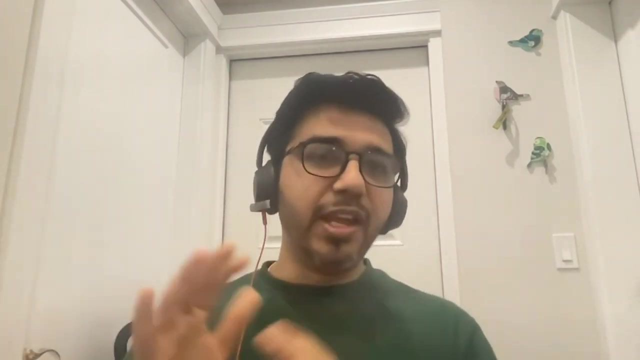 So we need to be involved in designing tools. Third, we need to work on reducing operational cost. So now, reducing operational cost means you may work in latency optimization, You may figure out ways how you can reduce the load on your machine, on your system, on your services. There are many ways, but yes, operational cost. 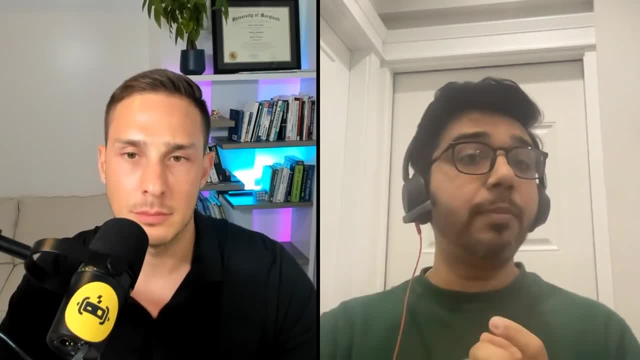 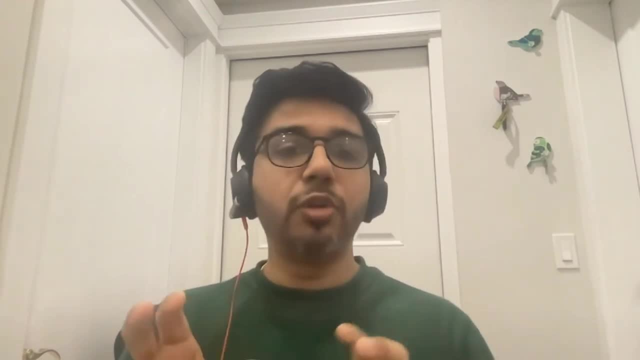 reduction and latency optimization very important. Fourth, you should be able to mentor other QAs So they can write more code or they can contribute more towards the automation. They should not consider themselves for only functional part. Why? Because in a big organization they cannot tell. 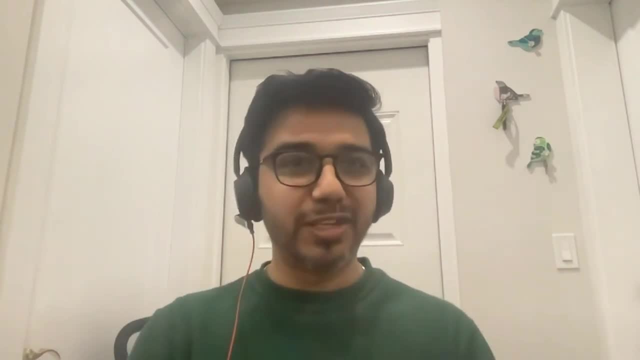 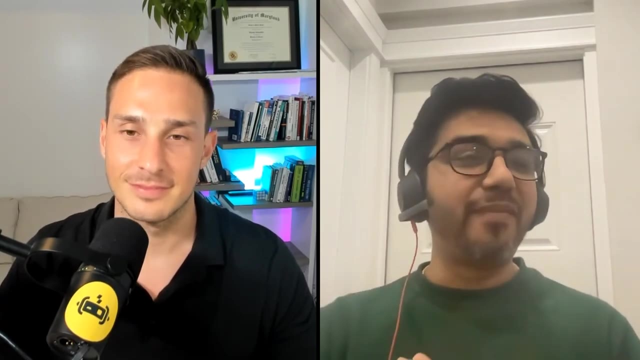 you like. 12 months, I will give you a manual task, or 12 months I will give you automation tasks, right? So you should be prepared for everything. Whatever comes in your plate, just grab it and do it. Okay, And fifth and last thing is more about how you are well-versed with AWS, Because in and 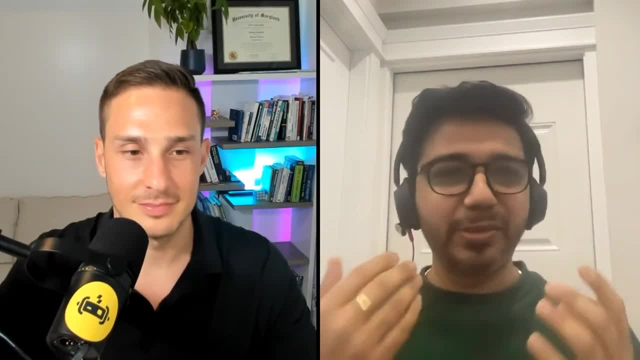 out. you will work with AWS right. AWS CodePipeline, AWS CodePipeline, AWS Code CloudFormation. So everything is AWS. So you have to be very good in AWS service. I used to spend a lot of time in that unit to write. 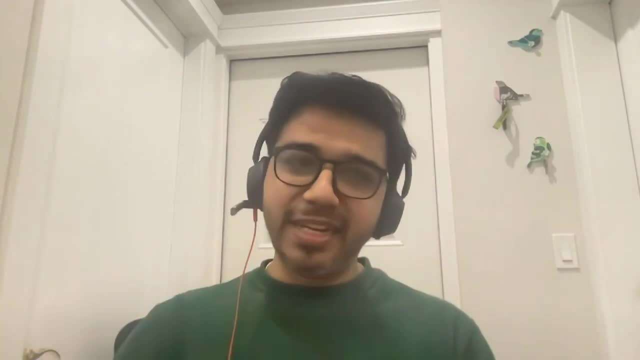 So, starting from infrastructure as code to creating pipeline, to integrating a lot of Amazon internal tools, technologies, frameworks- So yes, AWS is kind of a very important part of our life. That's very amazing. And how did you learn all of these skills? 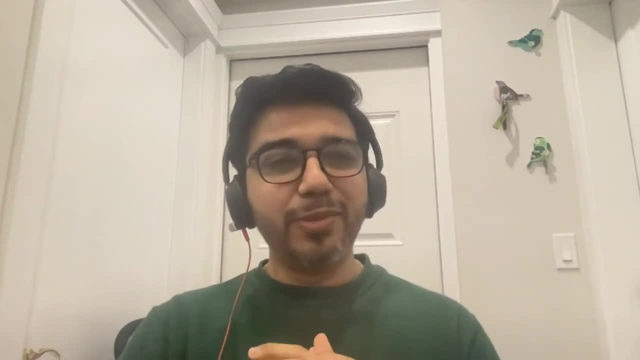 to become an asset at Amazon. I am a person who reads a lot from documentation. I know this is old school, but I don't trust any videos and all right away. I just go to any tools and trust me in companies like Amazon. 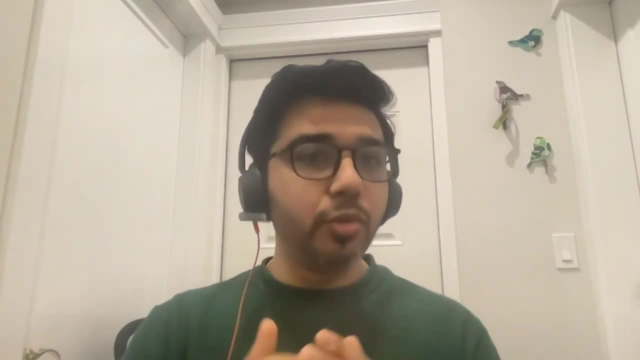 they have put a lot of effort to create very nice documents And if you go through the documents you have that patience. Instead of debugging things for eight hours, watch or read those documents for four hours and you can wrap it up in one hour. 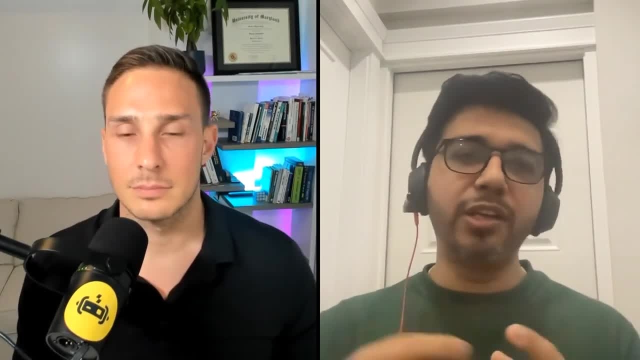 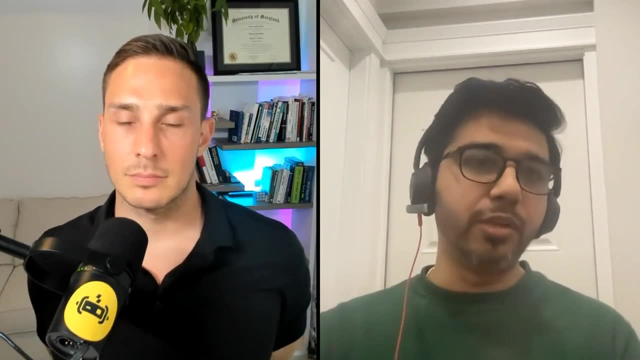 Or else don't go through the documentation, do a hit and trial method and you will waste eight hours. So I prefer to always read the documents. AWS also, I have learned while working and then going through the documents, because AWS documents are really super awesome, right. 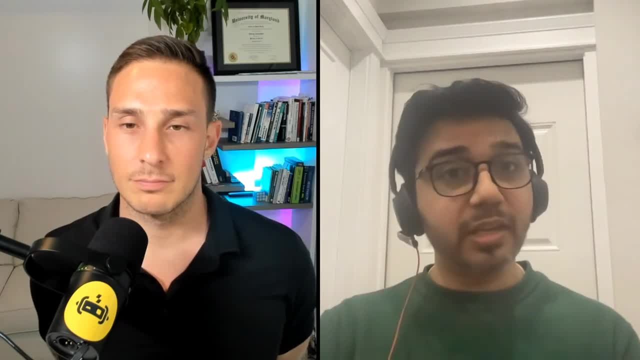 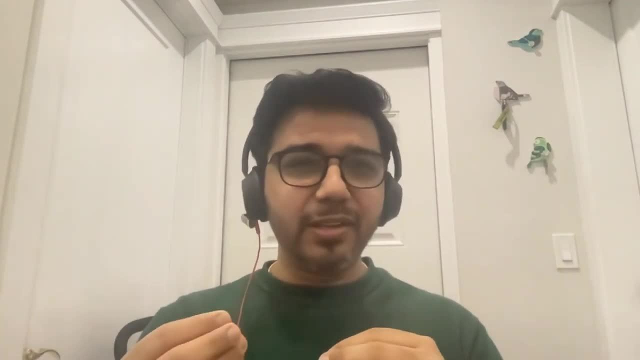 You just go through the documents. everything is well written and nowadays Amazon Q is there. So Amazon Q is kind of a new AI. If you ask anything about AWS or anything about when you get stuck like how to create IAM role, how to create IAM policy, 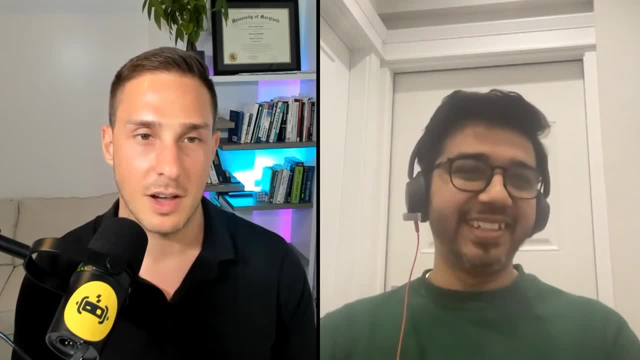 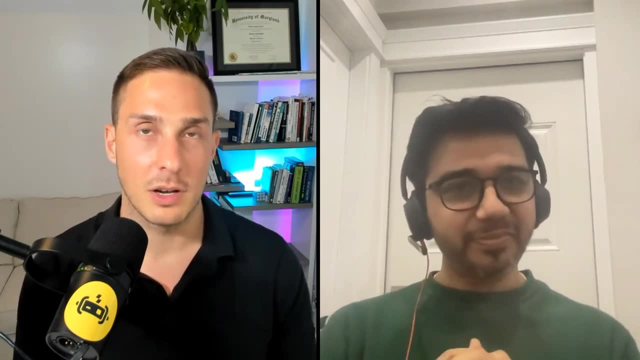 it will give you exact thing, what you need. Great to hear that documentation still works, and it makes sense for sure. If the documentation is good, that could be a great thing. It's a great place for everybody to start. Yes, it saves time right. 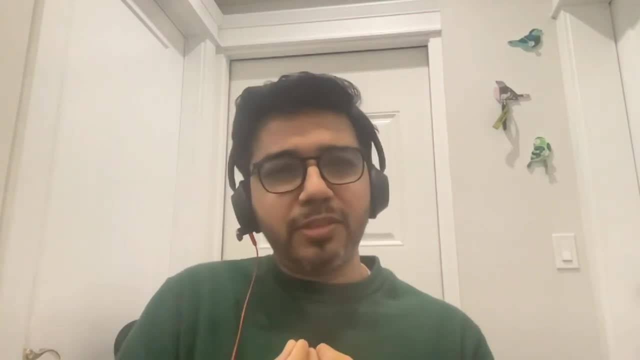 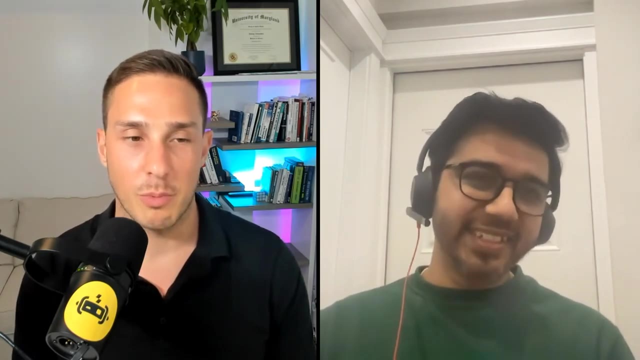 For why to unnecessarily hit and trial? Because if you don't have knowledge about something- I don't think so- you do hit and trial. Gain that knowledge. It will save time, right, That's so true, And you bring about actually a really good point. 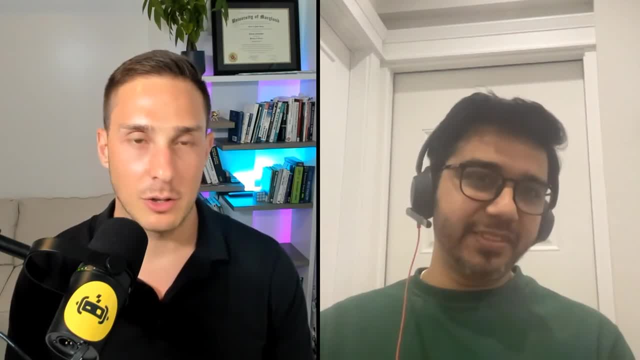 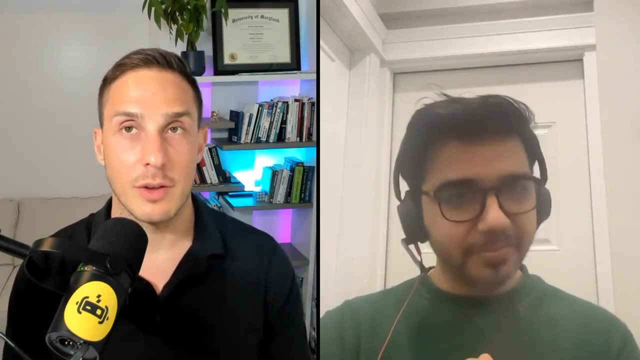 because I'm thinking like for myself: how do I learn stuff? I also look at the documentation, and that'll be a starting point. But if I'm learning from someone else, it's possible they don't capture or they don't get it. 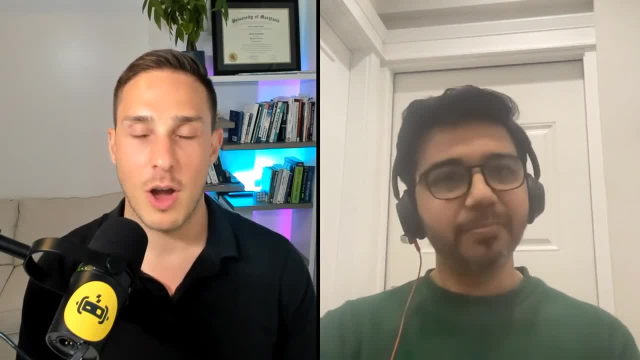 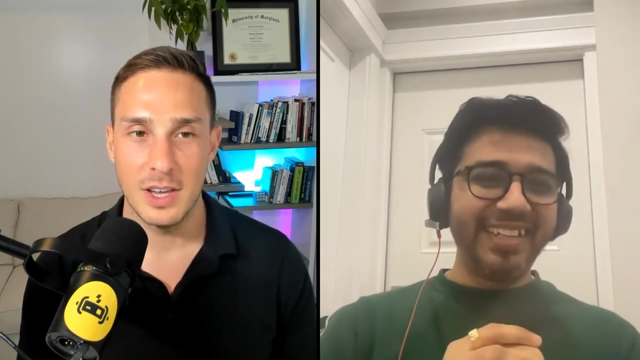 They don't get all the information that is in the documentation, or they translate stuff themselves like lost in translation: from the documentation to their mind, from their mouth into our ears. There may be things that get translated incorrectly, And so now we actually learned incorrect information. 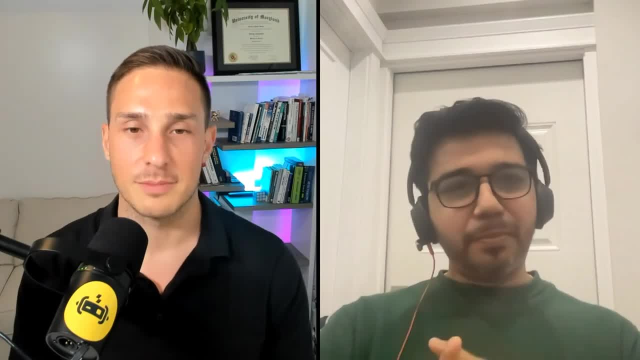 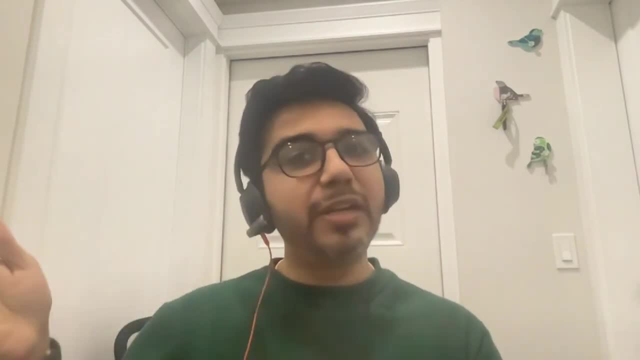 And so, probably, documentation is a great place to start, Because if you see if an SD and QA both read the same document and if you talk to both of them, their perception would be completely different. But you want a neutral one, right? You want to learn everything in and around. 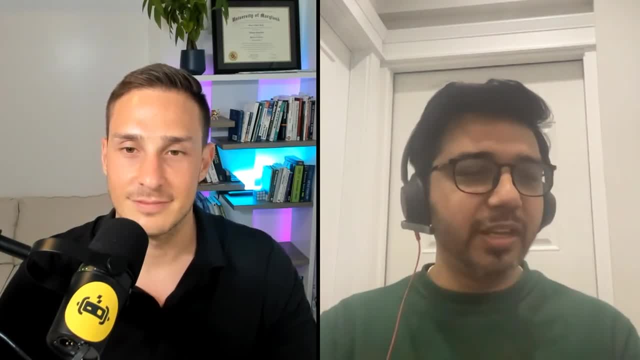 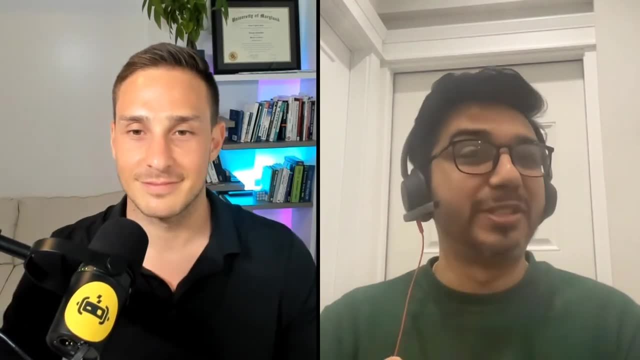 Because I feel, after five years of experience, if you're in IT field, you cannot just assume things. You have to be 100% sure. And how AI is doing these days, you have to be more than 100% sure that what you are doing. 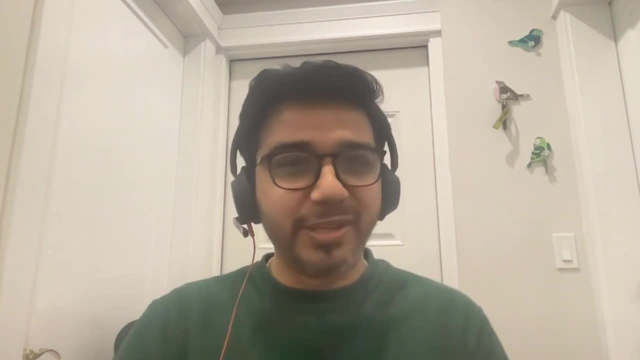 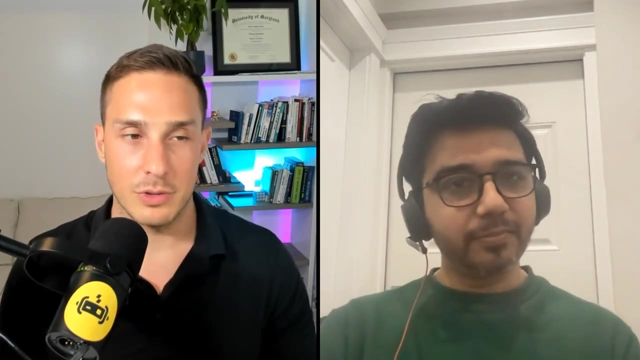 you do understand it right. You're just not doing it randomly by watching videos or copy pasting code. Yeah, great points, Thanks. So you also have a really great background in in helping people improve their careers, And I saw in your LinkedIn profile. 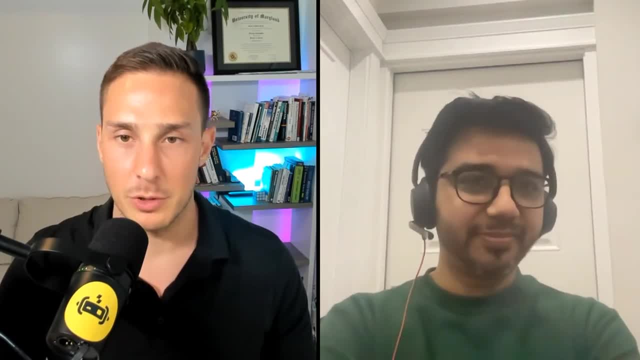 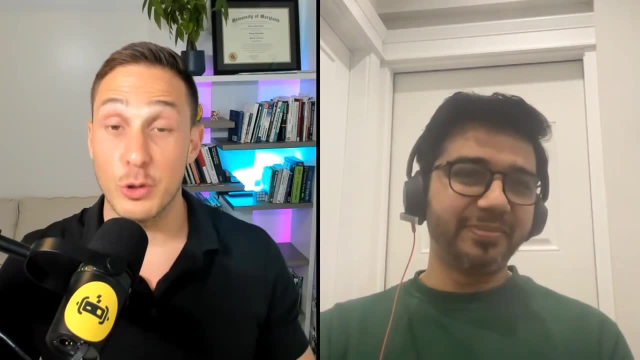 where all your links are available. you provide a lot of like helping people with interviews, providing career guidance. I'd love to visit that in a moment, But before I forget the code that you wrote, I'm very curious about it. Can you show that again and walk us through? 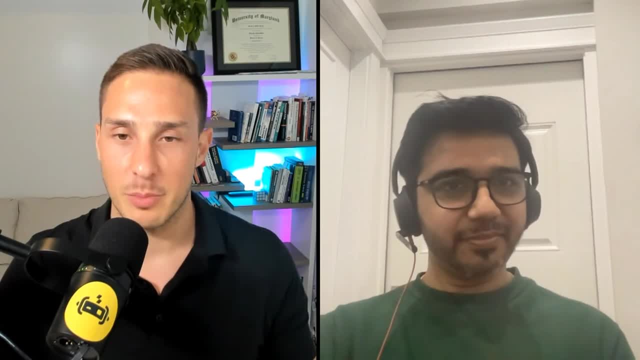 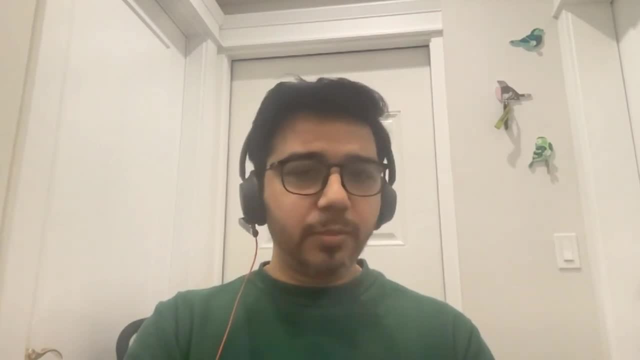 what tools you use to make that happen and teach us a little bit more about it. please Teach us how we can also make that kind of code happen. Let me tell you a very good thing about CodeWhisperer. CodeWhisperer is provided by Amazon right. 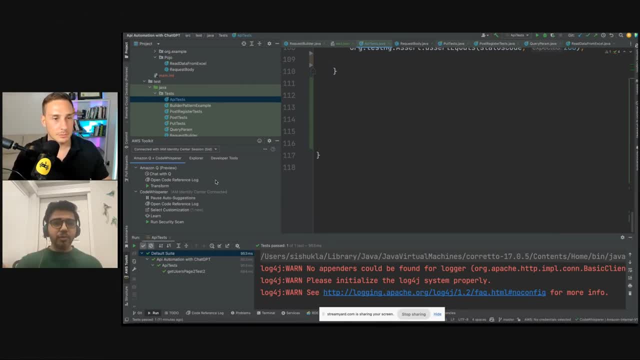 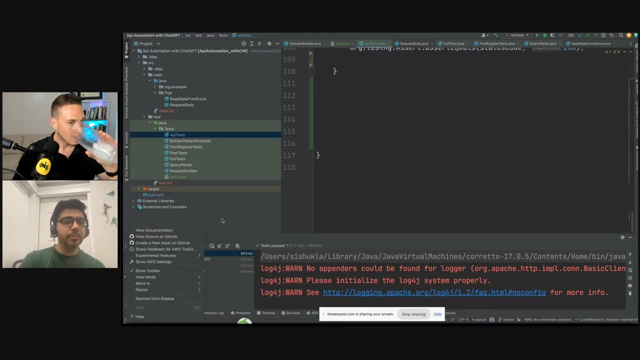 Not like it's for Amazon internal folks, It's for everyone. Whoever has AWS, they can use it. So this is the one. you can see AWS Toolkit right. This AWS Toolkit is nothing but your CodeWhisperer and your Amazon Q, both coming together. 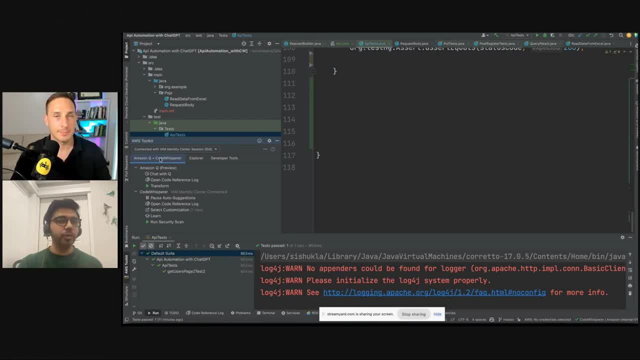 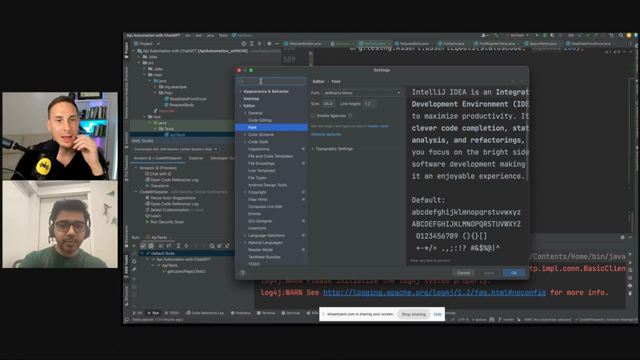 So now, if you are a person who want to set it up fresh on your IntelliJ, what you can do. you can go to IntelliJ settings and plugins. okay, Go to IntelliJ and go to plugins over here. Plugins- okay. Once you go to plugins, go to AWS Toolkit. 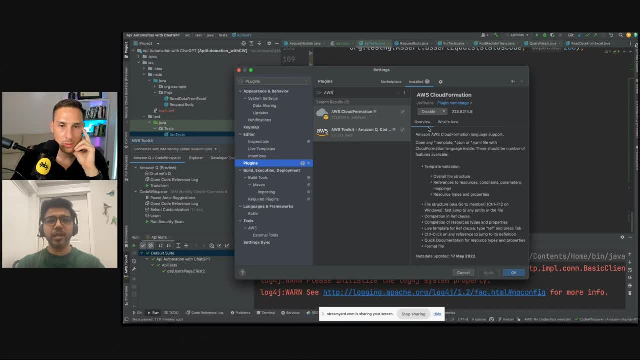 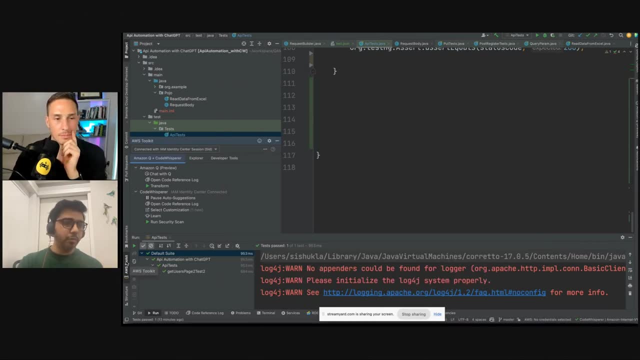 Can you see over here This one? just install this one. I have already enabled this plugin. Just install this one. Once you install this one, you should be able to see something like this over here in the left bottom part of your IntelliJ: 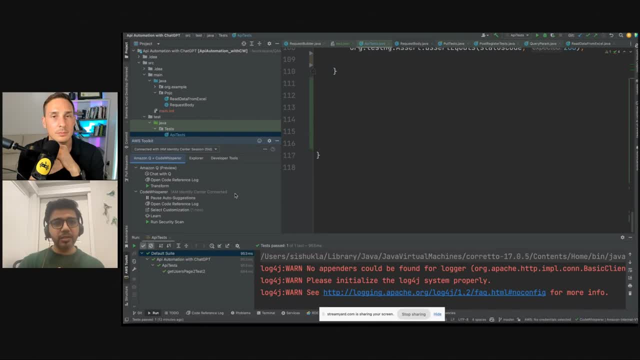 Now click on that. I have already logged in. So when you first time try this, it will ask you to log in. So either you create a free account with AWS or, if you have an account already with AWS, use it. You have to log in for the first time. 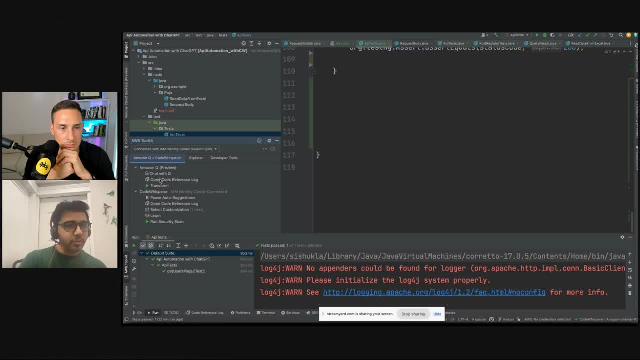 Once you log in, it will show you these options. So Amazon Q is, you can say, an advanced version of ChatGPT And CodeWhisperer is kind of your fellow mate who knows everything about coding, or maybe who can help you to write code better, right. 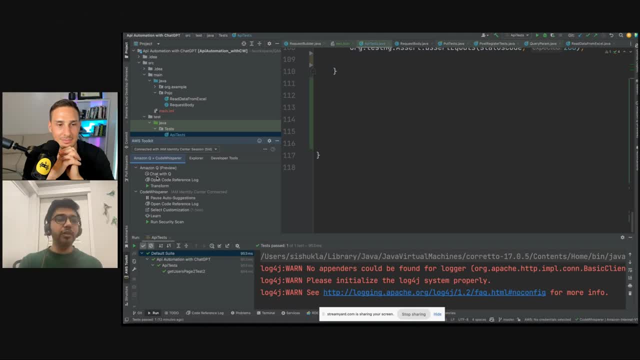 So CodeWhisperer we use to write better code and Amazon Q we use to chat, For example. I have a doubt like how to create EC2 instance right, For example, right. So now what it will do, it will kind of go through all the documents available. 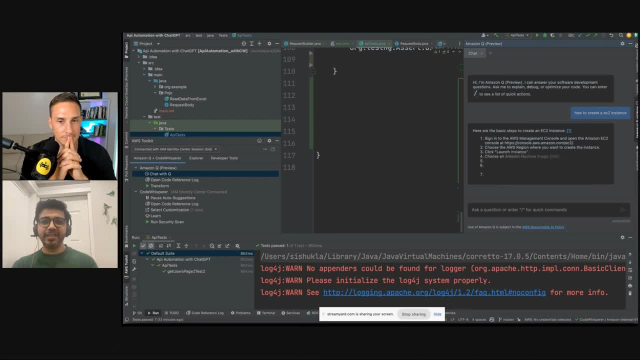 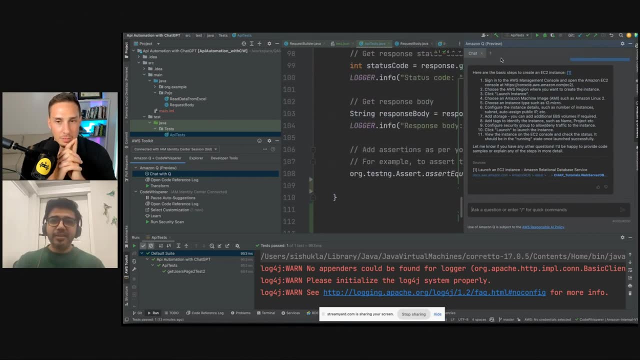 and then it will try to figure out. see, Isn't it awesome, right? You don't have to go to ChatGPT and do it. over here, You can do everything out of your IDE. You don't even have to leave your IDE for the docs. 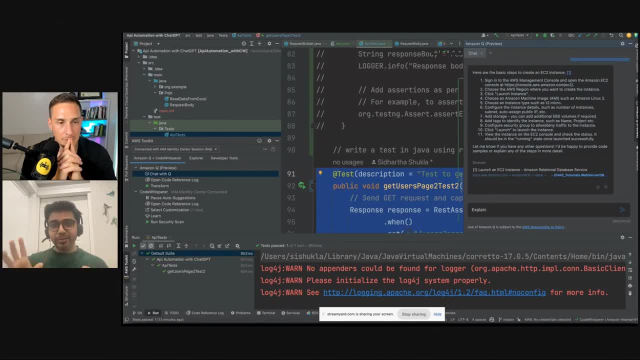 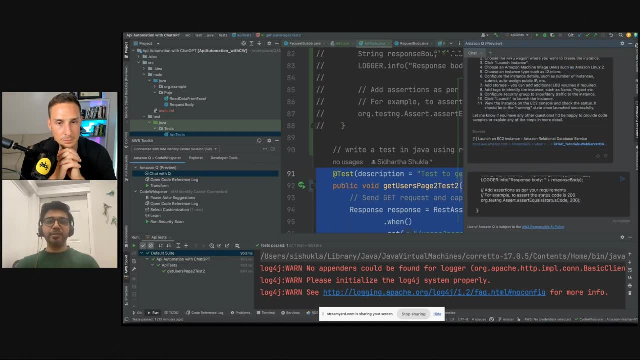 This thing every folks need to understand and I want folks to use this one. You are working on an existing framework and you don't understand some piece of code? Just use explain. Enter the piece of code. It will explain each and every line. 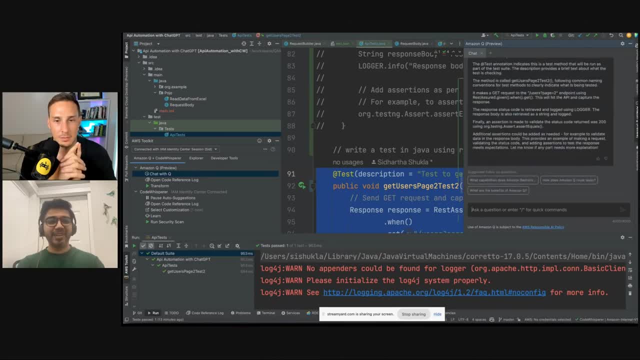 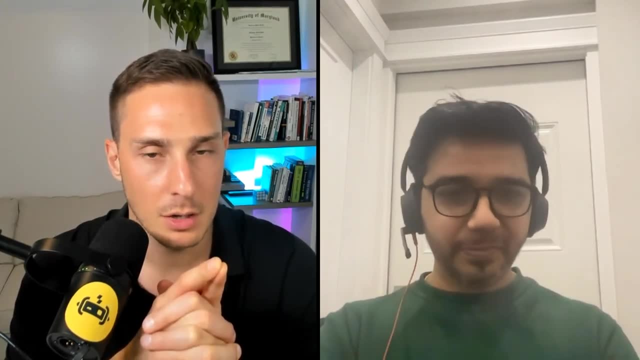 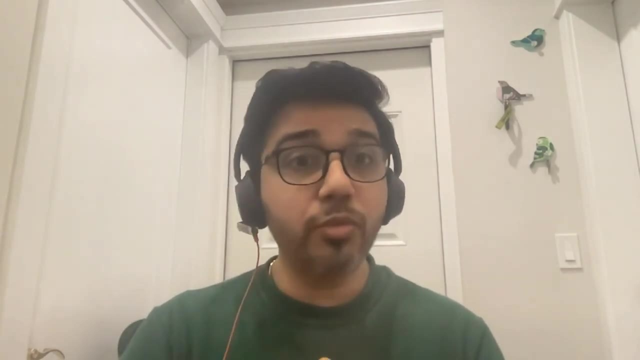 See, Isn't it awesome? right, It is awesome. Q. is that trained only on Amazon data or it's trained on a lot of other data? It trained a lot of other data and if you have a AWS license, you have the possibility to train it with your own data. 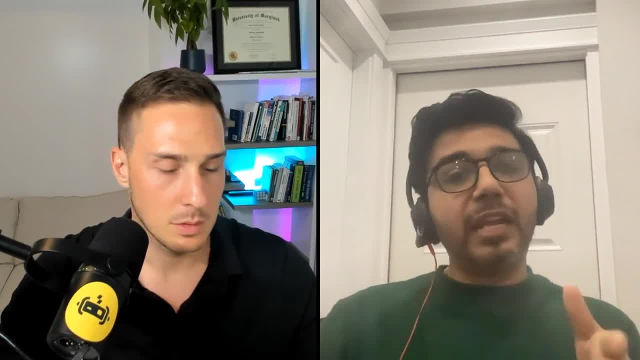 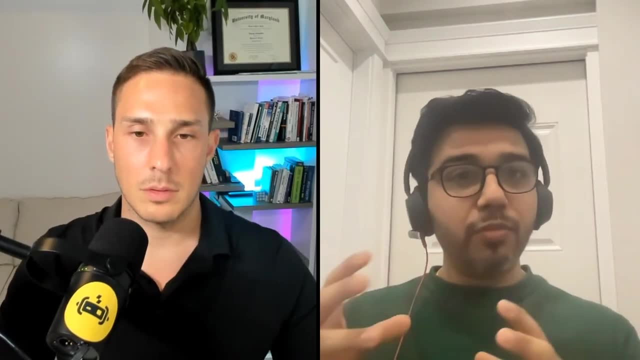 Isn't that awesome, right? Because rather than, for example, stale element exception, if you ask stale element exception, it will give you a generic answer. You may have some exceptions in your own project, and if you want to train it according to that, 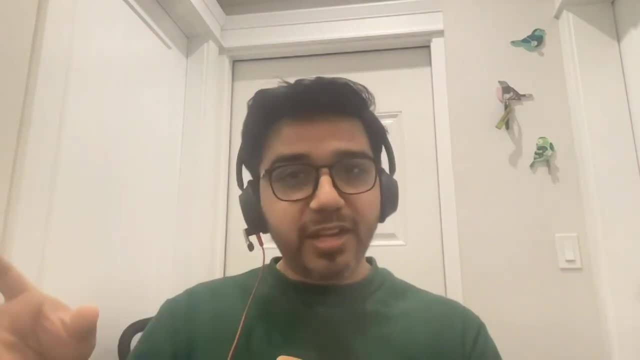 and tell Amazon Q that, instead of giving me generic answer, figure out the answer from this document, So it's not like you have to always get the generic answer. If you want to train it, you can train it. For that, you need to have AWS licenses. 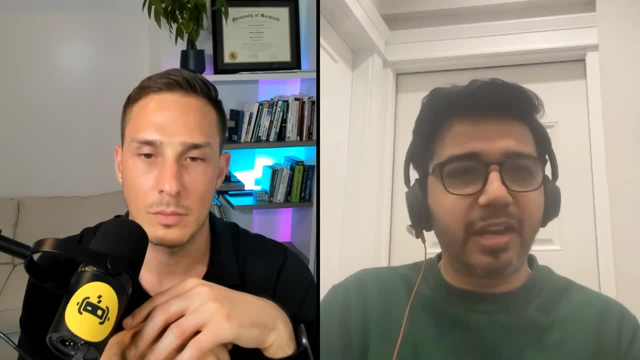 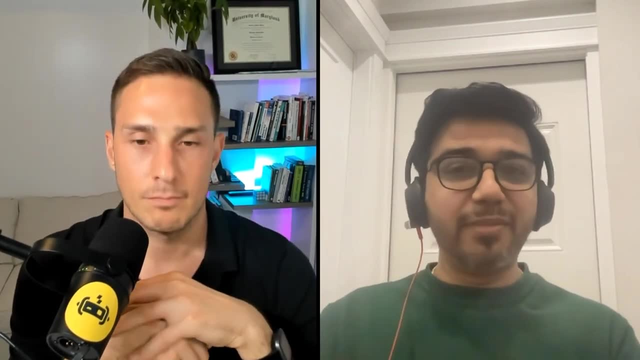 I guess most companies has AWS license, So folks can give it a try. It's not painful And if you don't have also no need to worry. If you want to give it a try, just create a AWS free account and give it a go, right? 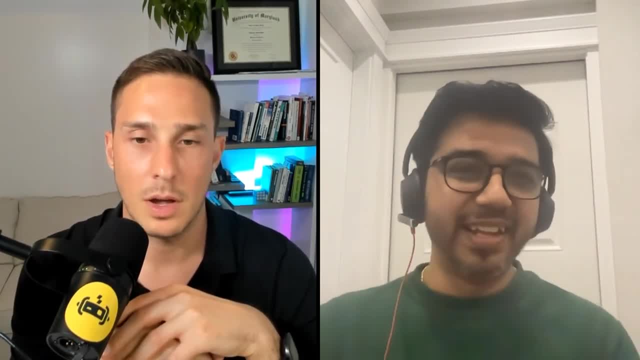 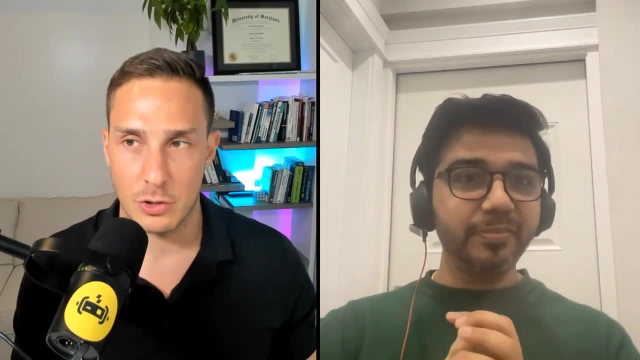 For first-time user. give it a go with a free account. right, It will work. CodeSparrer suggestion is unlimited for free account. There is no limit on it. That's what I was going to ask. Yeah, CodeWhisperer suggestions are totally free forever. 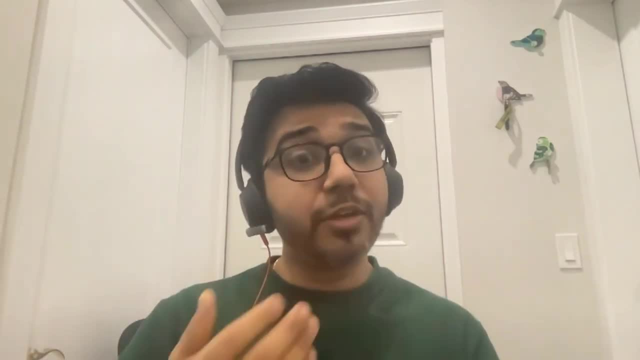 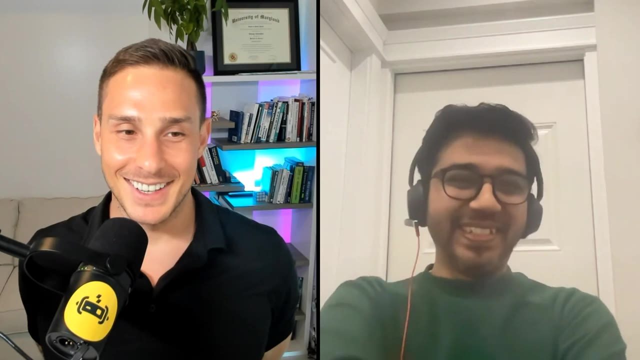 Exactly So. it's cool. There are many more features of CodeSparrer. right, You can do a security scan also of your existing code. There are a lot of things and now I feel I should create a course around it. Yeah, I think you should. 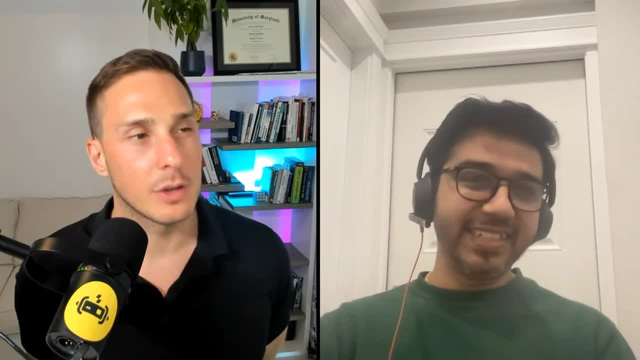 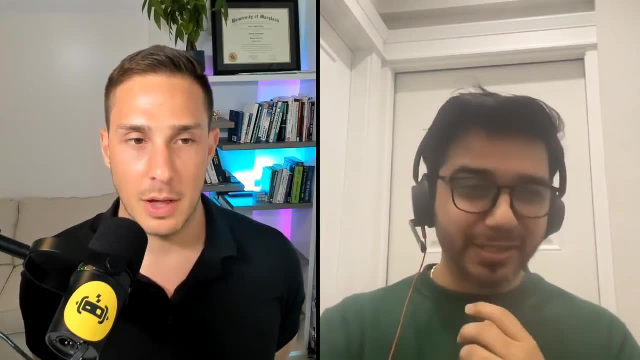 That would be super awesome. I would love to take that course. That's really cool that it's free, because you know there's like a plug-in like GitHub Copilot. Yeah, I do use GitHub Copilot also in my machine. That is not free. 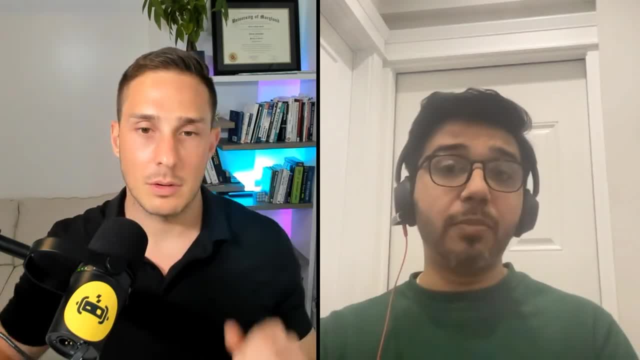 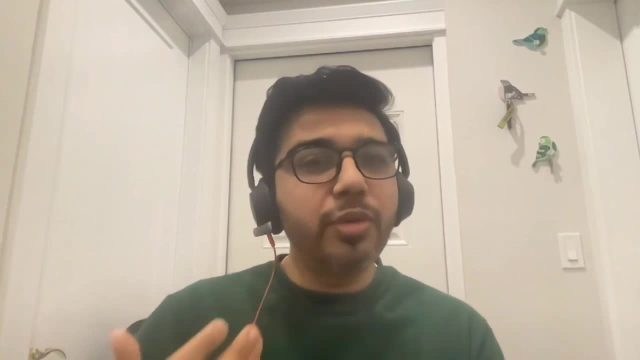 It's 20 bucks a month. I do have GitHub Copilot right now, but I feel Copilot we need to pay and sometime it takes time for us to gain that expertise- how to use it efficiently- right, And I feel during that time it should be free, right. 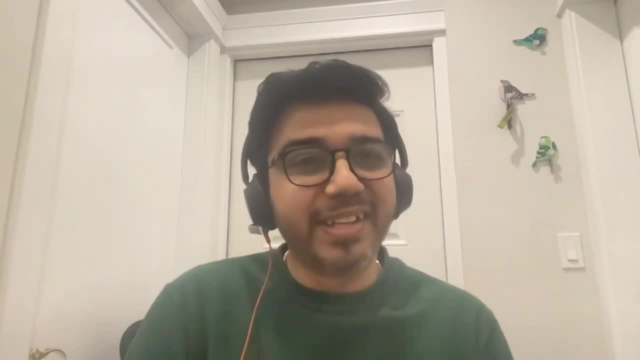 Because you are learning, You don't know what to ask, What is the right prompt to ask? So first, two, three months, I would suggest everybody to try it for free with CodeSparrer, Then they can figure out okay. 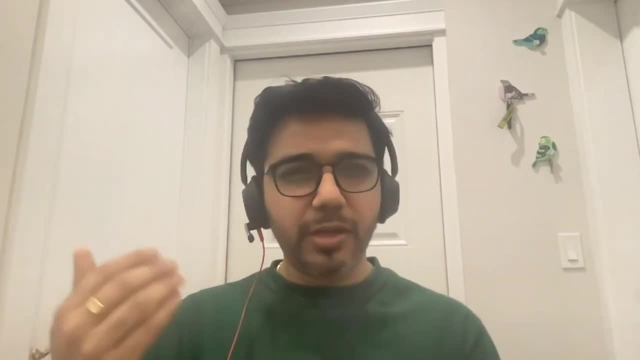 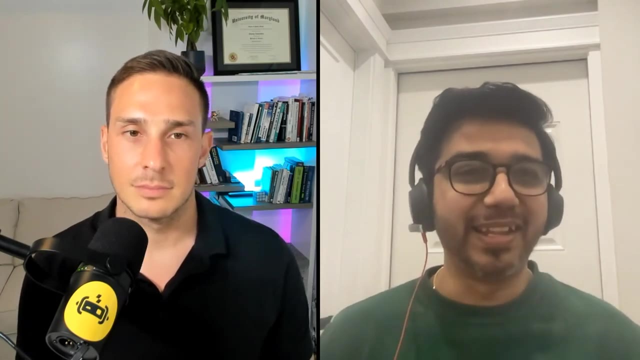 we are going to go for a licensed one, because with the licensed one you may get a lot of little bit more options. But for that you should be first kind of a pro in that right. At least in this era we don't have to pay money to explore things. 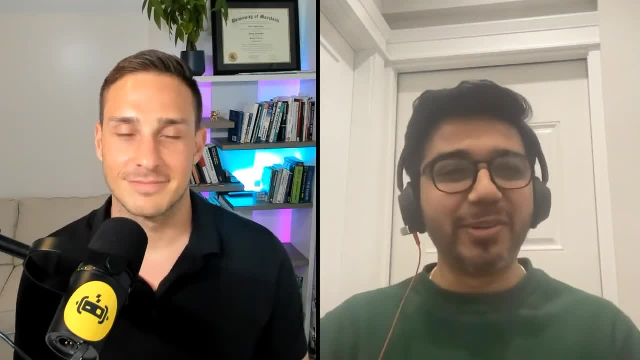 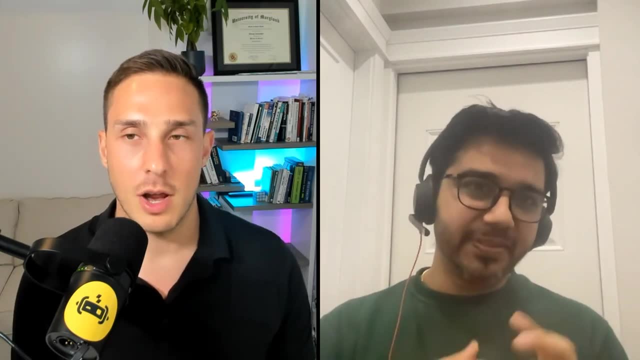 That's what I feel right. So if you're exploring, go for CodeSparrer for sure. Copilot I have also used. Both are pretty cool. Q and CodeWhisperer- are they trained on some existing LLM? 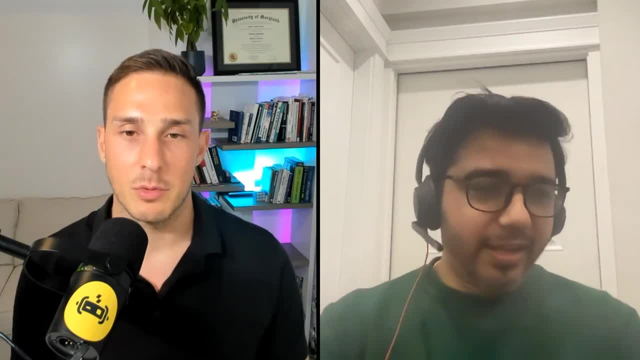 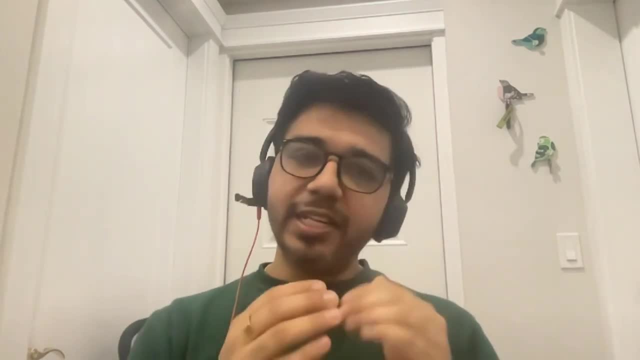 Is it an Amazon special LLM or is it some other LLM that we know It has some Amazon specific. I will give a link on that because it's a very big topic. What happened actually? CW is built on top of Amazon Q. 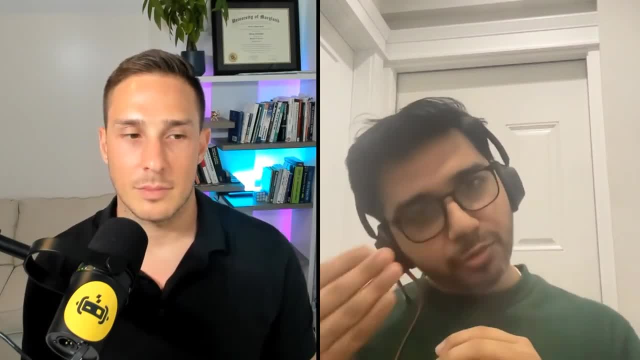 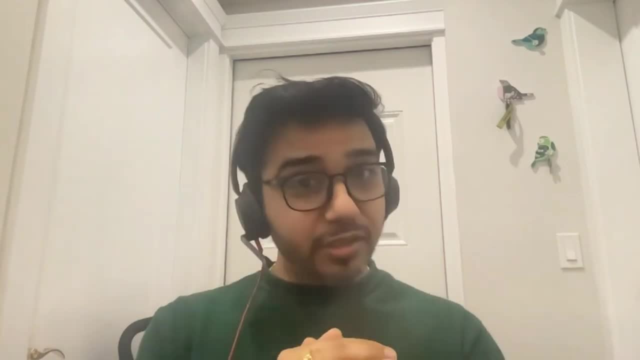 So what you are seeing in Amazon Q, CodeSparrer has used Amazon Q to do that. So, basically, if you see, this is Amazon Q. CodeSparrer is built on top of Amazon Q And Amazon Q has a lot of LLM models working behind it. 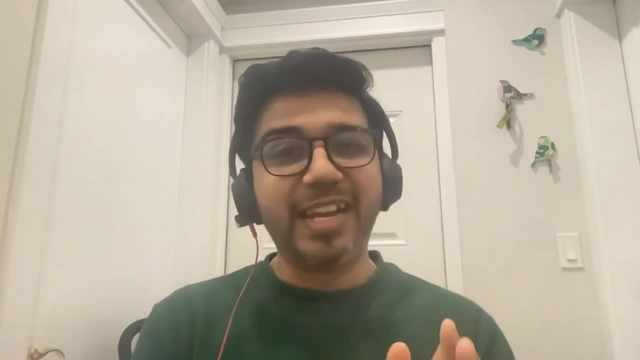 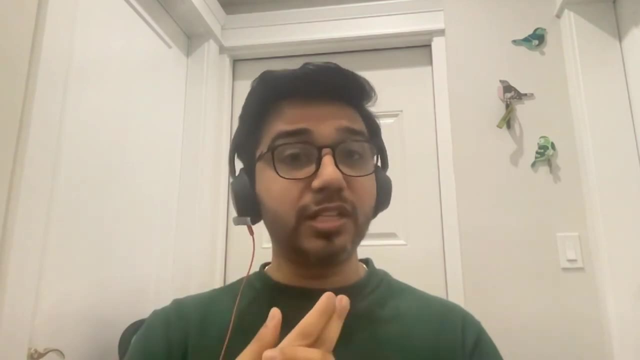 So maybe I will give a link, because it's a very big topic, because it's not only LLM models. There are a lot of things working behind Amazon Q to make it work, And that's what I told that. why a lot of things? because so that they can give you a customization option. 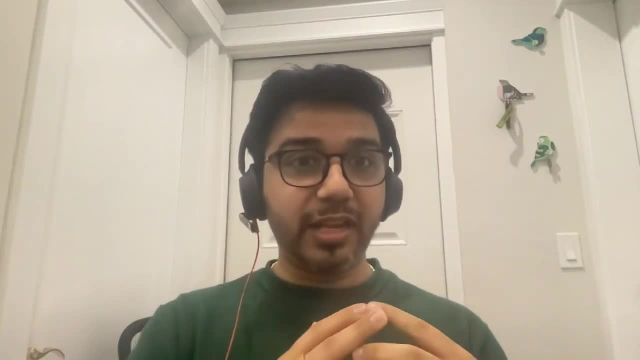 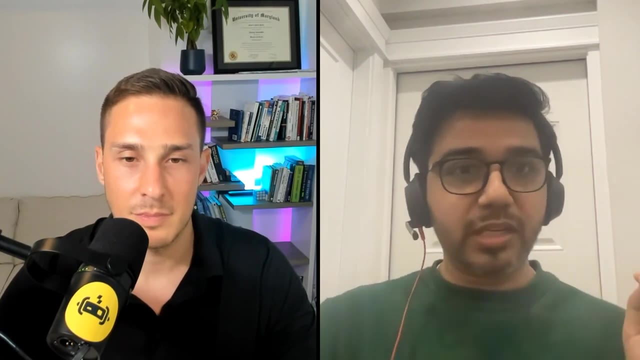 Also, you can customize. it means you can feed your own data, So that's not like it's feed on only a singular specific data. For example, GPT is only trained on some specific information, right? You cannot customize it. Now it is, I guess, in GPT-4, they have given the option to customize. 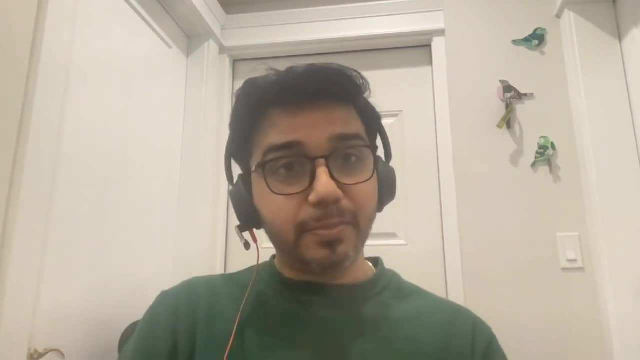 I'm not sure, though, but good, Amazon Q, you can customize it. So you can use this LLM models and you can customize it. Or if you are a very much into tech person, then you can create your own LLM. 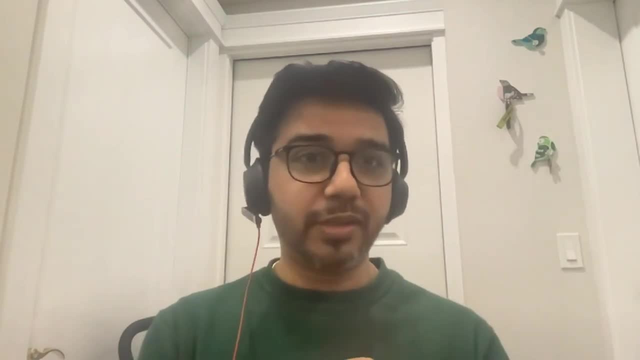 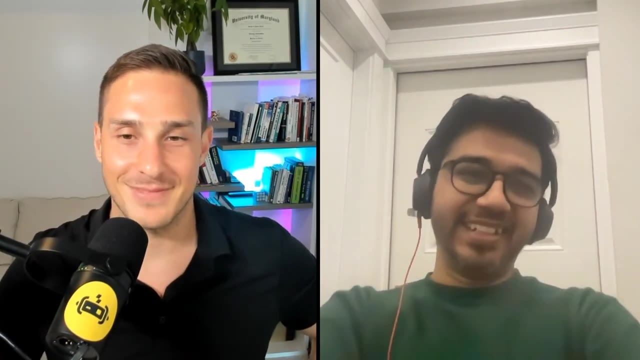 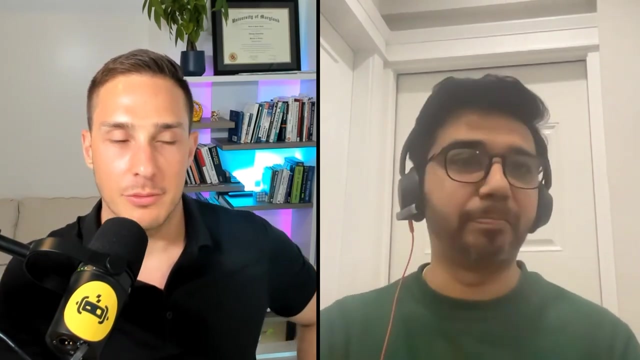 You can create your own pattern to do the analysis on top of it. Yeah, absolutely. Now I'm excited to play with this after we get off our interview, Sid, circling back to some interview advice from you and some career advice which you do a lot of in your experience conducting mock interviews: 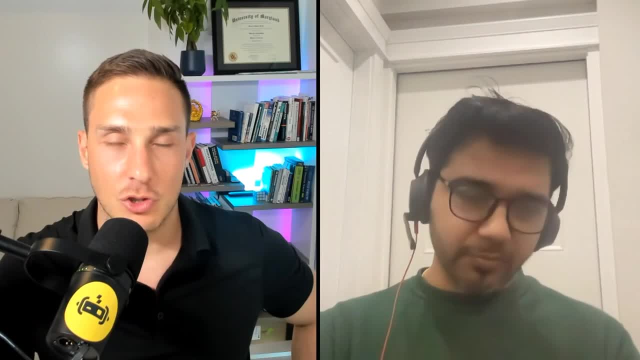 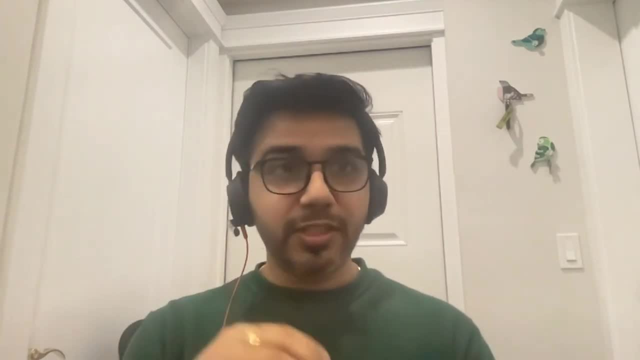 What common areas do candidates struggle with and how can they prepare better? Okay, So there are two things. I have seen it a lot. Just to mention before: due to my mentorship, I was featured on Times Square- also believable. I have contributed to a lot of folks. 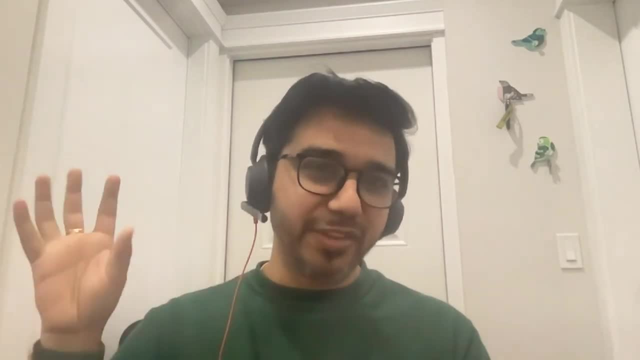 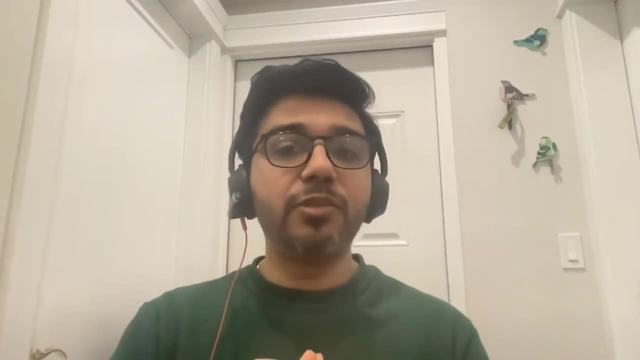 I have got very good starts, So TopMet has selected me to featured me on Times Square- Amazing Congratulations. So yes, coming to the mock. Usually what happens whenever I ask somebody to talk about your framework or topic? what happens? 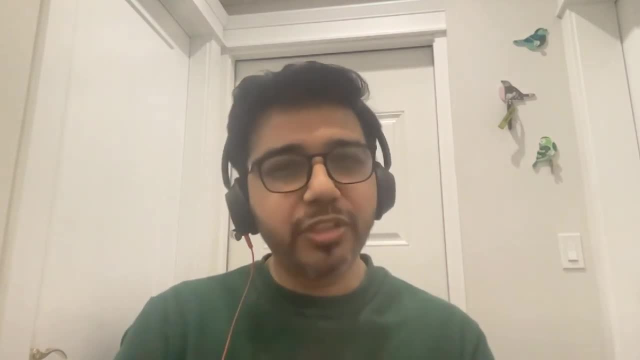 So yes, coming to the mock, Usually what happens whenever I ask somebody to talk about your framework or talk about where you have used encapsulation or maybe overriding in your project, they always give very generic answer, And from that it would be easy to figure out that this person has not used it in real project, rather than he has learned it from YouTube or Udemy. 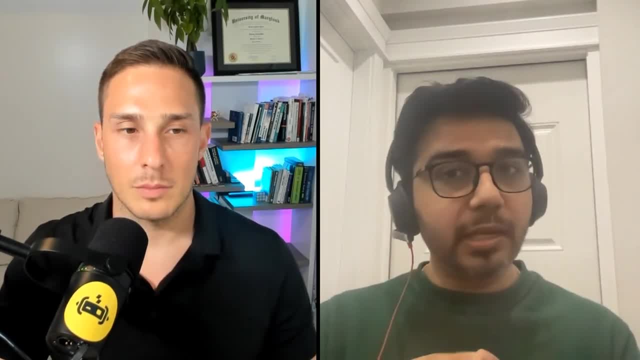 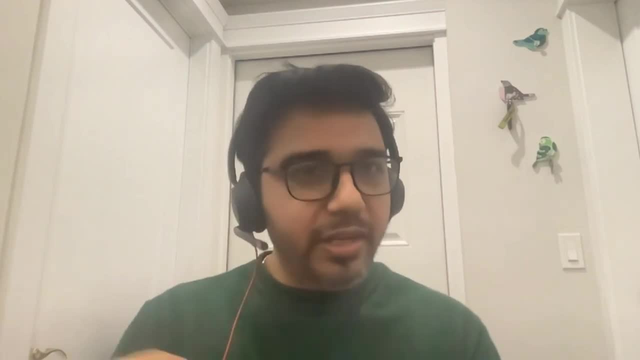 And you will be stunned that if you ask ten people the same question, eight people will give you the exact same example because they have learned from same video. I'm not saying there is anything wrong in it, But just imagine you are hiring somebody. 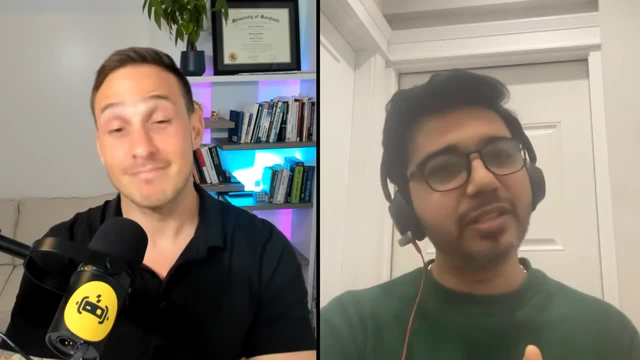 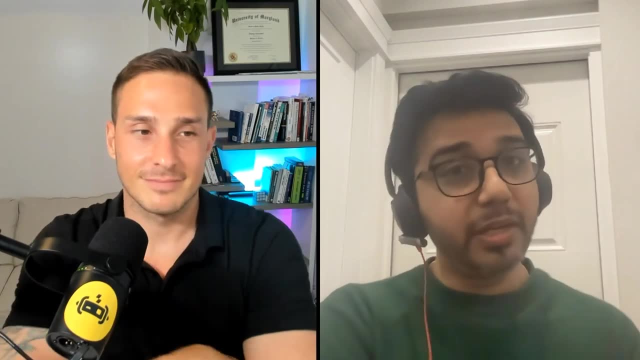 Who is just focused on video and thinking that, okay, this is the only source of truth. There is no harm in watching videos. Do watch videos, Learn from it, But do a little bit of self-exploration. Try to implement in your project. 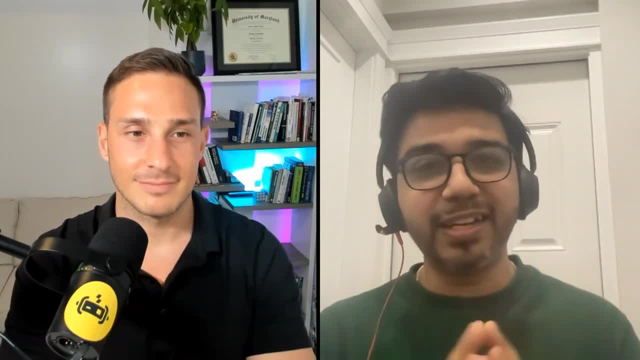 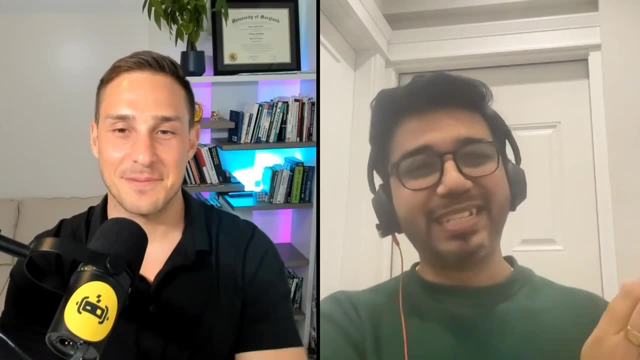 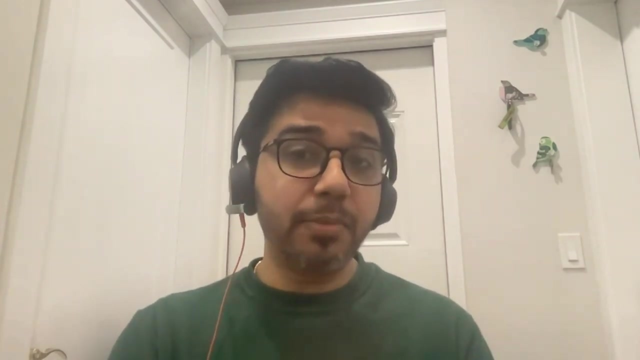 And give an example from your project: Don't give generic cat animal, Don't give cat dog animal, Because we all know that it's coming from one specific website or one specific video. Second thing: whenever I ask some coding question, I feel many a time a person is asking a question. 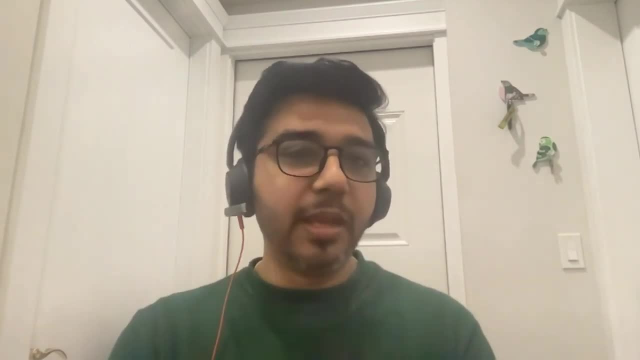 And that person is able to answer, But he is too much scared And the reason behind it is he has never written it on ID. He is just learning it, watching videos, looking into the code. He has not done it. And if he has done it, he has just copy-pasted the code and executed it. 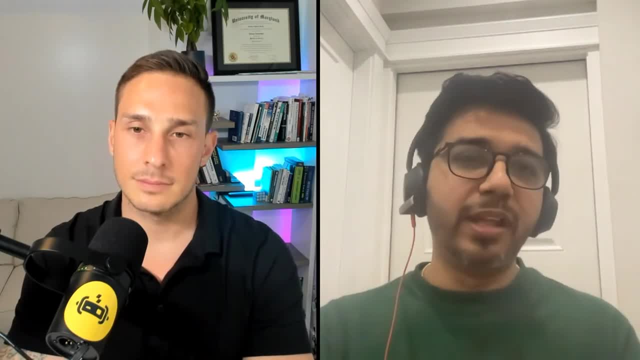 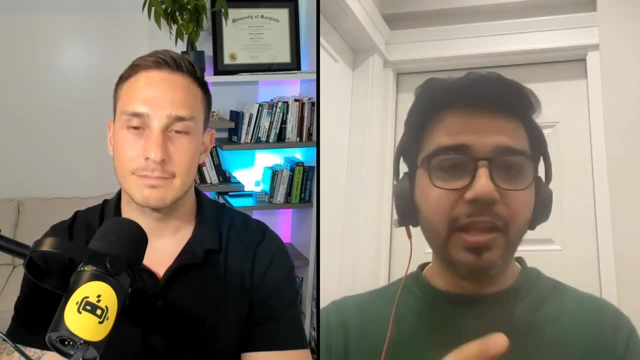 Trust me, folks, it will not give you confidence. Write it of your own. I would suggest don't even accept those compile time error from ID. Try to fix of your own first that what could be the issue over here. Trust me, it will help you to grow how you write code. 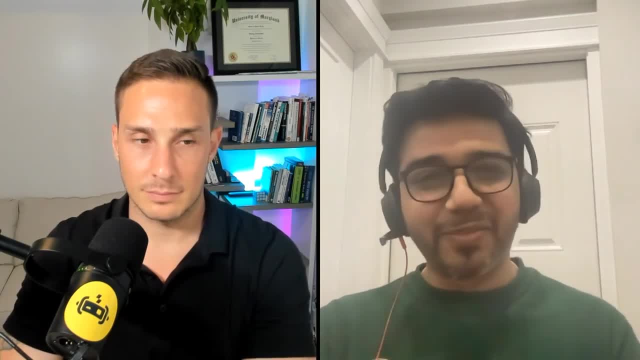 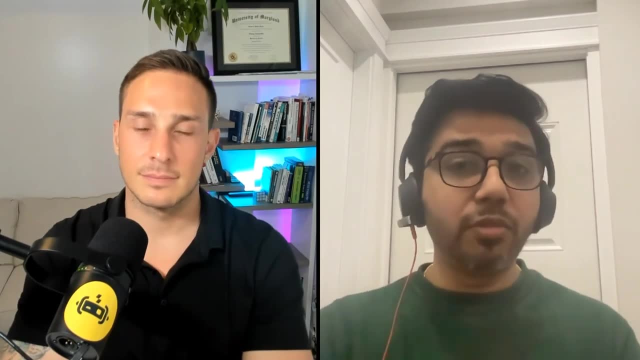 If you always keep on, just move your cursor and accept, you will miss a lot of things. Try to fix of your own that what could be the compilation error, And those things will help you to write code during interview. It will give you confidence. 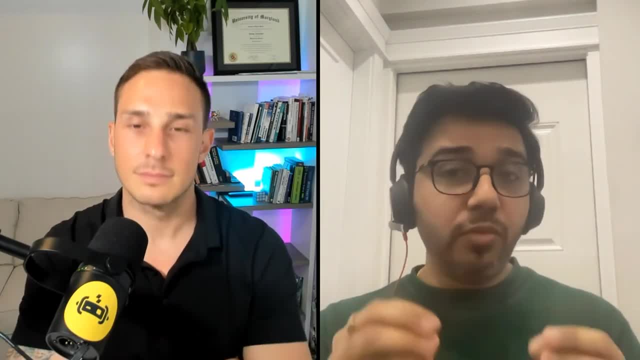 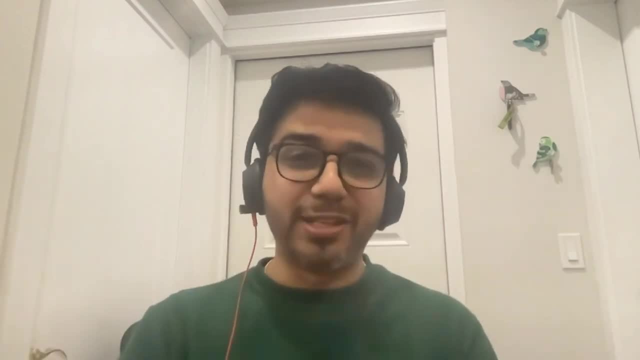 And with that I will add just one more small thing: Do follow coding standards when you go for interviews. Don't just write for i less than equal to 0 i plus Use advanced for loop. Don't leave the catch as it is. 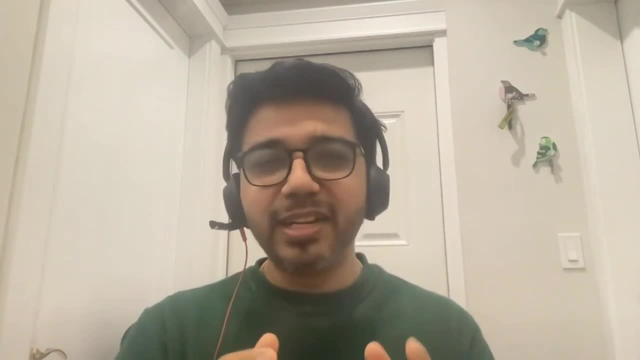 Give it a throw, or give a proper logging Something. give in the catch, right. I have seen many times they are leaving catch blank. No, don't do that. It's a very bad practice, right? Don't throw generic exceptions. 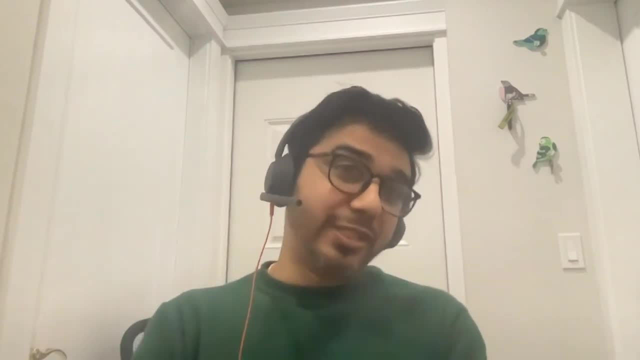 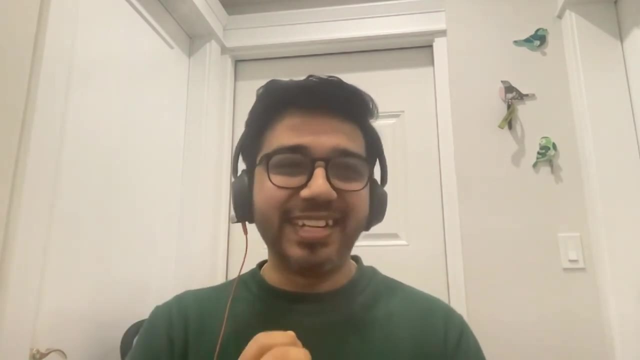 If you are throwing something, give a specific exception, null pointer exception. So those things I do look when I take interview that what kind of coder he is. From that you can judge. okay, this guy is a smart coder or he is just copy-pasting always. 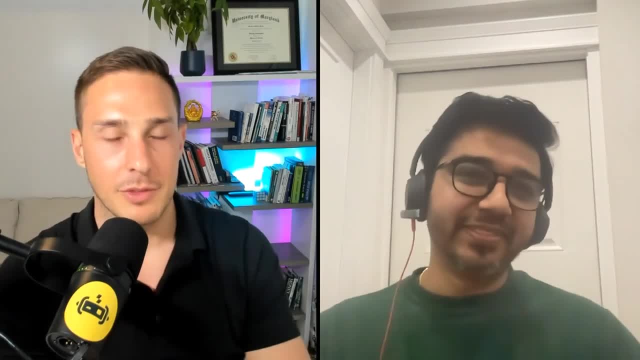 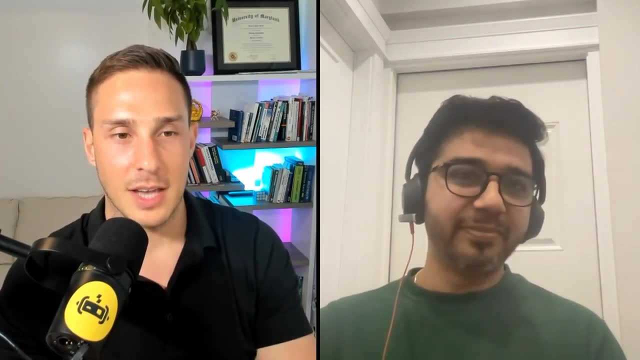 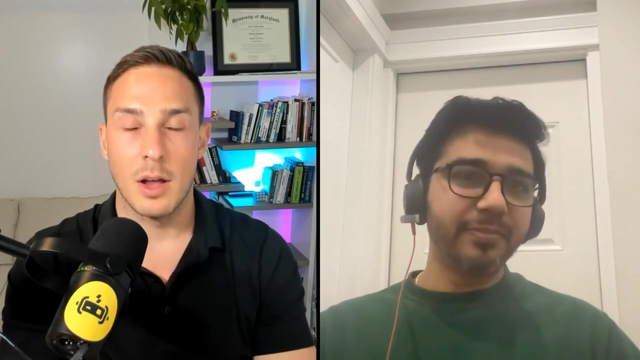 Amazing. Yeah, those are really cool examples that you gave. I love the example of the first one that you gave, The generic answer that I totally agree with. everything you said makes sense. And then it also made me think from an interviewer perspective and a company perspective, where when we are interviewing people, we are trying to find the best candidate. 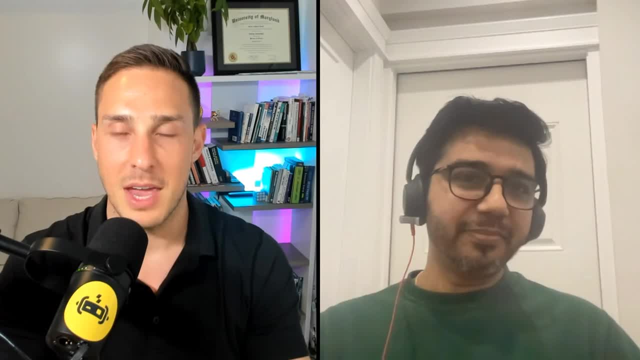 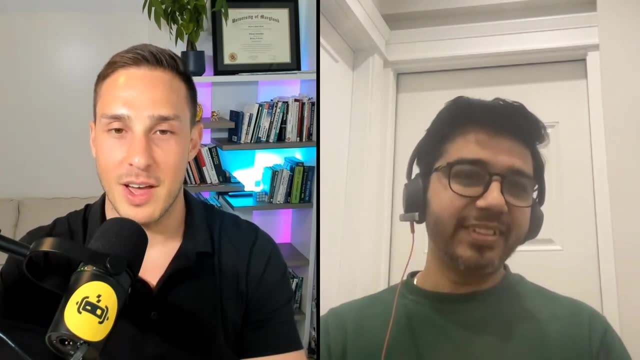 And if all the candidates- as you said, 8 out of 10 people- will give the same answer? those candidates don't stand out in any way. They are the same as the other people that came before them. And so then the one or two people. 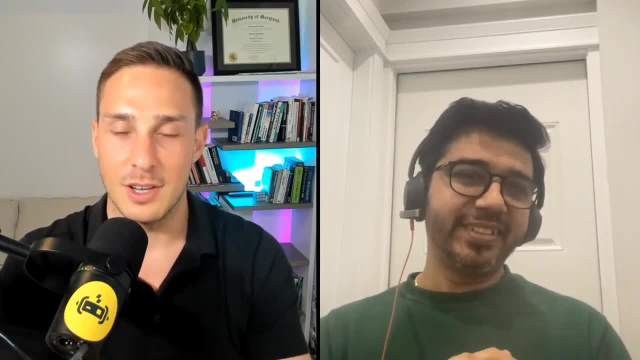 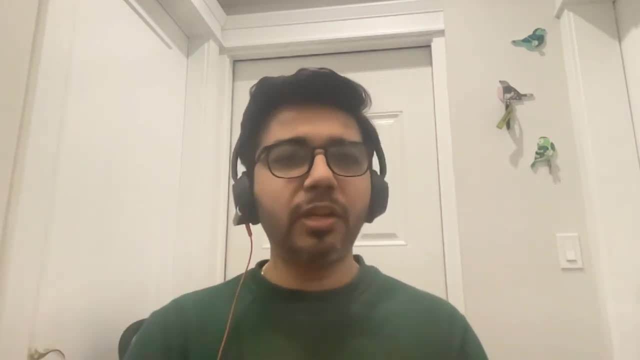 That give a different answer. now they're standing out in the interviewer's eyes right, Exactly, And we want them to grow right. For example, let's take example of any company like Amazon, Google. We don't hire folks to keep on struggling in our project. 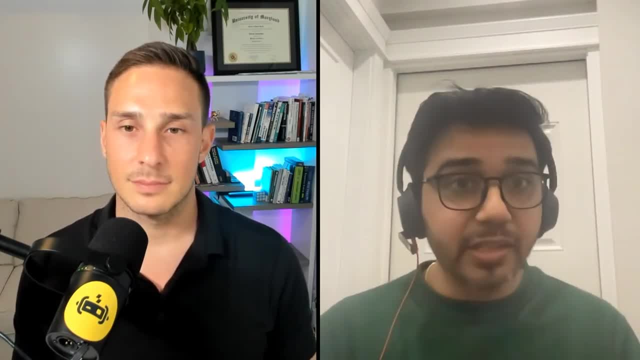 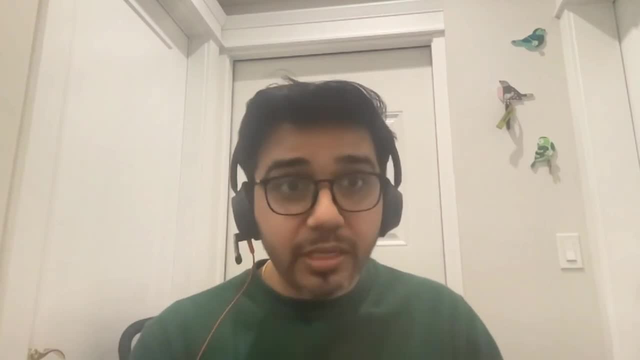 We don't want that. We want whoever we are hiring they will excel in their position And it's not like they are not good for us. They are maybe very good for us, But as of now, what we are kind of looking for in a person that is not mapping with the skills right. 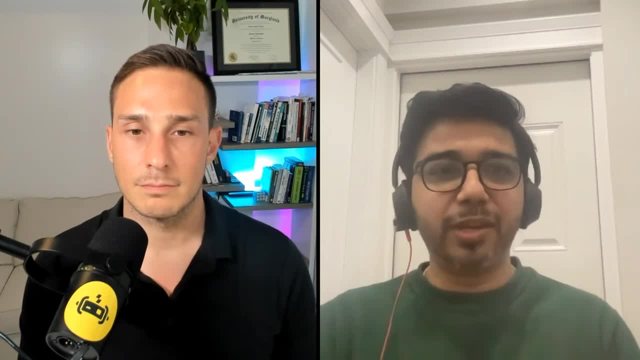 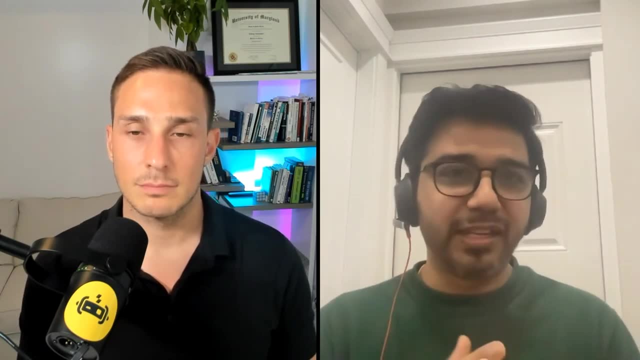 So I'm saying that people may feel: okay, It's like we are not good. You folks are really good, Everybody who is trying. they are good Folks who are not trying. maybe they need to do something extra, But if you are watching videos, do that. 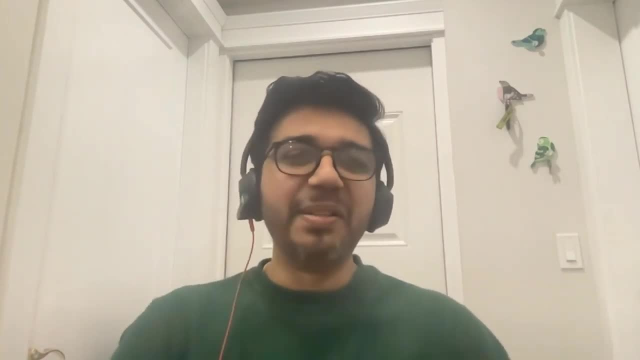 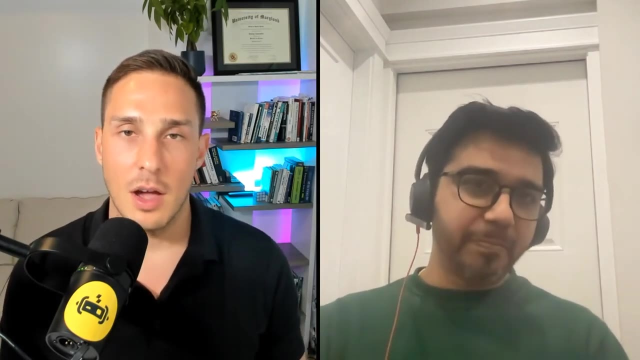 Don't stop doing it. I'm not saying don't watch videos and learn, But, yeah, do a little bit of exploration, right? Yeah, that makes total sense. Another question I have for you, Sid, is: what qualities does Amazon look for as the candidates? 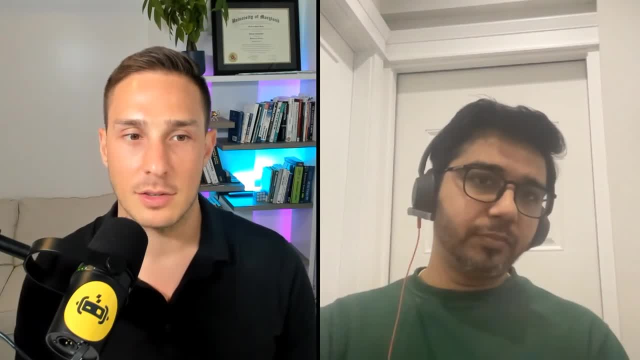 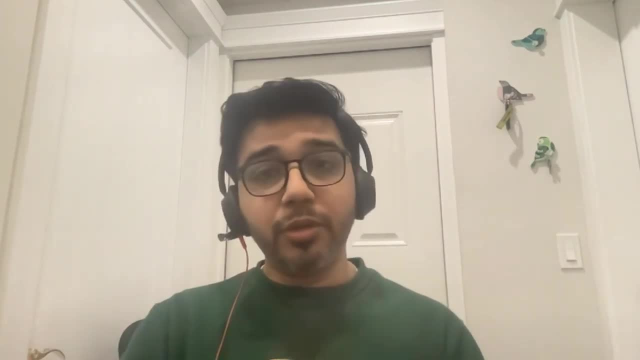 And how can other aspiring, as the candidates, align themselves with these expectations? First, you should have knowledge in design patterns. It should not be like you only know Selenium, Rest Assured. APMU will make sense, okay. So first thing, design patterns, architecture. 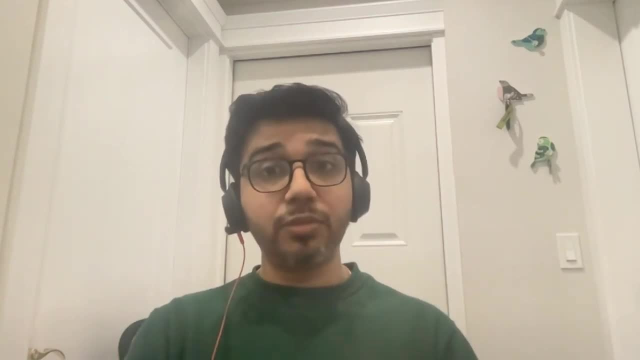 That's why I cover this in my courses. In my courses, I always ask my students that before you jump into Rest Assured, understand architectures. Understand how microservice works, how SOA works, how event-driven works. Understand it. If you don't understand, you cannot write integration tests properly. 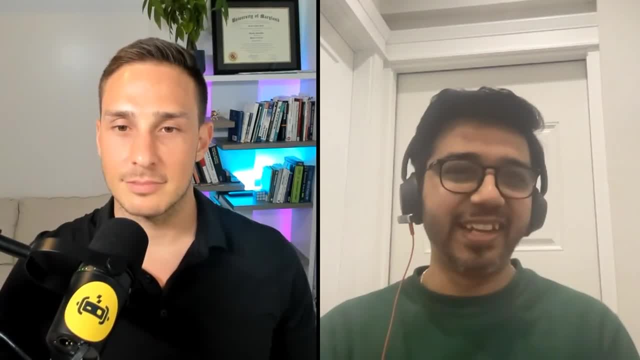 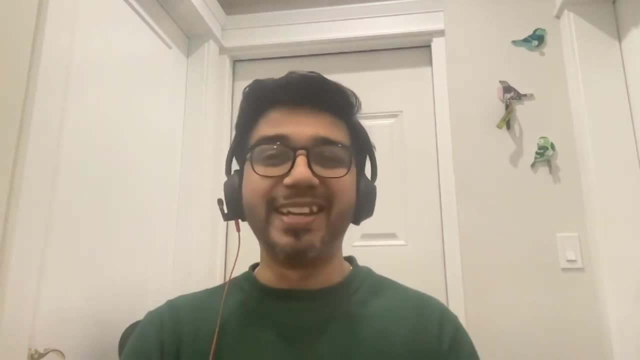 If you don't understand architecture, how you will write integration tests right? So understand architecture and design patterns will make you a good coder, And don't go with only page object model okay, Which is not really even a design pattern anyway. 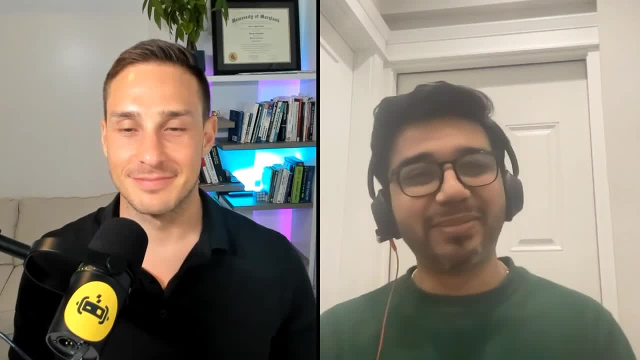 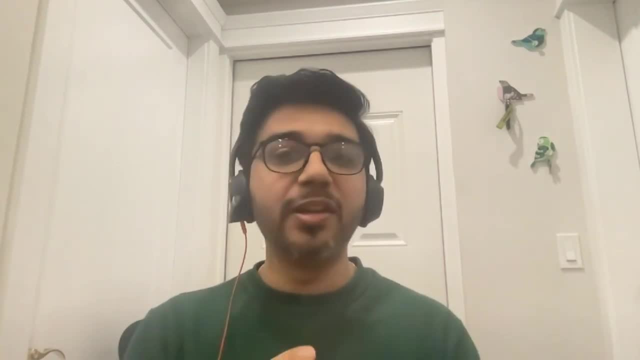 Exactly. So many times I ask folks in interviews. they are saying page object model. I don't want to argue, but I told them: okay, After that, singleton, done Movements apart from these two. If you want me to say, then go for builder pattern. 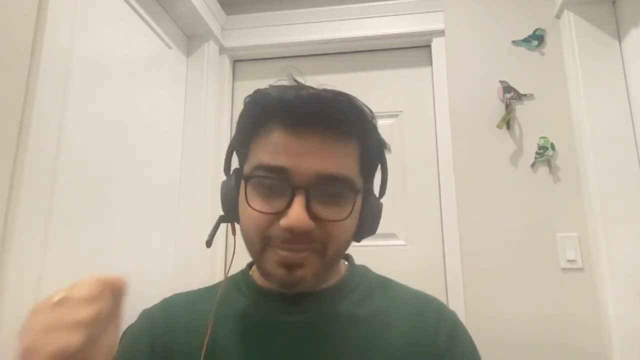 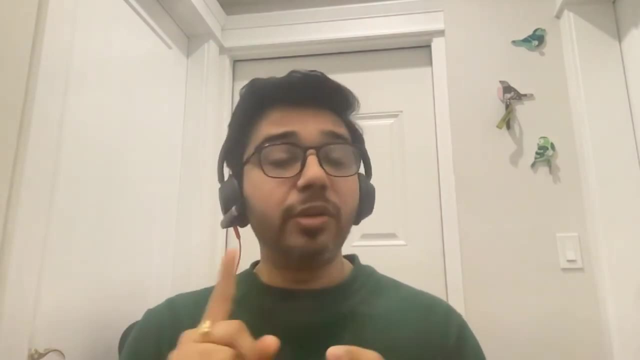 Understand it. We use it a lot. So builder pattern very important. If you want to explore extra strategy and decorative are good, But builder pattern very important. Second thing: coding standards and optimization. Write optimized code. have good coding standards. 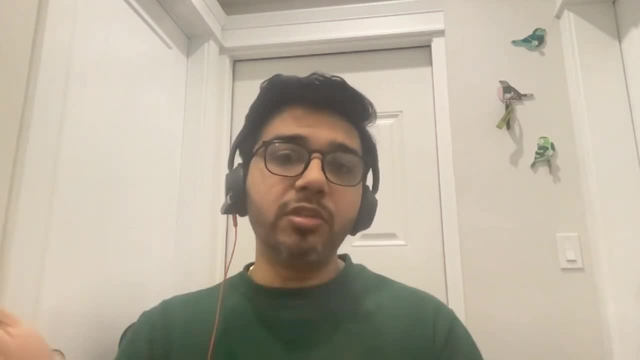 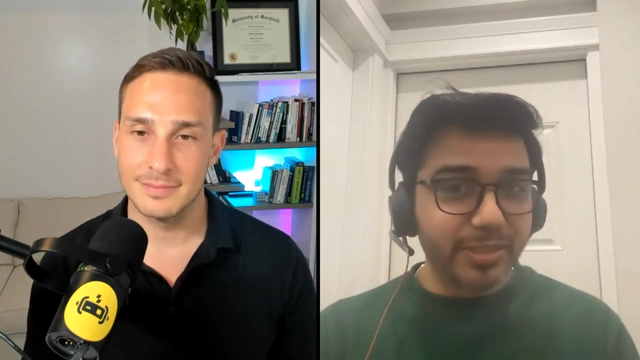 Third, don't learn multiple tools from single automation. For example, I have seen folks who are learning Selenium Cypress Playwright. The problem is, all are web automation Rather than Selenium Cypress Playwright. That's why in my courses I always ask folks: don't do that. 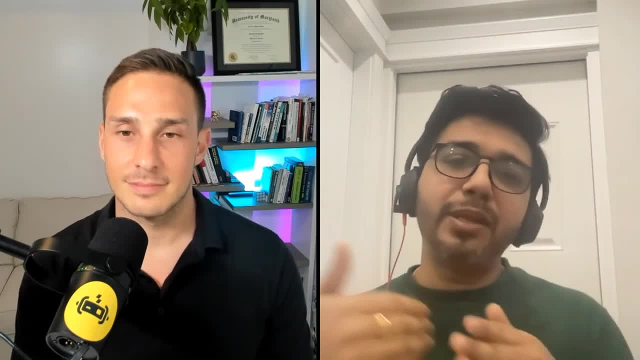 It's a harmful thing. What you should learn: Selenium APM Rest Assured Because you are kind of Learning all aspects of automation, right Web API, mobile. So instead of spending time in Cypress Playwright, spend time in these two things. 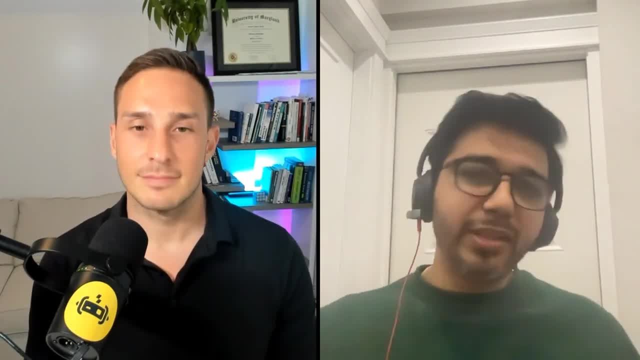 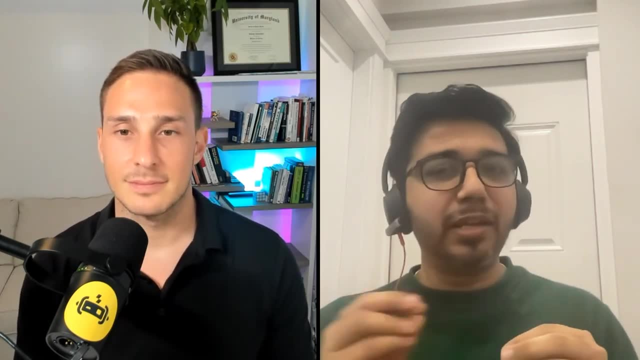 And trust me, interviewer knows If you say I have skills in Playwright, they will not give you extra point if you have Selenium and Playwright, Because still you are in web automation. I used to give extra points to explore other aspects. 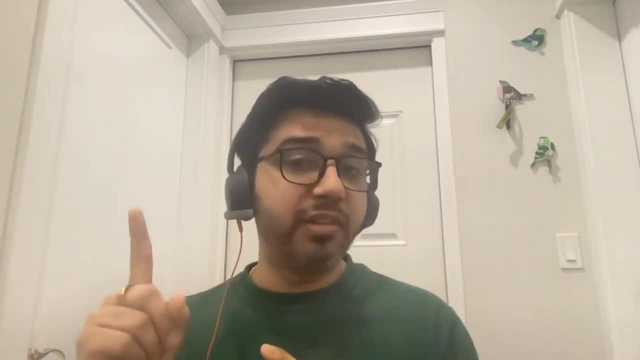 Fourth, have proper understanding of Maven Jenkins Git. You cannot sustain without build tool, CICT and source code repository. It's a lot. You cannot build repository in any project. And the last one: explore cloud fundamentals. It will help you a long way. Because, as an estate, you need to take care, Because many team doesn't have DevOps, They don't have SRE, So you need to take care of things. You need to fix pipelines, You need to fix severity to tickets. You need to take care of your pipelines how it can be healthy for a longer period of time. 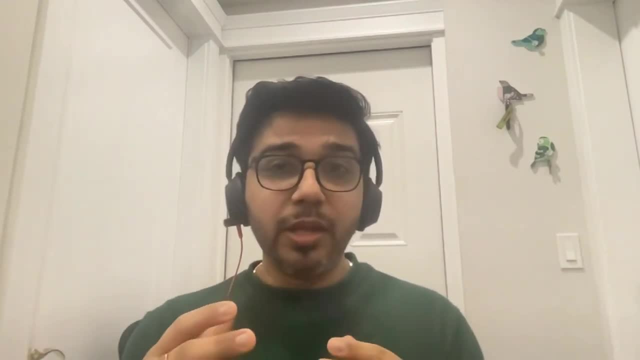 How you can implement different automation technique to reduce the operational cost by reducing number of severity to tickets. So you have to think in that perspective. So cloud exposure is, I feel I'm not saying it is mandatory, but good to have, It's definitely good to have. 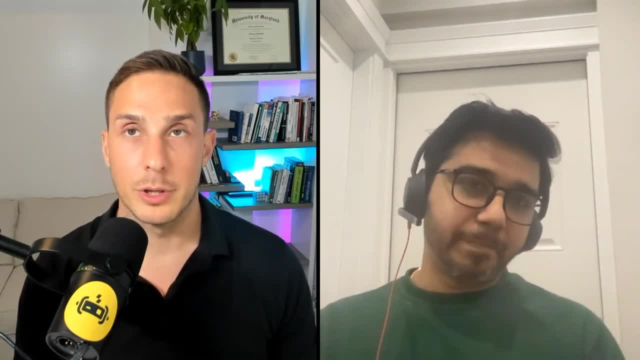 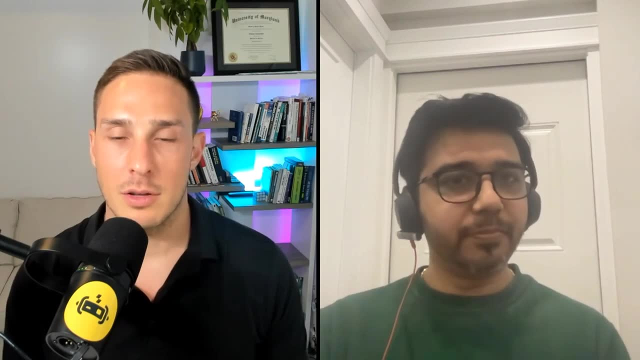 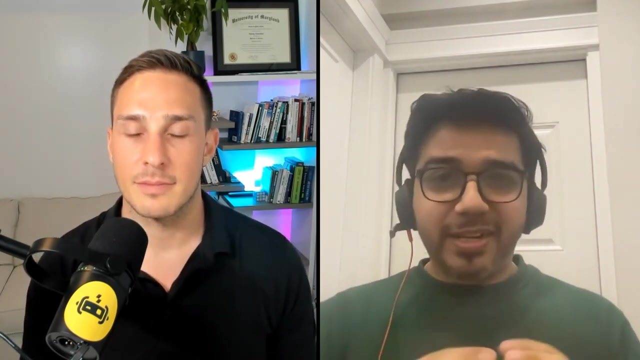 Really great advice. So are you building and maintaining your own CI pipelines? Yes, Are you also responsible for monitoring the pipeline and monitoring the state of the application and production? So we have kind of automated the centralization. So monitoring, notification, everything is properly automated. 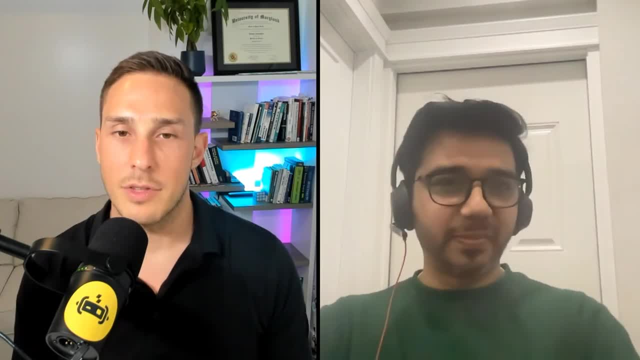 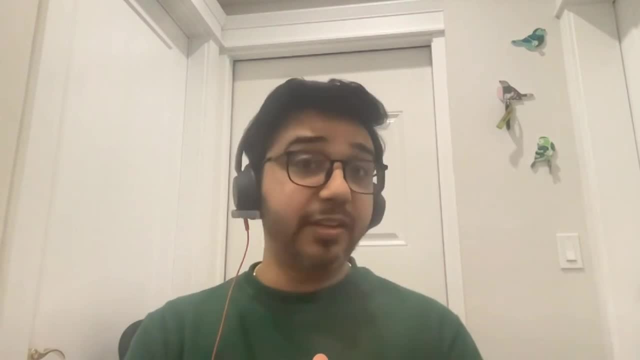 But yes, we do look into it And if there's an outage, are you responsible for triaging it and figuring out what went wrong, and so on. Exactly, RCA is a very important role of an SDET. You have to do root cause analysis. 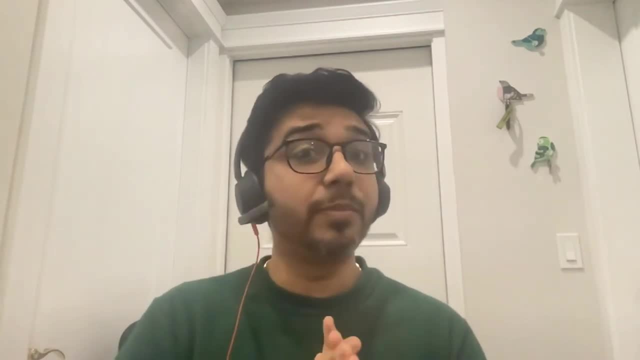 You're an SDET, right. You have to figure out what could be the problem and how we can avoid it happening next time. That is the most important aspect of SDET: You have to figure out a process so that it will not happen again. 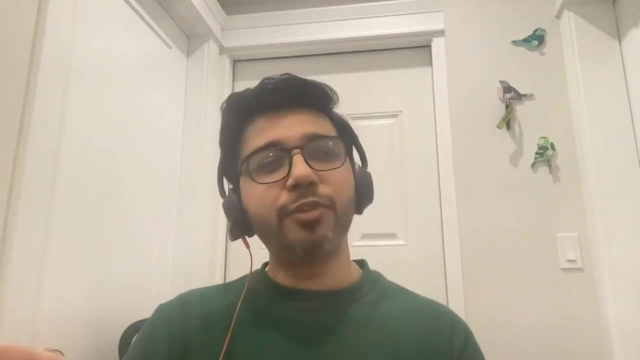 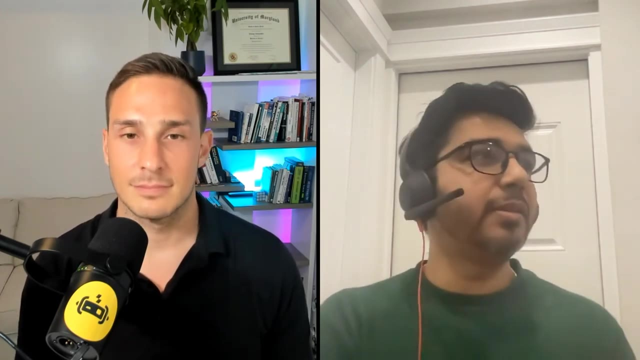 You have to figure it out. If you are fixing the same ticket again and again, and if you are an SDET in your team, then he is somehow not doing his job properly. You should not wait for somebody to come and say, okay, why it is happening again and again. you do something. 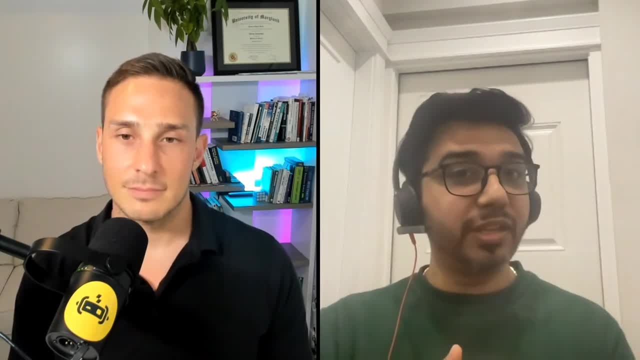 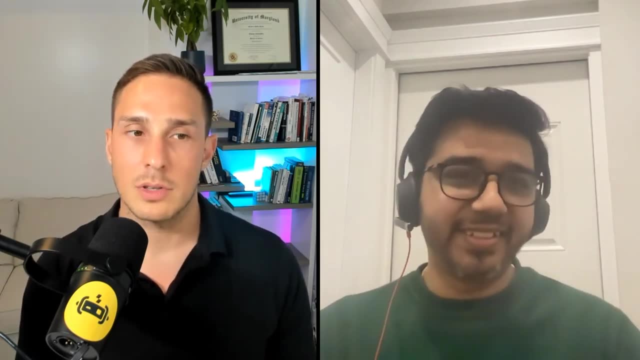 He should come up on his own. Okay, this is happening again and again. We are spending two hours for each ticket. We have spent around 16 hours in this month, So let's do something for it, right? Yeah, Great points. 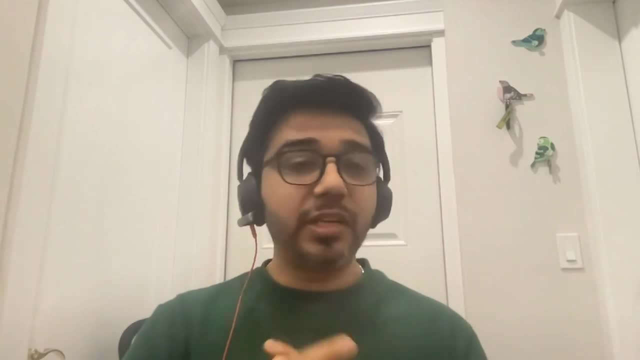 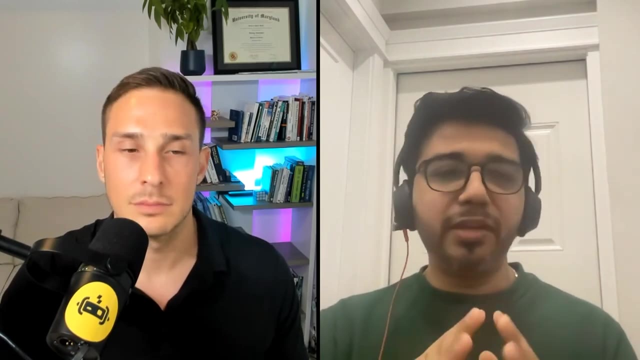 And do you also write unit tests? Yes, For example, the tool we design, the services we design, the package we design- We have to write unit tests of our own, And that is kind of very much expected from an SDET. 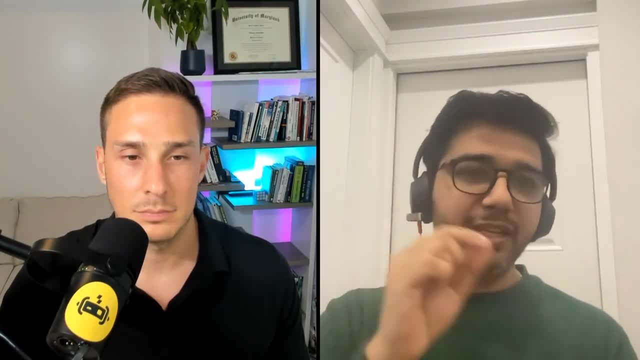 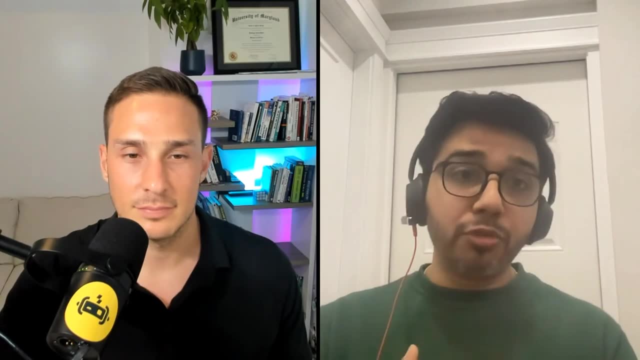 See, SDET starts with SDE. So the common thing: SDE is there right. TE is only there so that you have expertise in testing, so that you can come up with a solution which will help QAs. That is one aspect they are looking for. 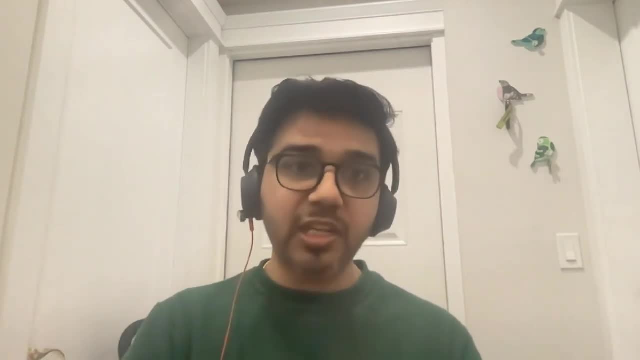 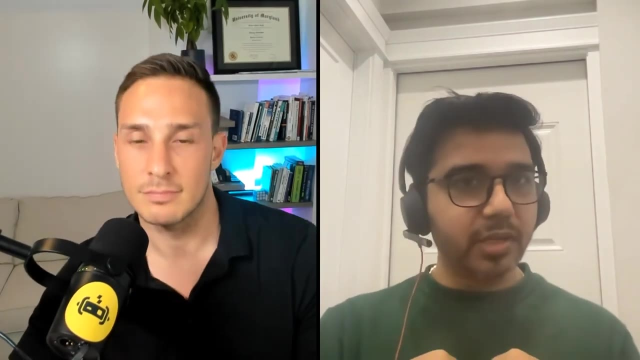 And it's not like you will not do SDE's task. You will do SDE's task, but you are not doing something for end user. So SDE is designed something for end user, right For customer. You are not doing something for customer directly. 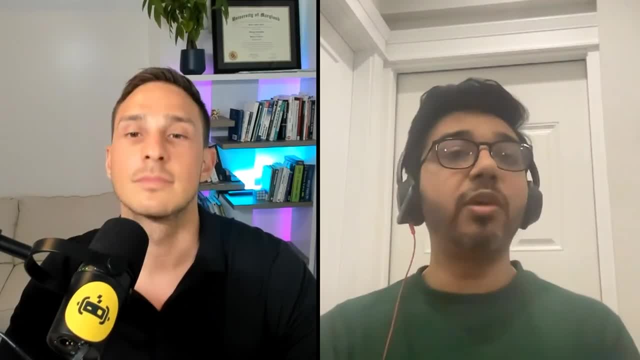 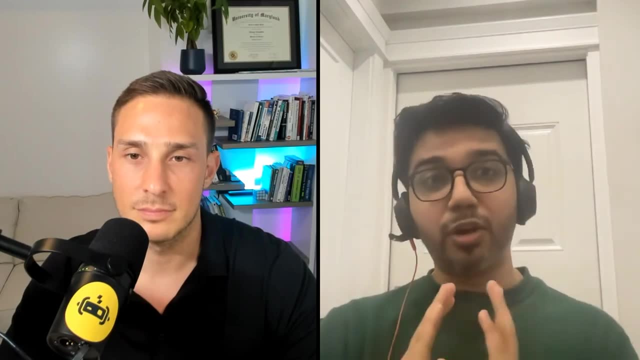 You are doing something for SDE's and QAs. You are helping them so that they can do their job efficiently And at the end of the day, the customer will get profited out of it, But you are not catering anything to customers directly. 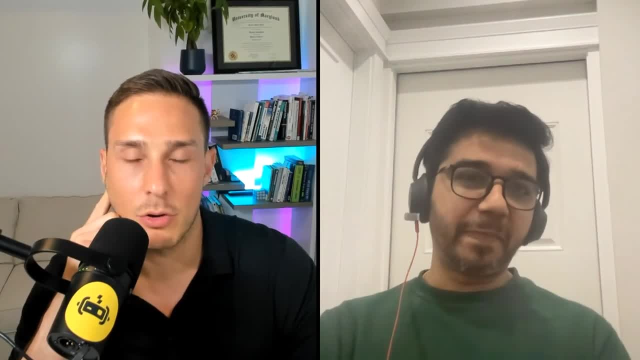 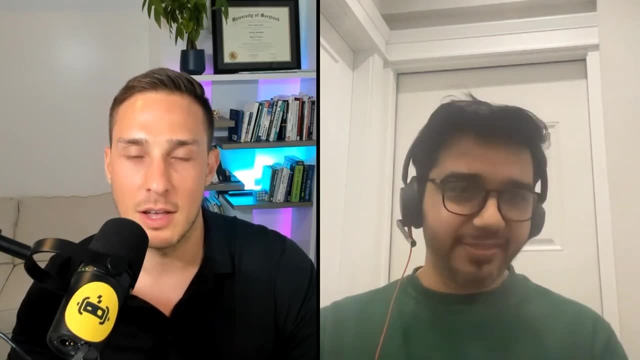 That is an important point to notice. right. That makes total sense. Basically, your customers are internal engineers, As you said, QAs and software engineers. they're your customers And you're delivering software. You're delivering software products for them. 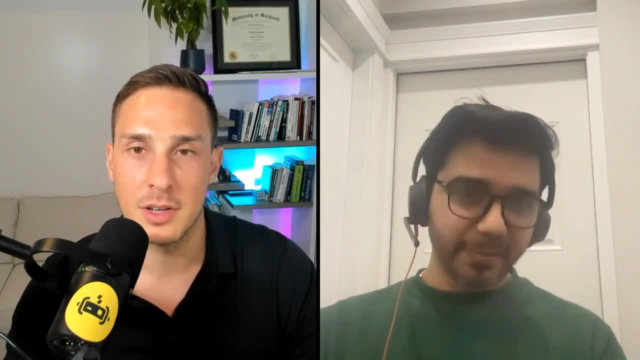 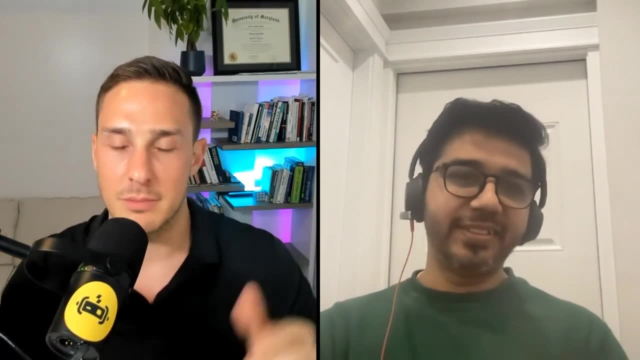 And, of course, if you're delivering software products, you have to follow software development best practices, Even though it's just automation code. but it is Exactly So. if you're writing a package, if you're creating a library, you have to set up your own pipeline. 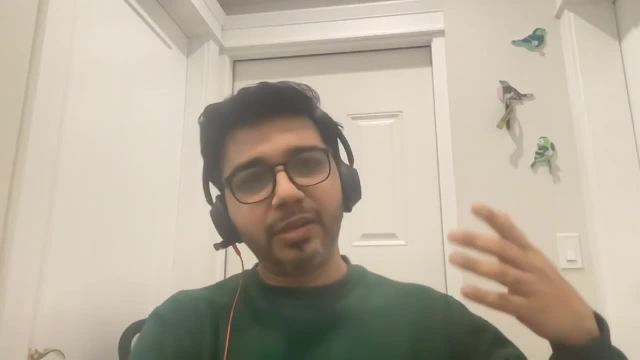 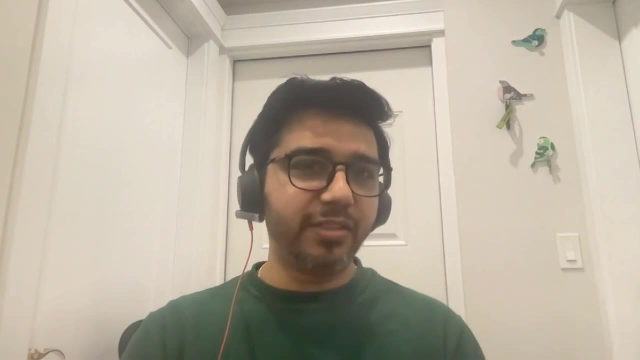 You have to set up everything right. That happens. You cannot do it with one package. You may be dealing with four to five packages. You need to create HLD LLD. We only do the HLD LLD, So everything you need to do like a software developer. 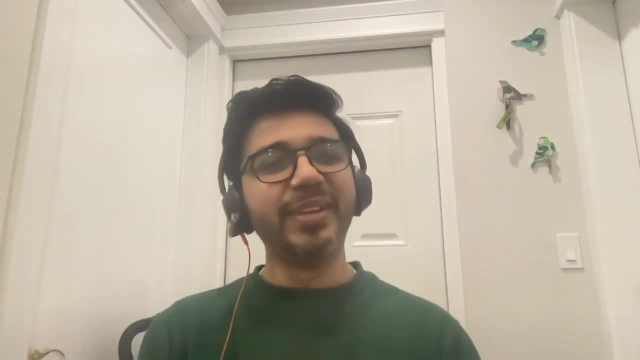 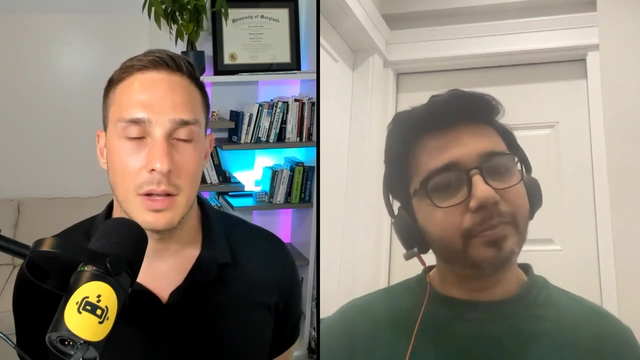 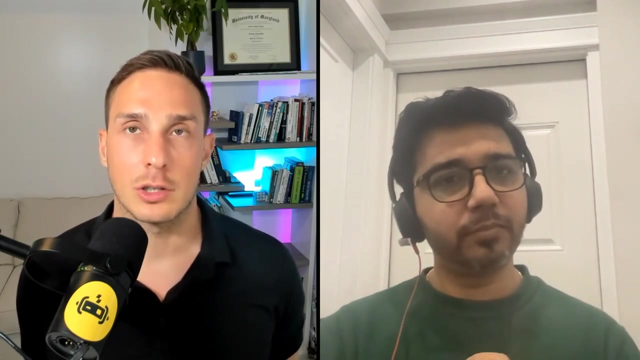 But the only thing is you're not catering to customer, You're catering to, basically, SDEs and QAs. Yeah, that makes sense. Sid, if someone wanted to become like a software development engineer and test at Amazon, how would you recommend for them to start learning, and which skill set should they prepare for that career? 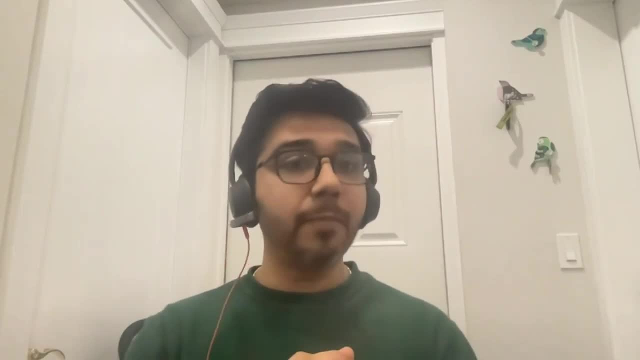 So the five things that I told they need to focus on that one for sure. Okay, They need to pick one tool, one library framework or tool on each web. all the three sections of automation, as I told, and they have to make sure that they spend a lot of time in writing coding. 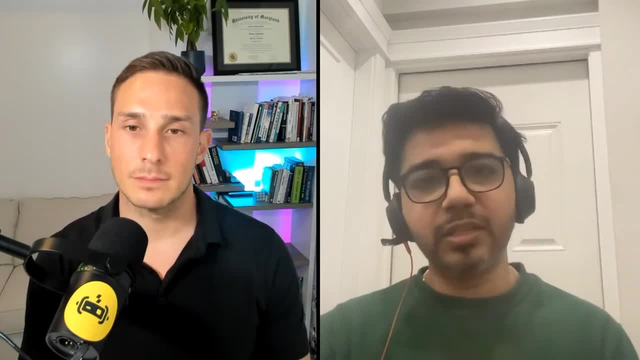 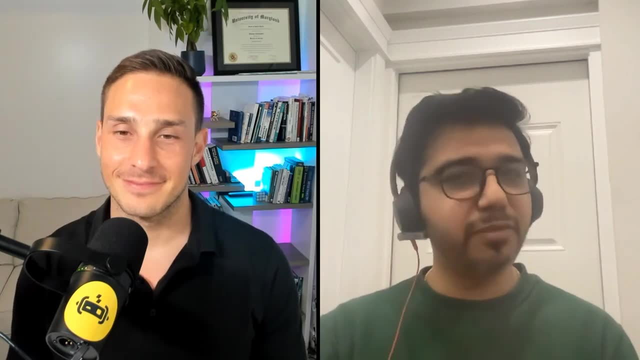 Okay, Why? Because there is no shortcut in it, There is nothing. If you watch a hundred hours of videos in coding, the value addition would be hardly one to two hours, Trust me. But if you write one hour of coding, the value addition is one hour. 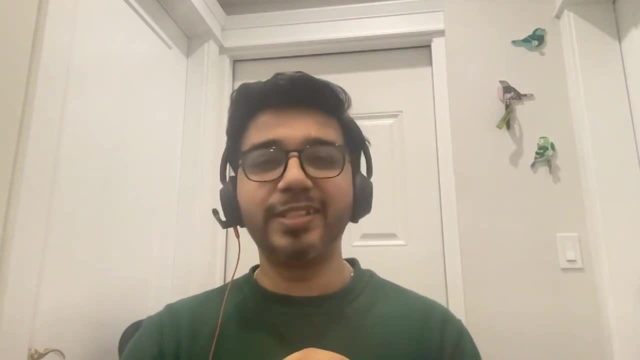 So from that you can imagine what you need to do. So just go to your VSTudio Or go to your IntelliJ, Start writing code And there is nothing like: okay, this code I have practiced. It will not help me. 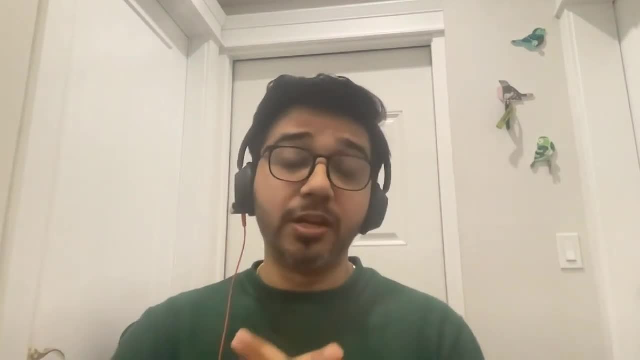 Trust me, It will help you Because it is something which is building in yourself automatically. When you write a lot of code, it will automatically build in yourself, Right? People say, hey, I will come, It will write your code. 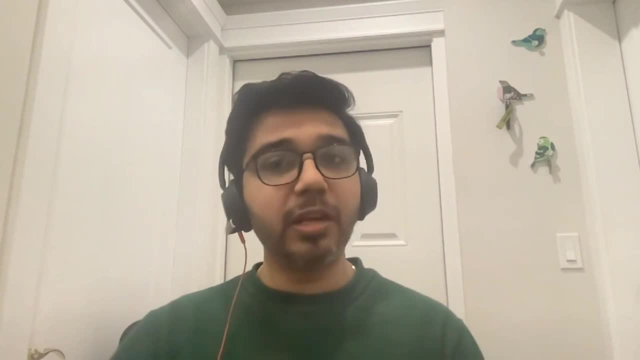 That's fine, But what code to write? Who will tell this to AI? And if you don't know coding, how you will tell to AI to write proper code? As an engineer, irrespective of SDT, SD and QAE, don't avoid programming. 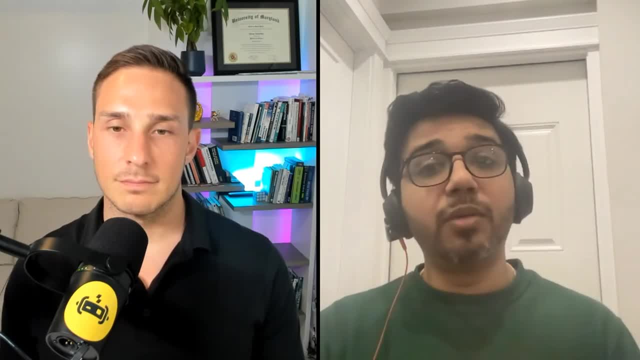 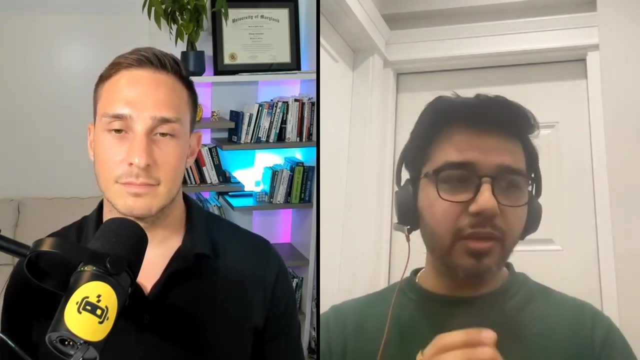 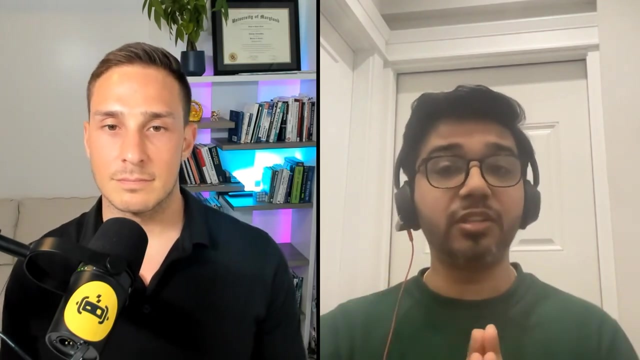 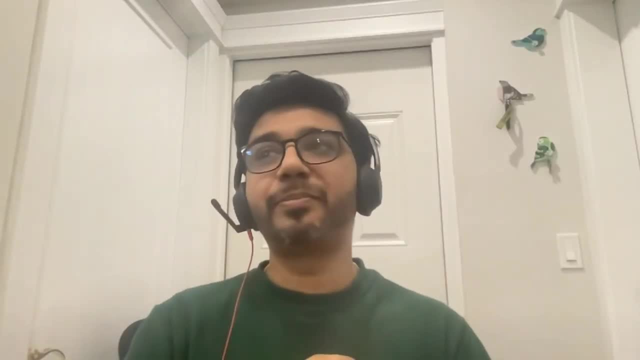 There is a lot of talk like DA Salgo and everything. Folks don't jump into DA Salgo. I have seen folks who are learning DA Salgo But they don't know much about ArrayList and Map. This is a deadly situation. 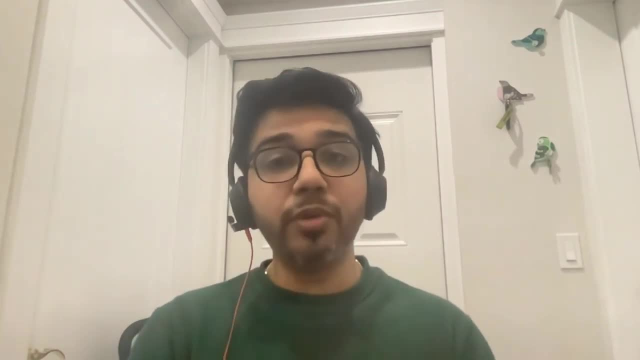 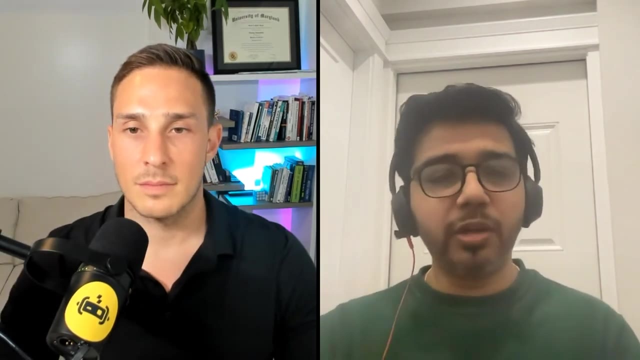 Okay, folks, Don't jump into DA Salgo. unless you are a pro in String, ArrayList, Map Exception Handling, Be a pro in these five things Than jump into DA Salgo, Or else you will feel lost. You will leave. 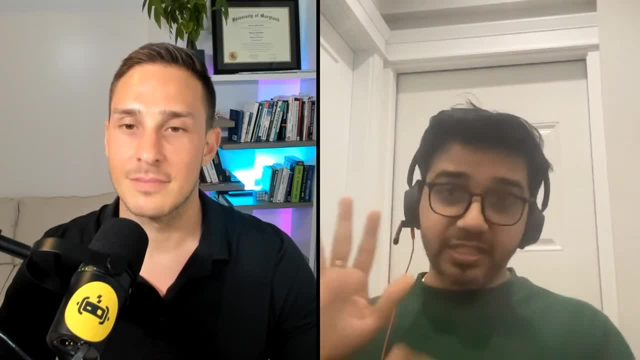 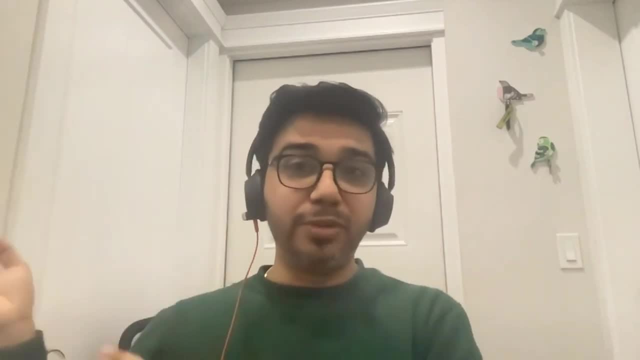 The videos or whatever you are learning for DSL go halfway. So first excel in these five things, Ivan, just give me a quick path. Then learn sorting and searching, Then time and space complexity. Don't jump into tree graph directly again, okay. 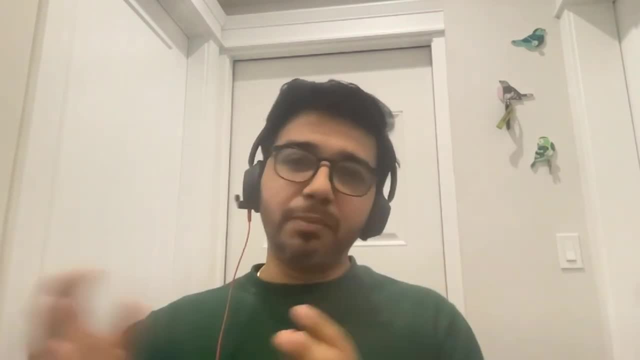 So there is a sequence to learn: If you skip ArrayListMap, jump into DSL, you will feel lost. So ArrayListMap, then sorting, searching, then time and space complexity. Sorting, searching, time and space complexity should go hand in hand, okay. 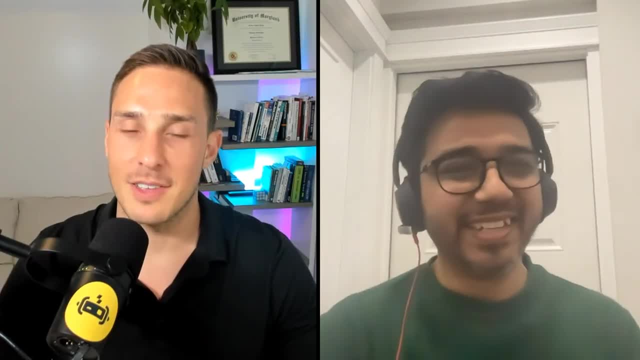 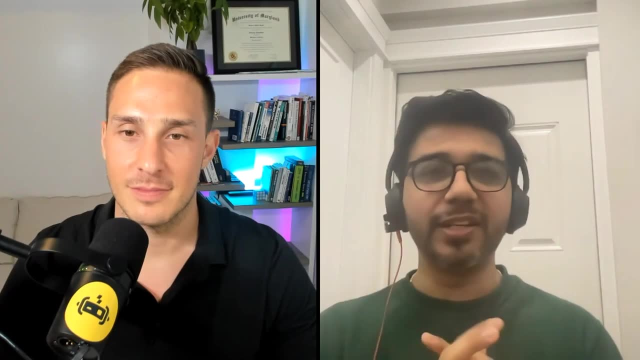 Because there are a lot of correlation between them. That was amazing. Do you have some resources You recommend for people? Yes, I do have a very nice SDT course which I put over here. I have covered every aspect of it, okay. 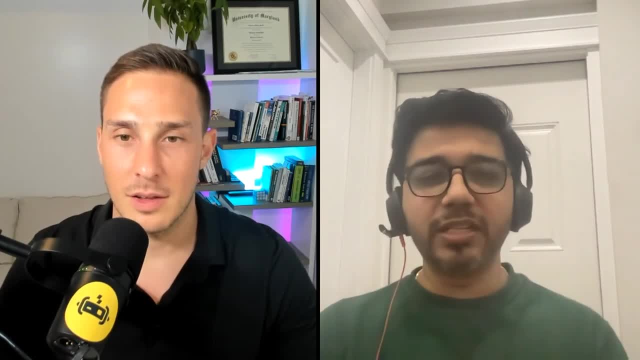 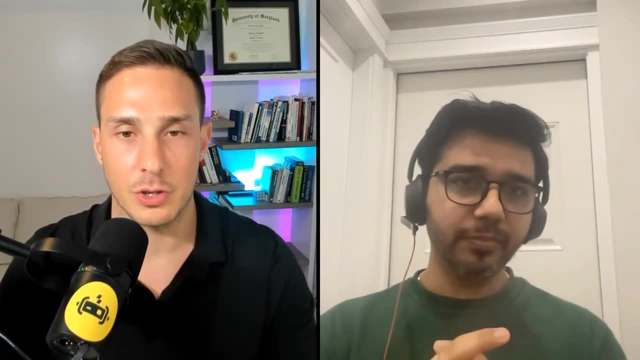 So I guess it will help you folks, Because my students are getting benefited out of it. So you can give it a try and see that how it will help you. If you want to pull that up on the screen and show it, I don't mind, please. 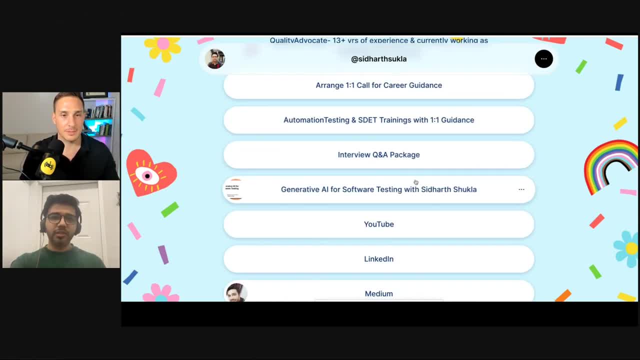 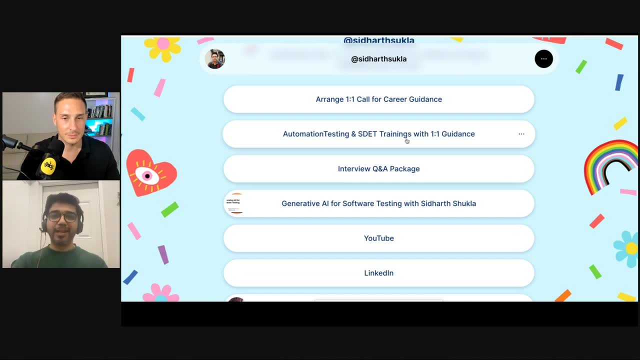 So this is my link tree. If you can see over here, folks, I have everything over here. I have a generative AI session also. You can go and buy it over here. I have created it with a lot of effort, like how you can use Gen AI. 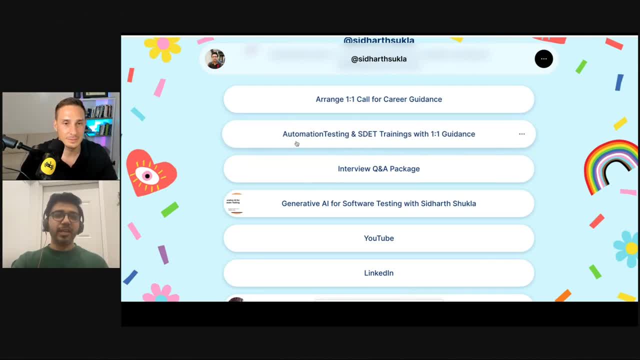 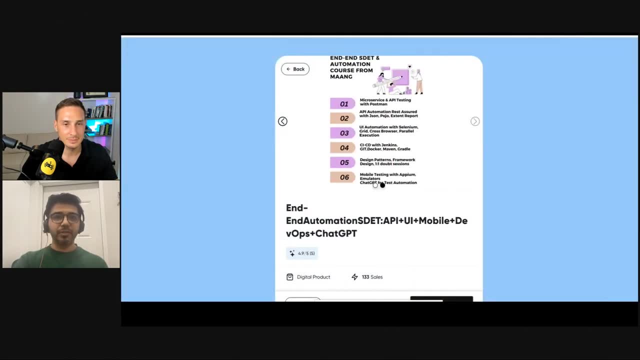 And if you want to talk to me, you can just talk me over here one-to-one call. And if you want trainings- the second option- you can go with automation testing and SDT training with one-to-one guidance. you can post it over here. 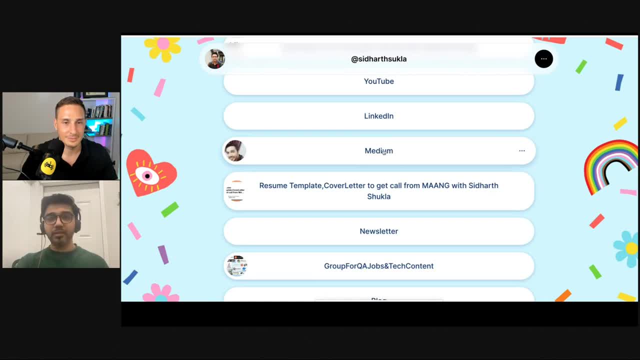 Here is my YouTube, LinkedIn and Medium Medium. you can see a lot of articles right. If you want to access it for free, go for it. And this is my newsletter And it's a very good one, okay. 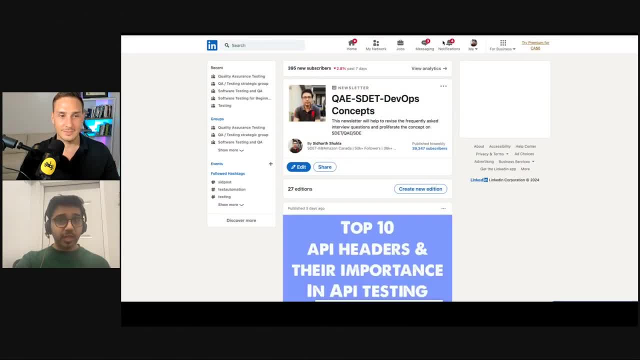 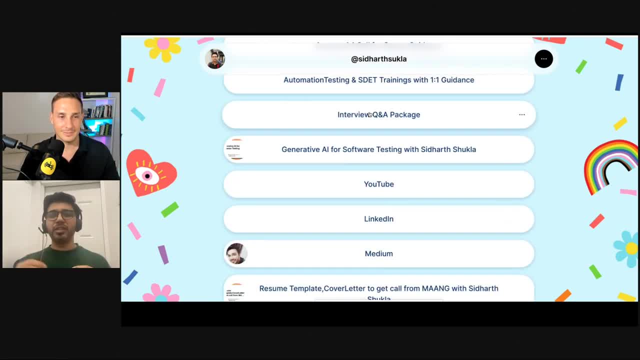 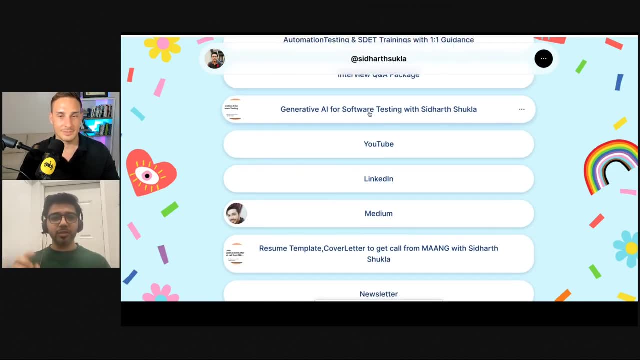 You can just go and read it. And again, if you are just looking for interview question and answer, you can go for it, But don't go for it directly without having your concepts clear, because that's not a good approach, okay. 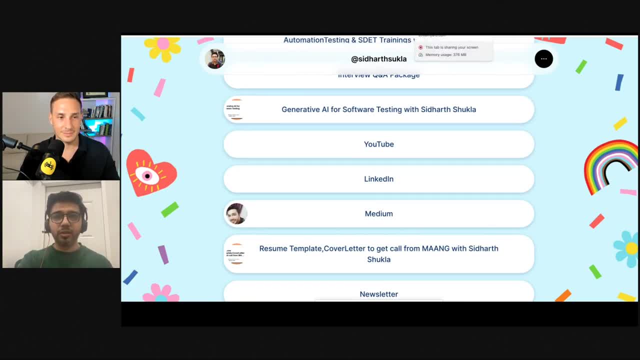 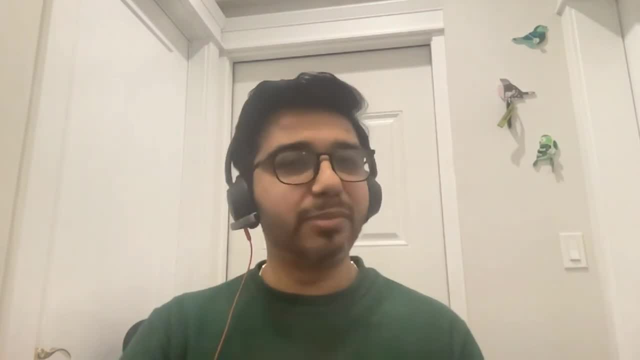 Just going through the interview, question and answer without knowing the concepts. So I don't market it a lot because I don't like folks directly jumping into question and answer and they don't have proper knowledge on the concepts. okay, Don't do that. 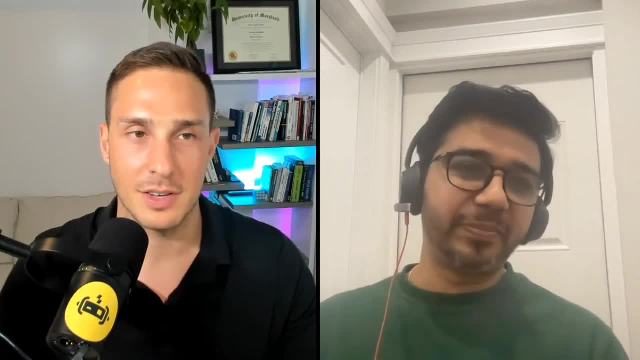 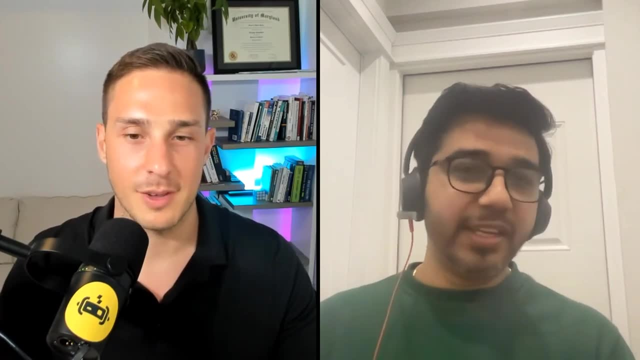 Yeah, absolutely. In that case, then it just becomes Okay summarizing a bunch of Q&A to pass an interview versus actually learning how to do your job. well, right, and the things have changed a lot since last. this JNI has come into picture. it has changed a. 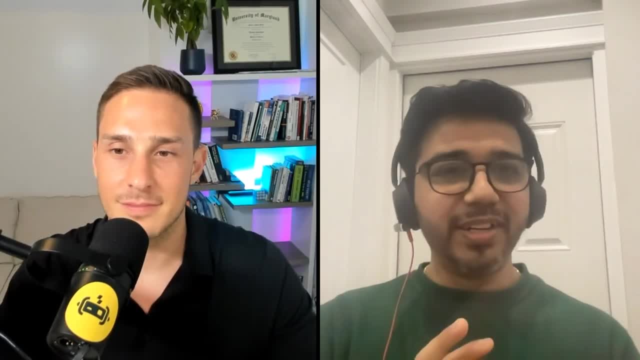 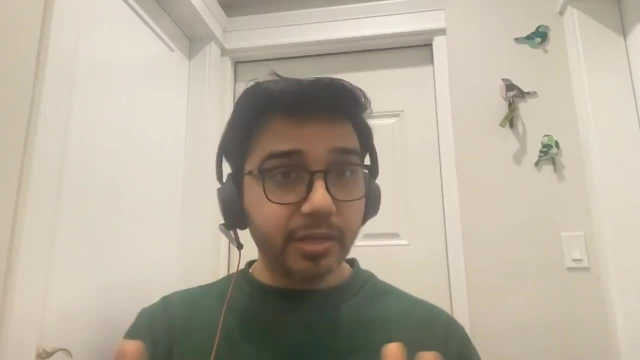 lot people are not satisfied only with true, false, yes, no definition answers, right, because I talk to my students. they are always asking scenario based questions. a lot that has impacted the entire interview. scenarios, right, and how the economic condition is also nowadays. you know about it, right? so two years back situation was different. one point I want to touch on- you mentioned you. 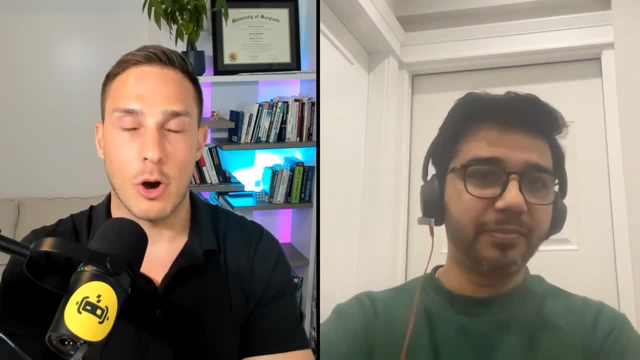 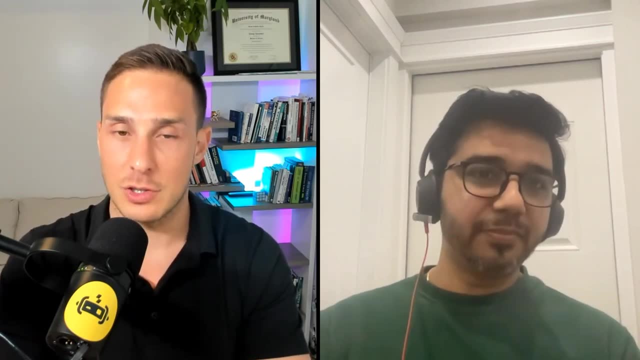 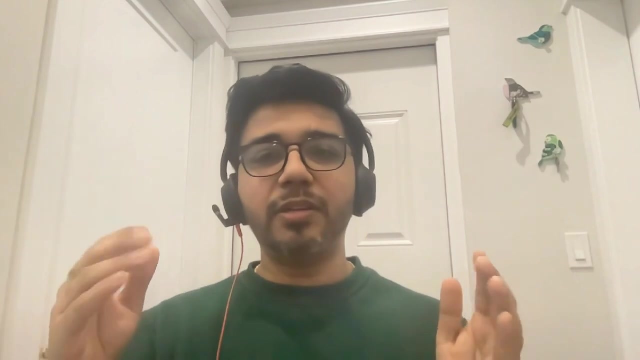 have to excel the things that you mentioned for us to learn, to become an asset at Amazon. if we learn those things well, will we excel, or is that just the bare minimum you will excel. so our focus would not be getting a job in Amazon. our focus is that, whatever I write, I understand. 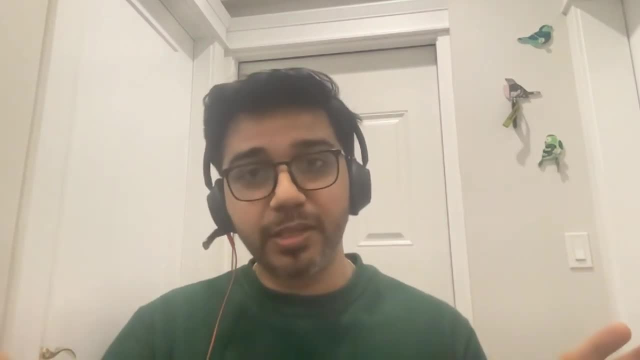 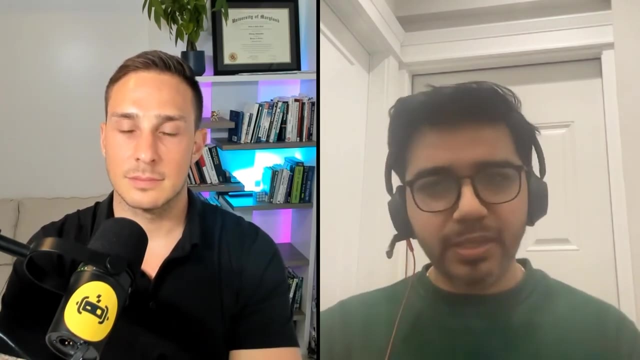 that and I am writing the best code possible by a human being. do that, trust me. companies doesn't matter right at some point of time, but if you are a good cutter, you will be hired at any place. right? you should not be worried, right, if you by some situation, if you get fired or 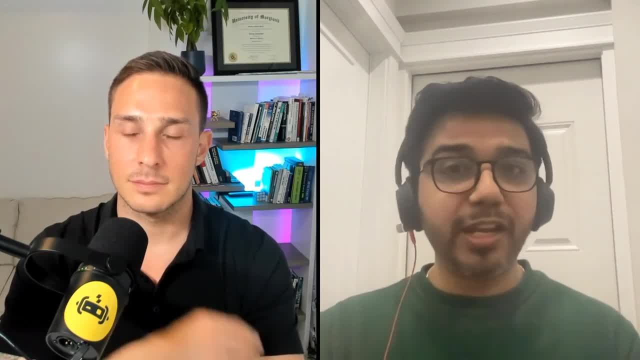 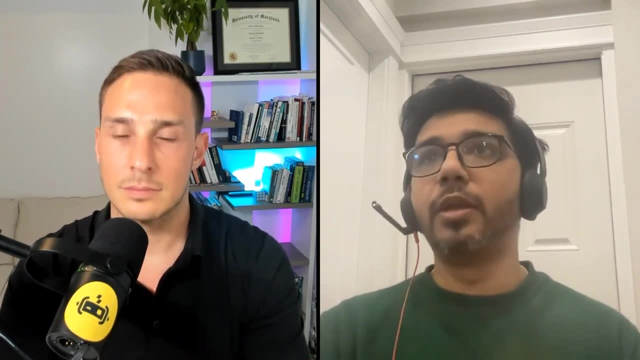 something happened. also, you should not be worried because my student today morning I got this message, Nikolai, I want to share. there is a folk who is in US okay, and he lost his job. he has 60 days to search. one month back he reached out to me and he told that I'm in big trouble right now. 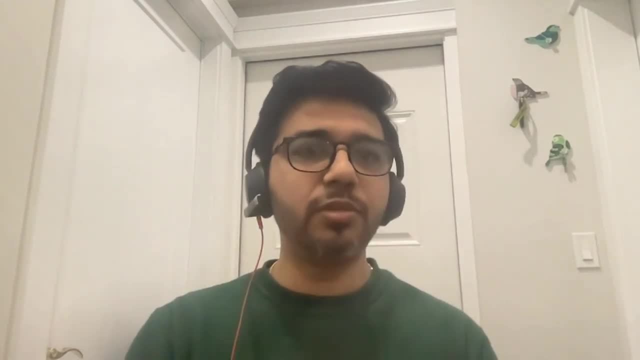 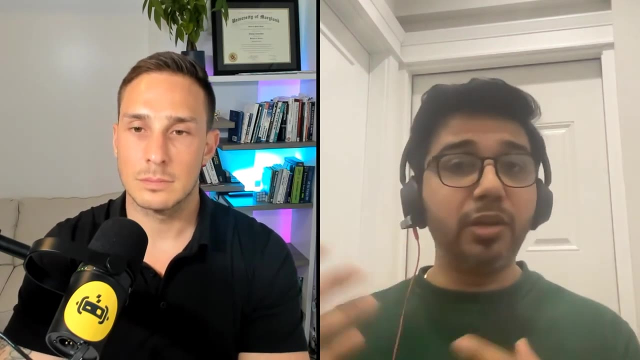 because I was working with some salesforce testing and I have a very good knowledge in salesforce, but, due to my task, I was never able to understand that. I was not able to understand that, I was not able to understand automation. so what should I do? so he took my session. we have a very one-to-one. 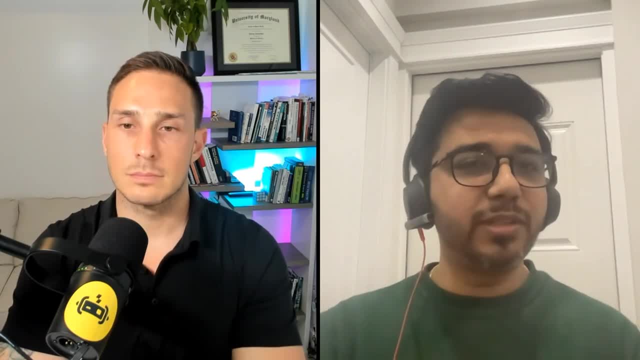 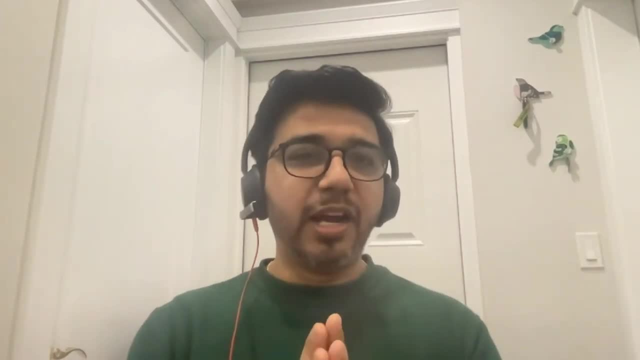 connection every week and I just keep on explaining the concepts and he got a job today morning. he has 13 days left. he didn't try to learn everything. I just ask him that focus on the concept. so only with concepts. he was able to crack interview only with concepts. honestly, I 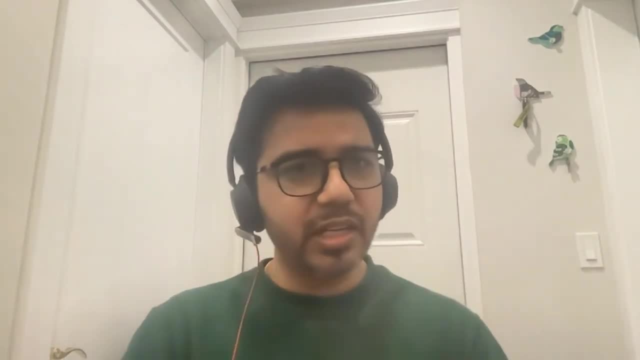 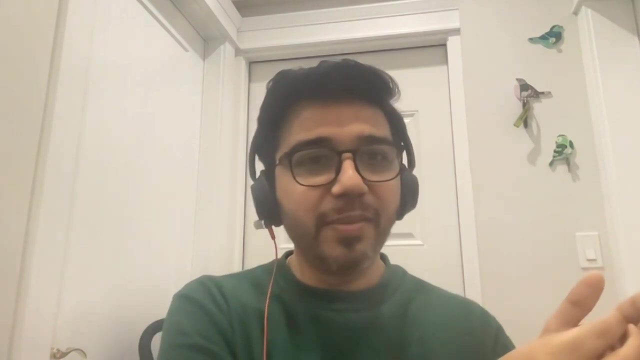 told him the same thing. tell honestly that you are working in salesforce setting. you didn't get the chance of automation, but you know concepts, how java works, how really over adding, overloading works. so he was explained the concept and the folks are very much impressed. they told: okay, this guy really understand what to do, so if we put him in a situation he will take. 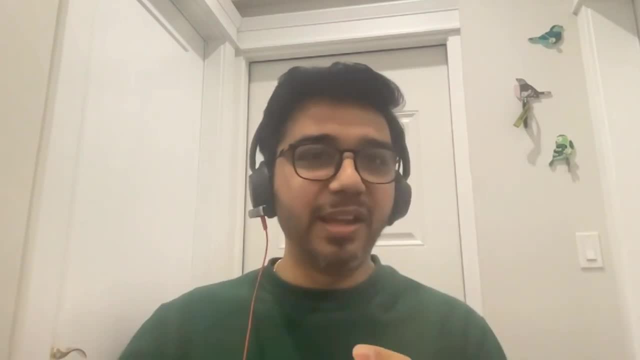 the right decision because he knows things. it's not like he has memorized things or he understand the concept. so excelling means you are properly understanding what you are doing, so if somebody asks why you have written this code, you should able to explain. that's awesome, said thanks for. 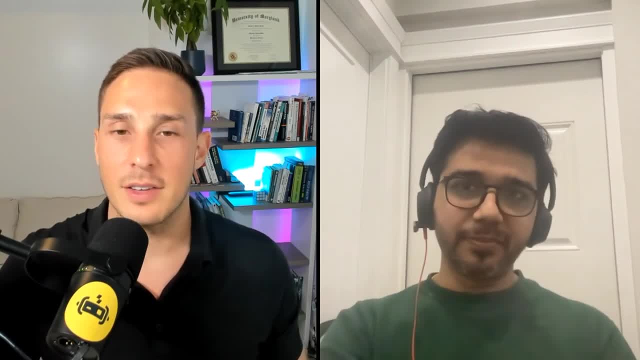 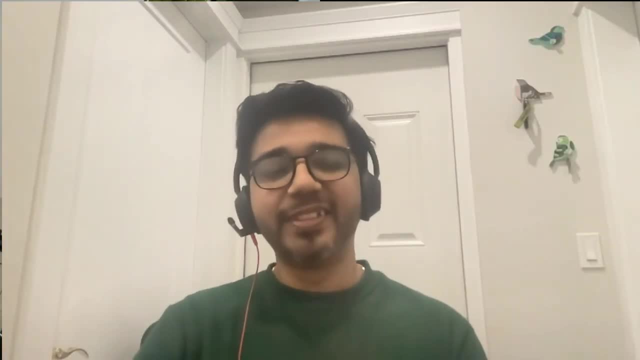 all of that, any last words of advice you want to leave us with before we wrap up the session, wrap up our interview? I would suggest that don't scared of generatively, okay, use it. so when automation started also, we never scared of it. right, we learned it and we do it. so learn generatively. 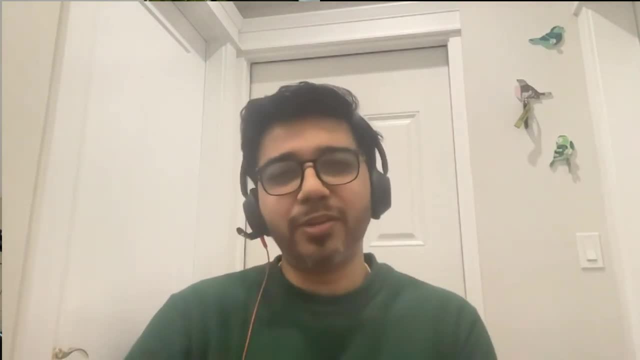 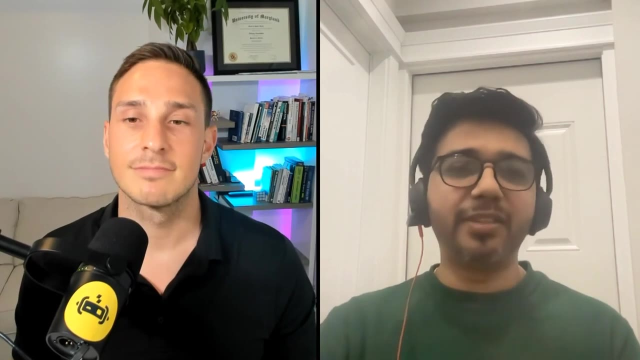 use it in your automation, take benefit out of it. right. it will not going to replace that. people are too much scared. we have designed generatively so how it will replace us. right. it will never replace us. rather, think about that. the boilerplate code we write, the repetitive task we do. we have 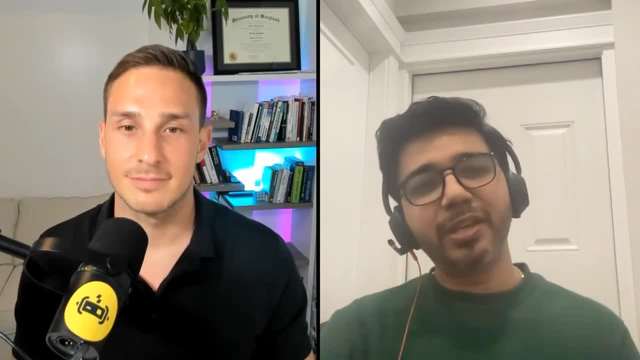 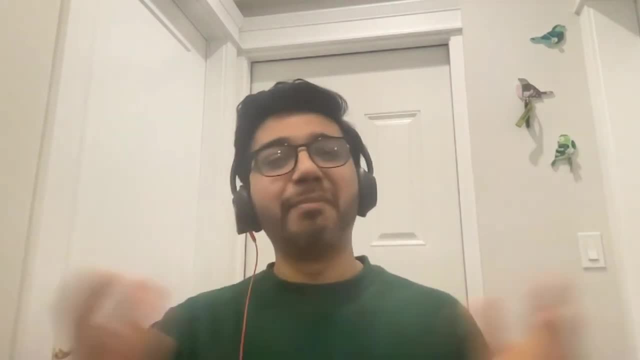 human intelligence, right, so let's use it in a constructive way. why, to do it in a constructive way? let's do the repetitive task and waste our time. let AI do that right. use your brain to do something more constructive right, for example, helping folks or community right, like Nicolay is doing. 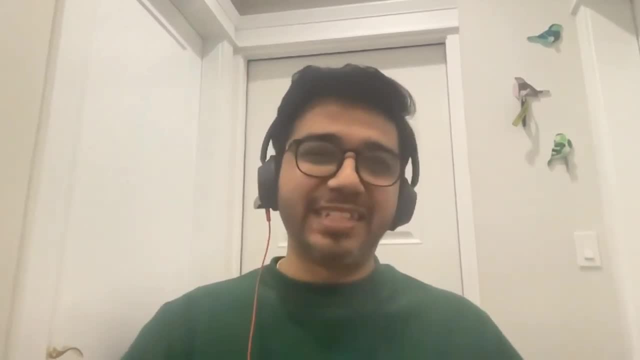 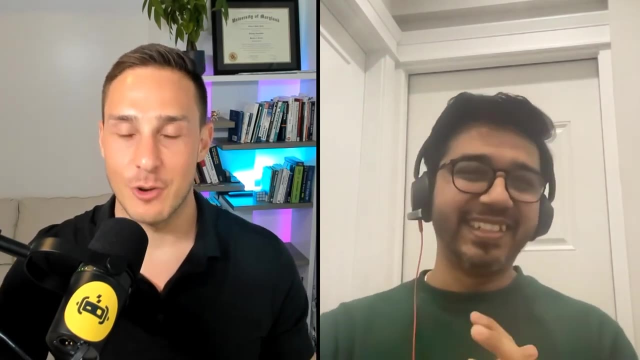 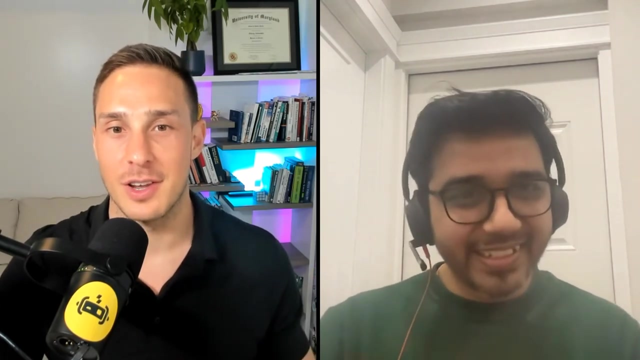 YouTube podcast right. help folks correct why to waste time in writing JSON reader. yeah, you can do that right. that's an amazing point, Sid, and thank you so much. and you're actually right. I actually use AI to help me prepare for the shows, so I have it prepare me the questions.